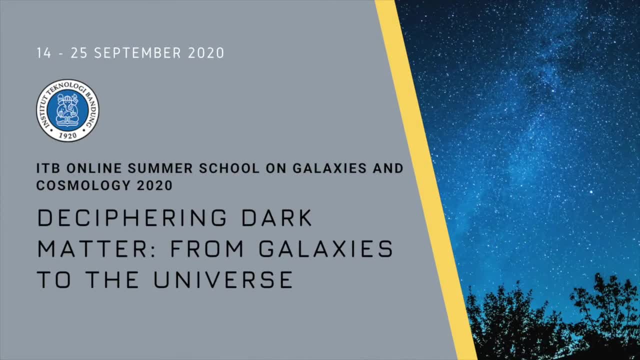 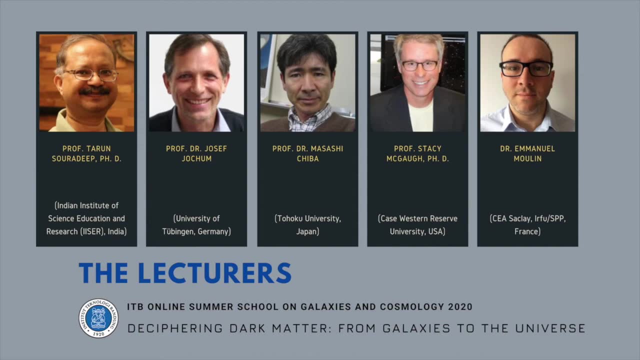 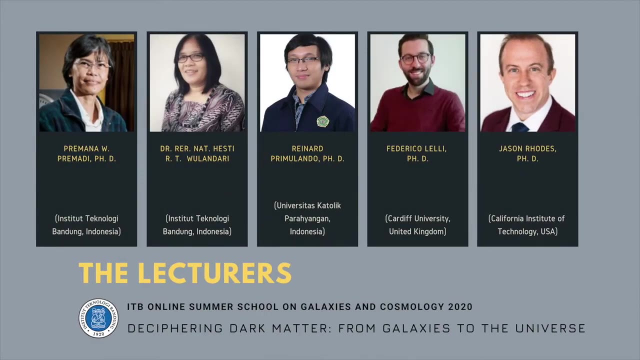 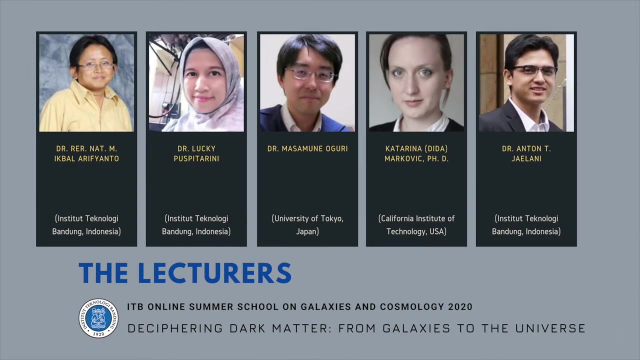 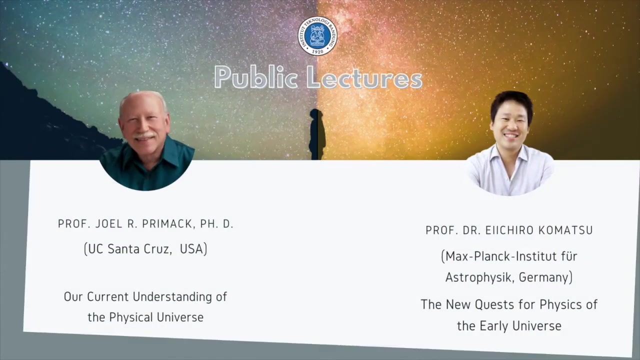 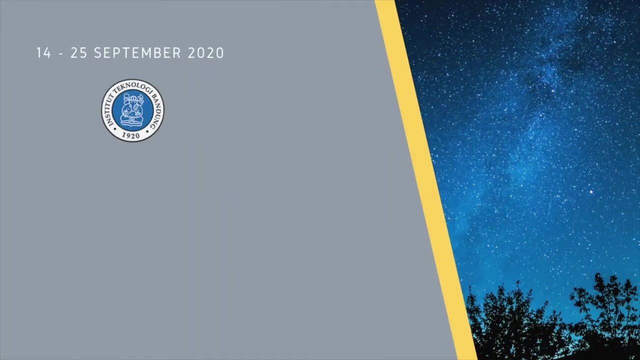 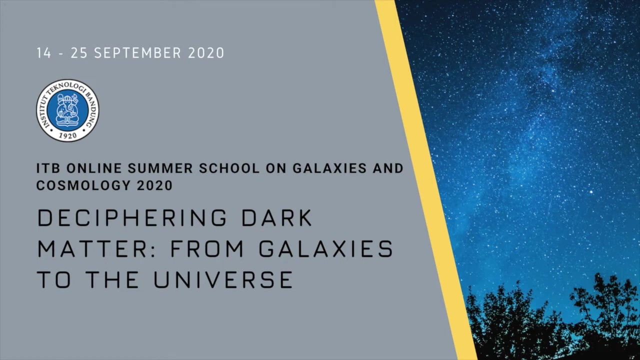 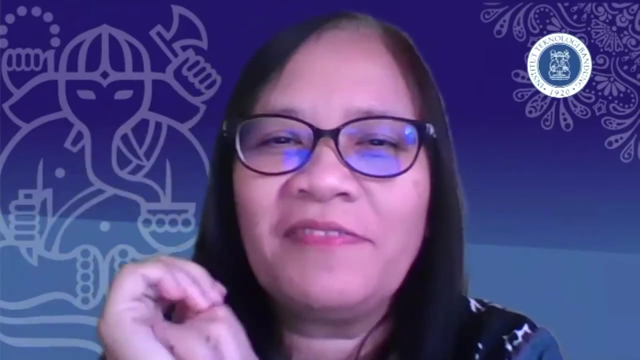 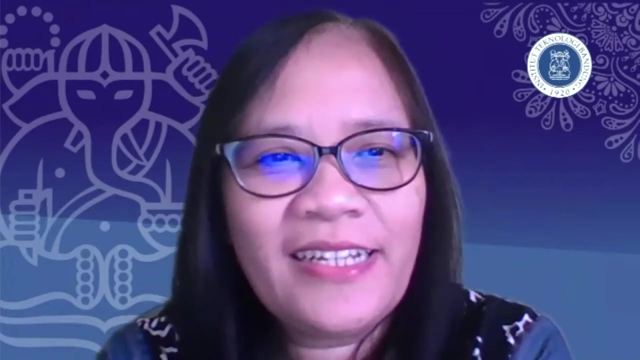 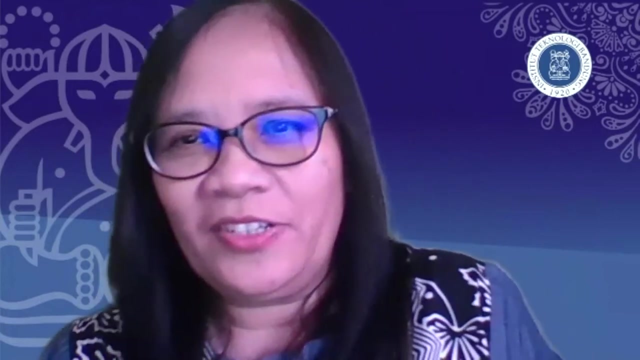 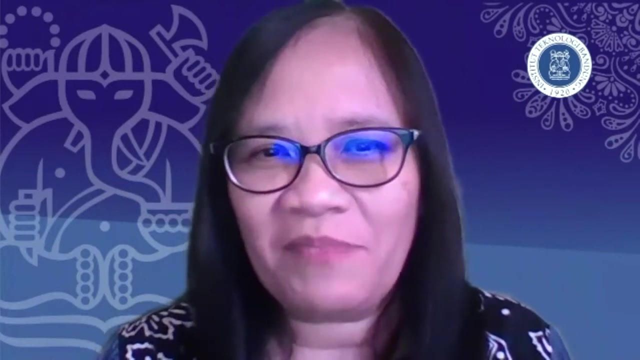 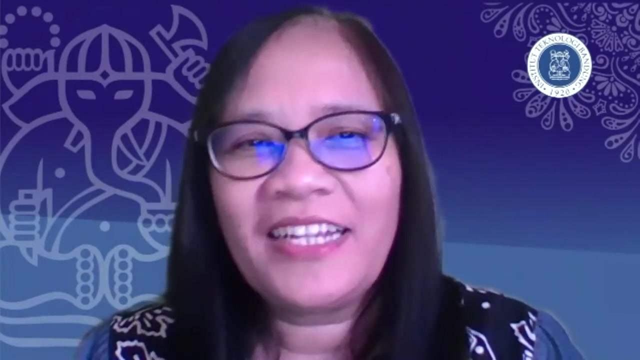 Thank you for watching. Thank you for watching. Now it's time for direct detection. I'm delighted to introduce our lecturer today, which is actually a special person for me because he was my former co-supervisor at the Technical University of Munich decades back. 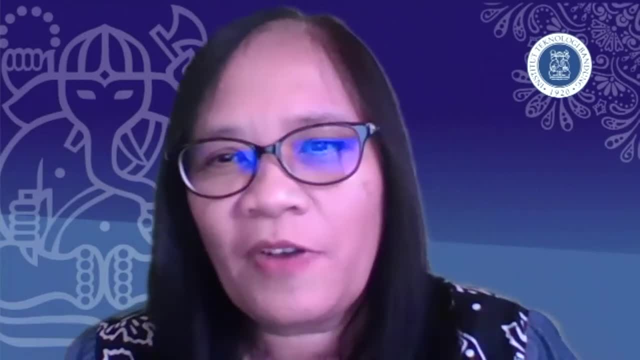 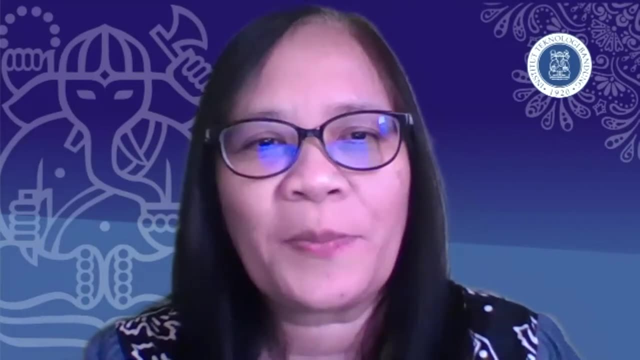 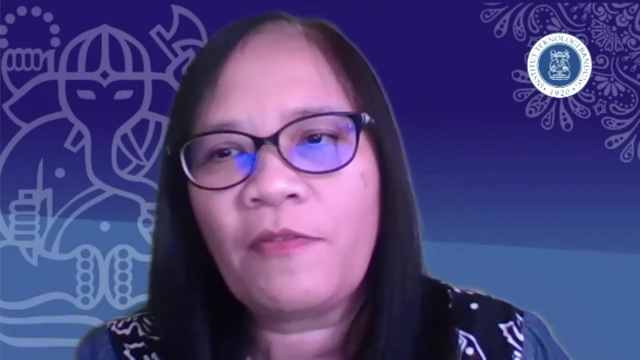 He is Professor Dr Joseph Jochum from the Kepler Center for Astro and Particle Physics of the University of Tübingen in Germany. Professor Jochum received his doctorate in physics from the Technical University of Munich in Germany. His fields of interest are in particle. 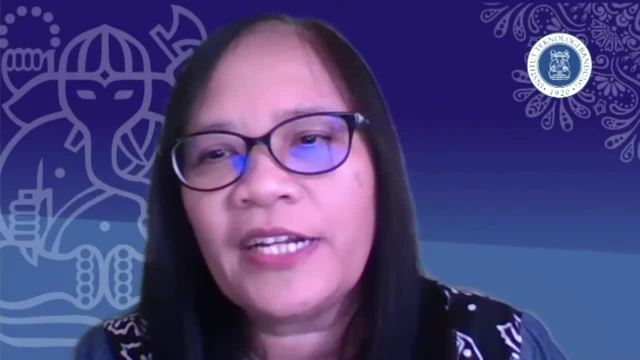 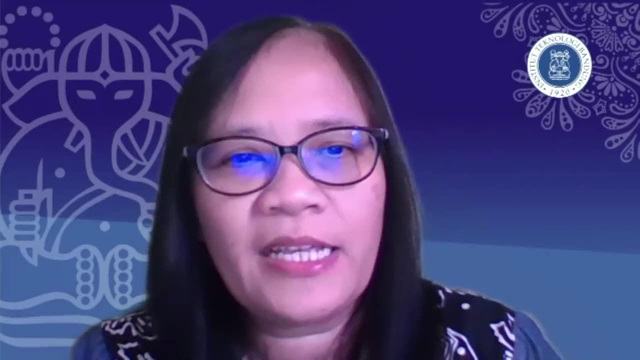 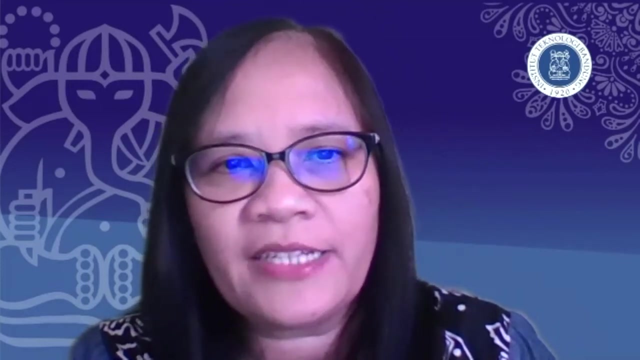 as well as astroparticle physics, including dark matter and neutrinos, and also detector development for astroparticle experiments. He has been involved in direct detection experiments at the University of Tübingen, namely CREST for wind detection, and also in METMEX. 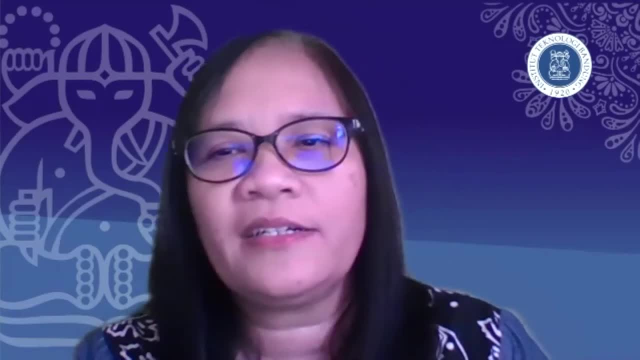 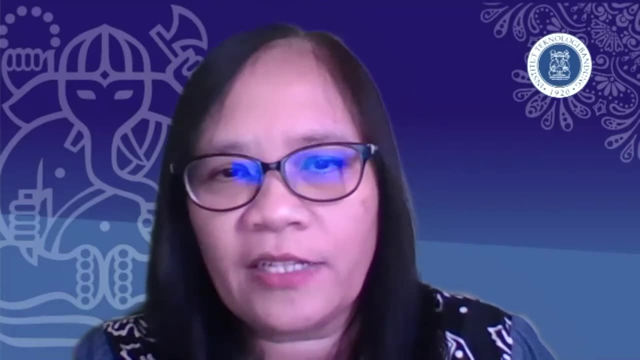 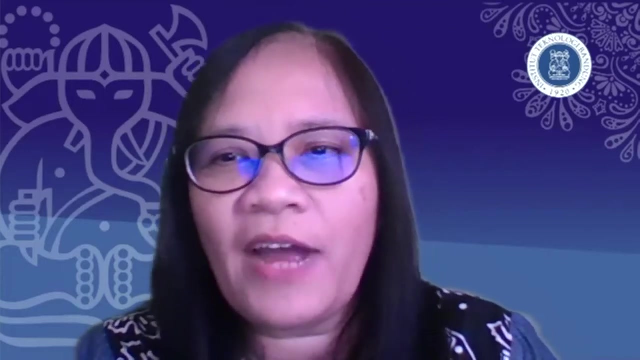 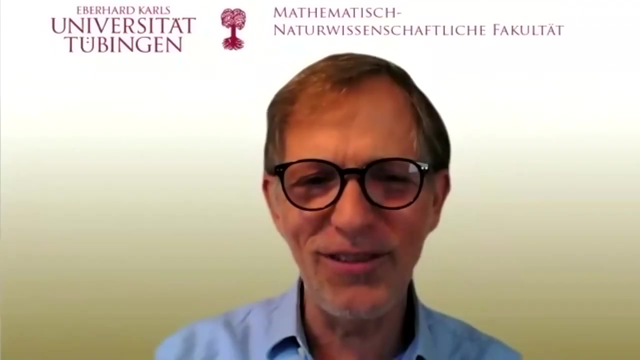 an axion dark matter detector. He is also involved in neutrino-less double beta decay detectors such as GERDA and now LEGEN. Okay, now let's invite Professor Jochum to deliver the lecture. Yes, Yes, good afternoon. Actually it's good morning for me. 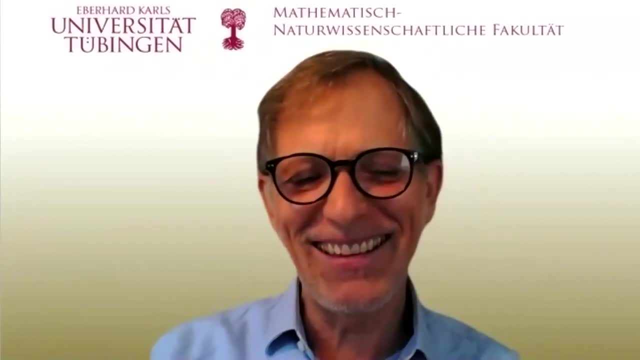 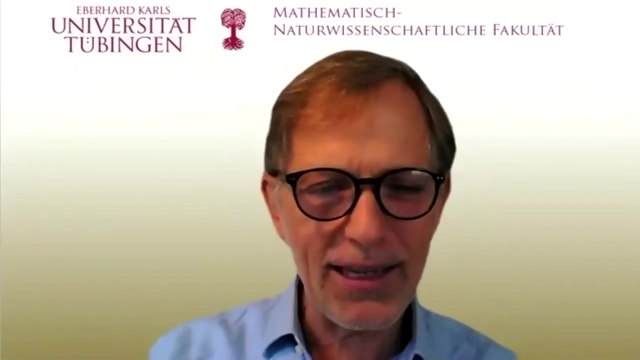 I am in Germany. It's nine o'clock in the morning. Thanks for having me in your summer school. It's an honor to represent direct detections in this school. Yes and well, I suggest we just right away start. I try to share the screen once again. 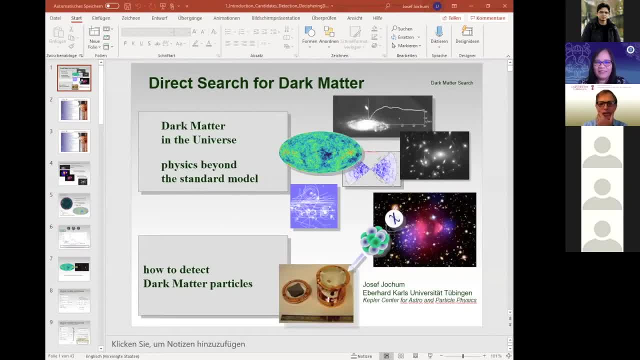 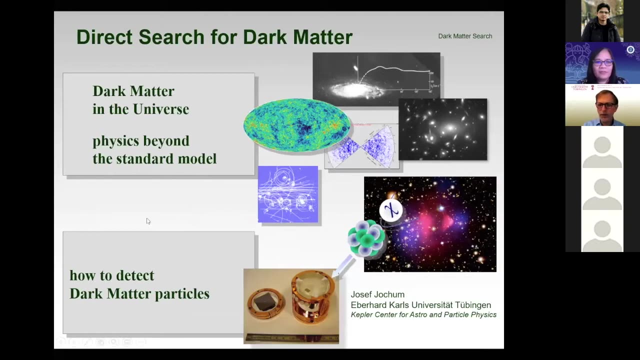 Let's see. So you should see the slides. now I go to presentation mode. Whoops, Just one, Okay, so I think you can see it. You can also see the pointer. Let's see. So this is my pointer. 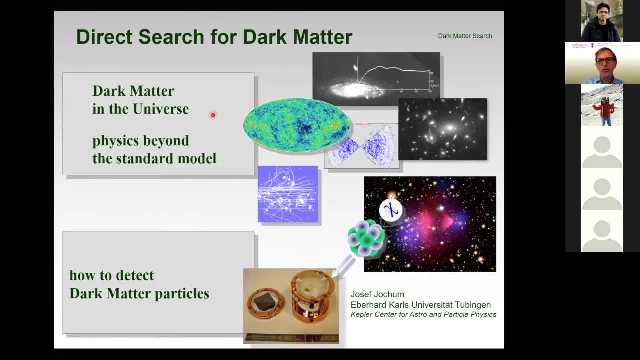 Okay, Okay. so the topic of my lecture today is direct search for dark matter. So of course, you know there is dark matter in the universe And for me, as coming from particle physics, the exciting thing of that- it's clearly pointing to physics beyond the standard model. 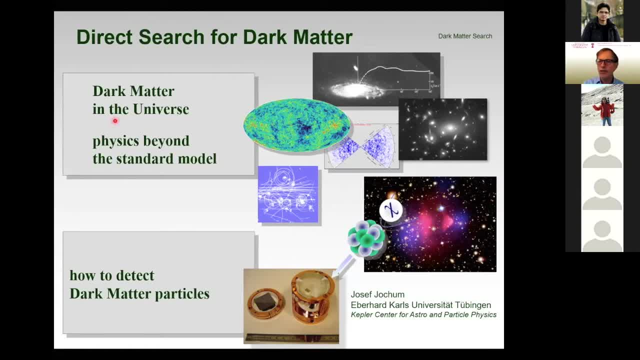 Actually, even after the era of LHC and all these accelerators, we have not found in the laboratory any proof of physics beyond the standard model, even if we believe it must be there. The only experimental or observational proof we have is actually dark matter. 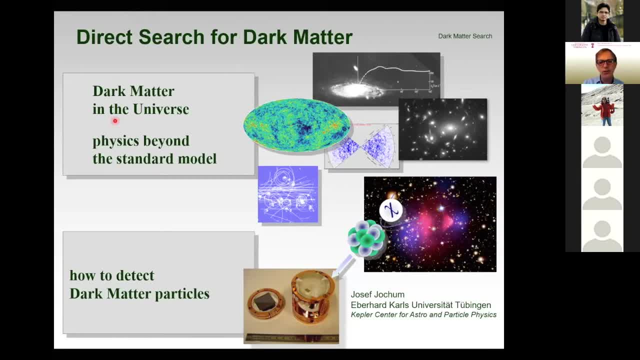 Maybe the masses of neutrino is also hinting towards physics beyond the standard model. but the only solid proof that there should be something more than what we know about particle physics right now is actually dark matter, And that's why I in the first part in my introduction 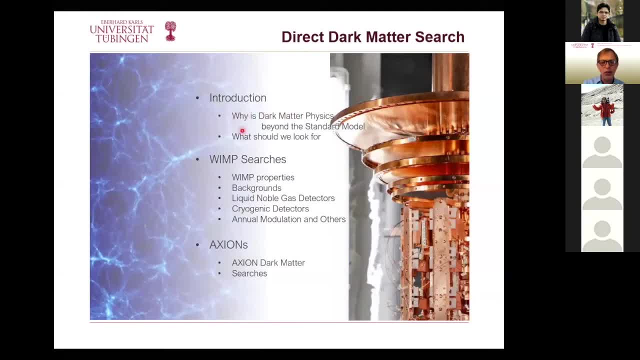 I would like to spend some time on the question: why is dark matter physics beyond the standard model, And that leads us to actually what we should look for, And then in the second or in the later parts, I actually go to the WIMP searches. 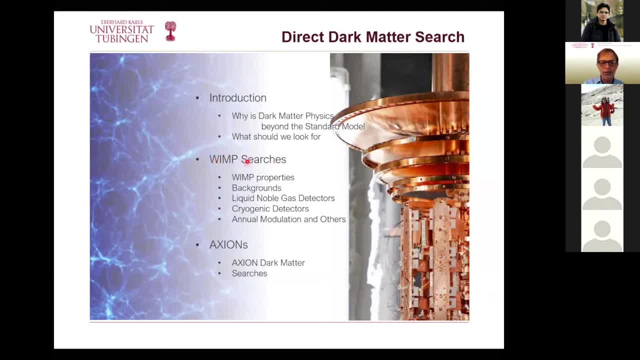 So the two, the two particles I will discuss are WIMPs and a little bit at the end, and axions as well. So, and I will show you the main challenges in the detector techniques And then, of course, something on axions. 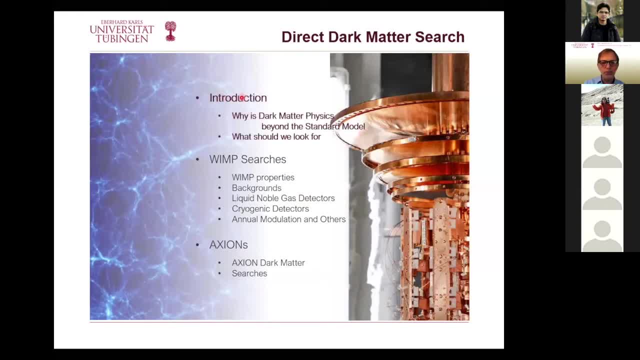 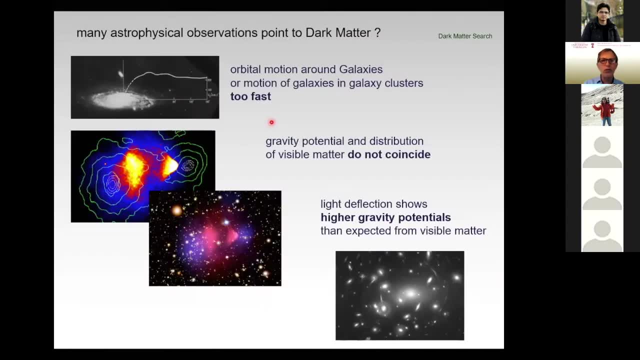 But let's start right away with the introduction. Why is dark matter physics beyond the standard model? OK, you all know the usual hints and observations and observational proofs of dark matter. It's the most classical one are the rotational curves around galaxies. So this is the orbital speed of objects orbiting around galaxies. 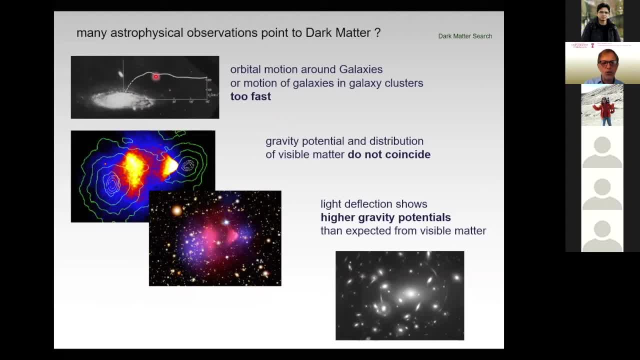 And this speed, according to the Keplerian law, should fall off, But it doesn't. And that shows you there is more centripetal force than what we see. So there must be mass around this galaxy, And since we don't see it, 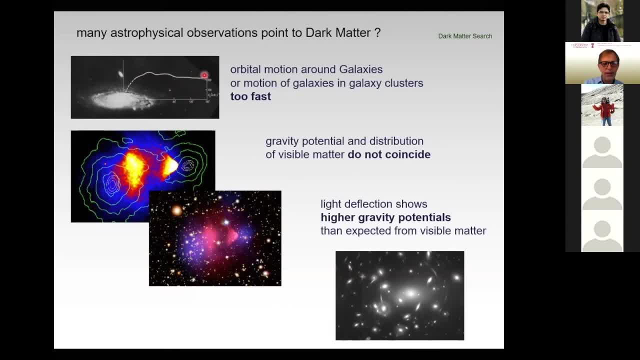 we call it dark matter. So this is the kinematical proof. Then there is a thing like the bullet cluster, which, in the bottom line, shows you that the gravitational potential can be where the visible matter is not. So the visible matter is here. 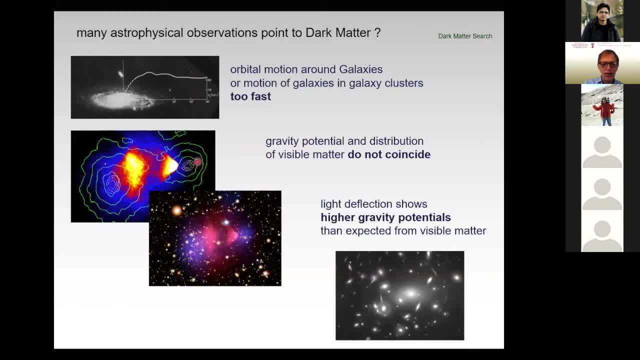 but the center of the gravity potential is somewhere else, And that is strange. This cannot be So. the center of gravity must be produced by something else which we do not see, And that's the dark matter. Another nice illustration are the gravitational lenses. 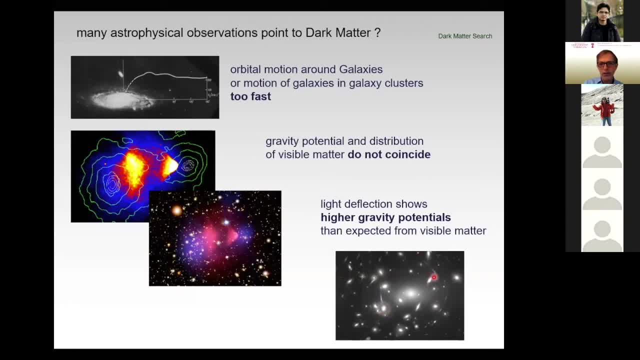 So here you see some examples. Here you see these arcs which are the light from more distant galaxies than the one you see in the foreground. But the light of these distant galaxies is spanned by the mass, by the gravity field of these galaxies. here 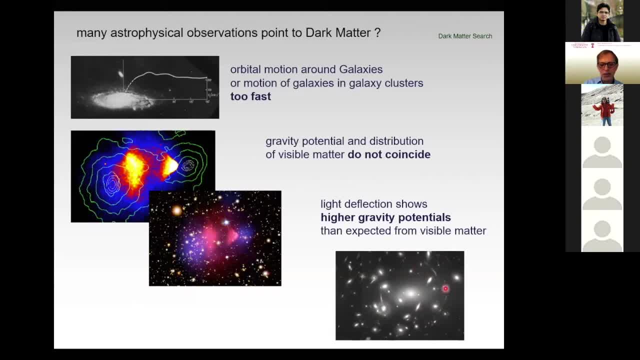 And there is a relation between the radius of these arcs and the mass of the lens of this galaxy cluster. And this also shows that there must be more mass to create these lenses here, these pictures here. There must be more mass than we see. 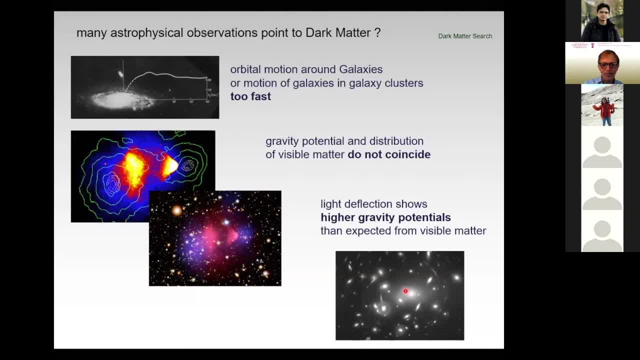 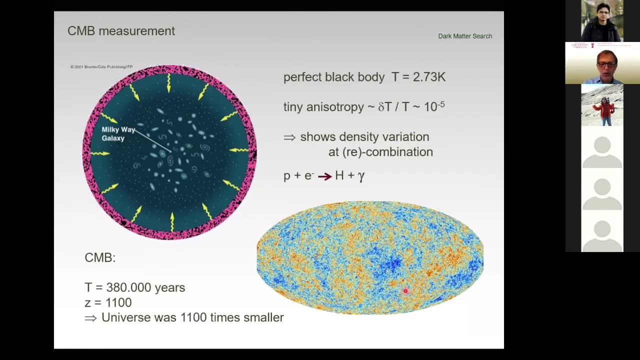 Okay, these are the standard, let's say kinematical proofs for dark matter, But the one I like most, and I think the most convincing actually, which brings it beyond the standard model, comes from cosmic microwave background. So the cosmic microwave background. 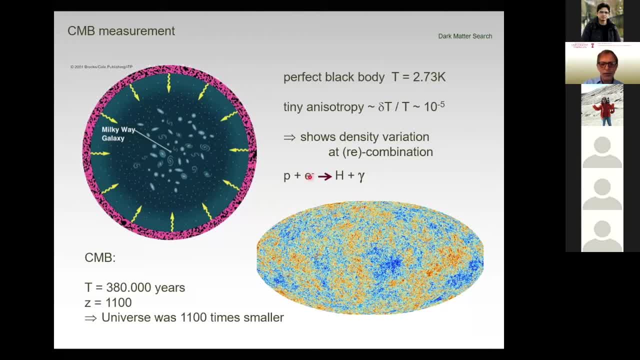 was created in the early universe. When the universe was hot, protons and electrons were still separated. But at the time of 380,000 years after the Big Bang they combined to hydrogen and produced photons, Before, of course, they could produce that as well. 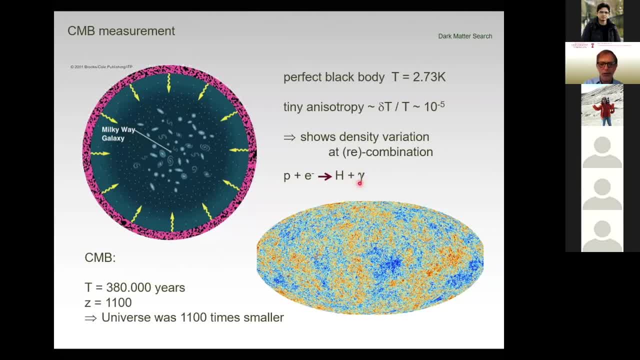 but the universe was hot enough so it had high enough energy photons to break the hydrogen again, And that was the time when it cooled down, so the hydrogen remained stable. We call that the recombination, but actually it was the first combination protons and electrons did. 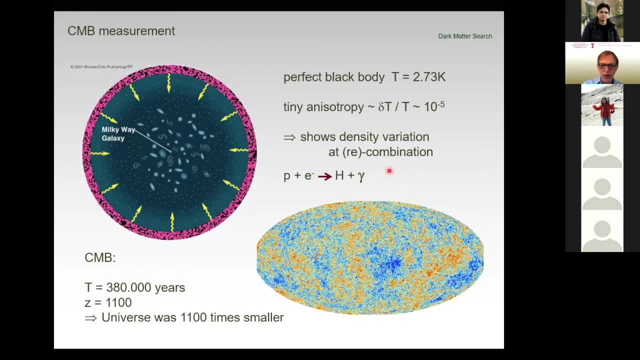 so it actually was the combination. Recombination only can occur later, But okay. so the thing is that before that happens, you have the universe full of charged particles and photons scatter on these particles, So the universe is intransparent. Photons cannot travel very far. 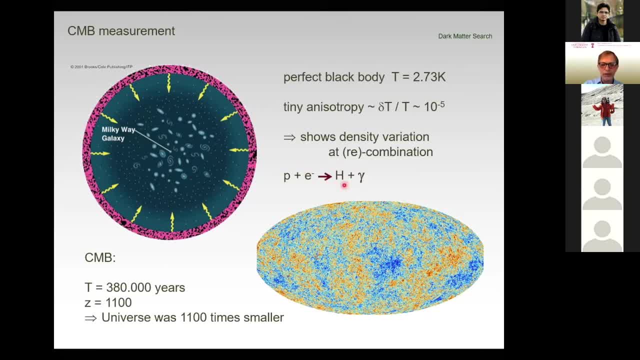 After that happened, you have only uncharged particles. the hydrogens and the photons have a very long mean-free path, so the universe is then transparent. So if we look, if we are here, and we look further and further away, 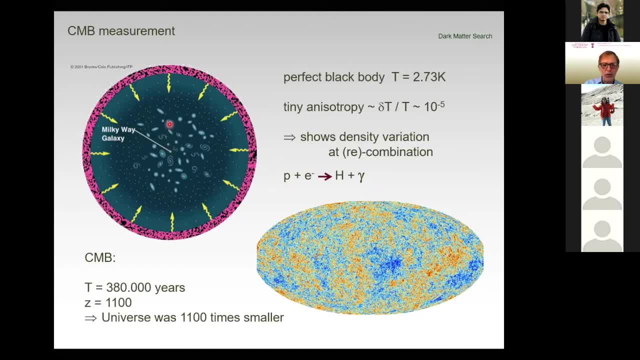 we also look earlier and earlier in the history of the universe. we see a transparent universe until we come to the time when this happened, And then we see a transition from a transparent universe to an intransparent universe And this surface of last scattering. 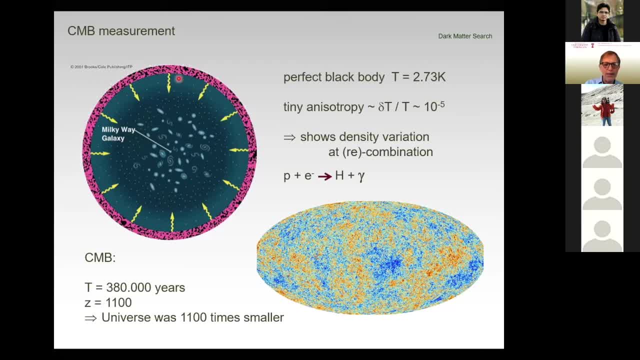 what we see. that's what we where. we see the anisotropy of the cosmic microwave background. So we can measure the microwaves coming from this surface of last scattering, which show a perfect black body at two or roughly three Kelvin. 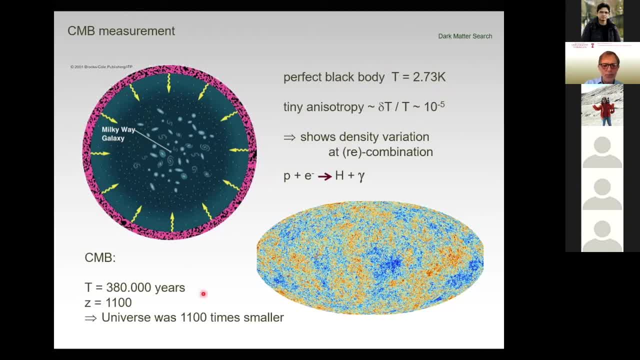 which shows us that the universe was a thousand times smaller at that time. So this happens at the redshift of 1100 roughly. So the scale, so the scale factor at that time was 1100 times smaller. But what we see on top of this black body radiation. 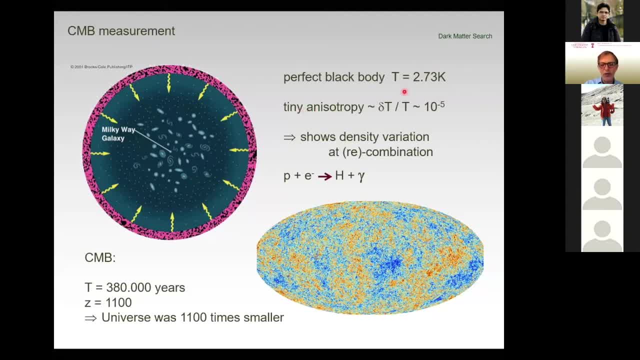 is anisotropy in this temperature on the level of 10 to the minus five or 10 to the minus six, And this is the interesting part. This shows us the structure of the universe at that time, And this is an illustration in galactic coordinates. 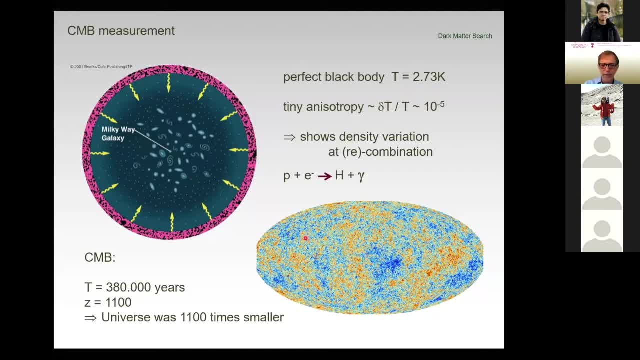 where you see these variations in this temperature And you can already see here a certain granularity which shows you the typical size of the structures at that time. And if you basically Fourier transform this pattern here, so in the simple view you would draw a line. 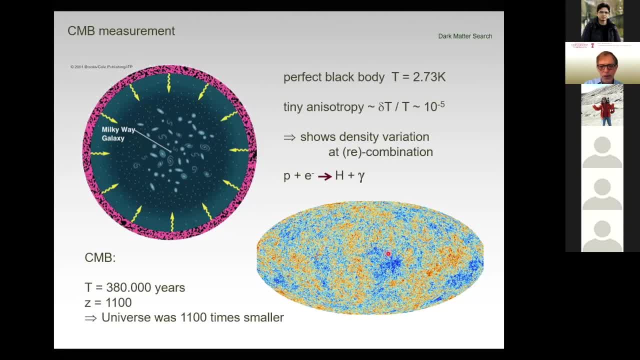 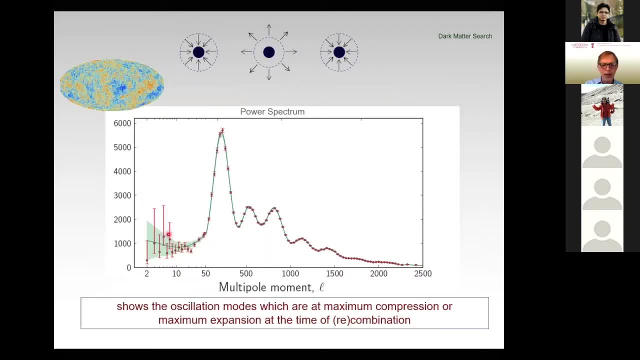 and along the line you have an up and down and an up and down of this density or this temperature, And if you do a Fourier transform of that, you get a spectrum like this, And this is a famous cosmic microwave multipole spectrum. 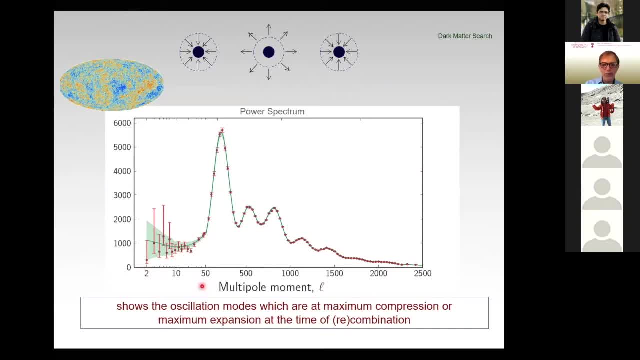 So here are multipoles. So this means the Fourier coefficient. So a high multipole means a high frequency. So these are small structures. here A small multipole, L means a large structure And this is basically the intensity of this structure. 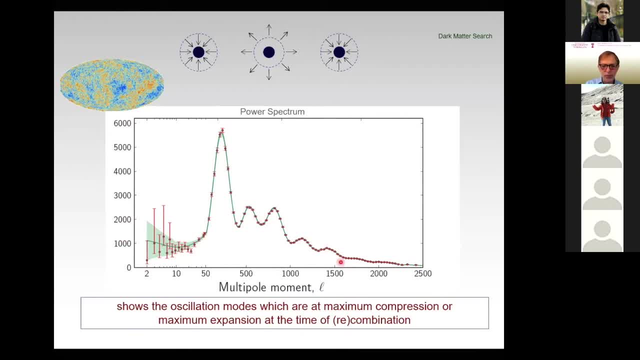 And you see peaks in this spectrum And these peaks represent the status of oscillations in this early plasma of protons, electrons and photons. And the first peak, basically, is a mode which had just enough time in this 380,000 years to go into maximum compression. 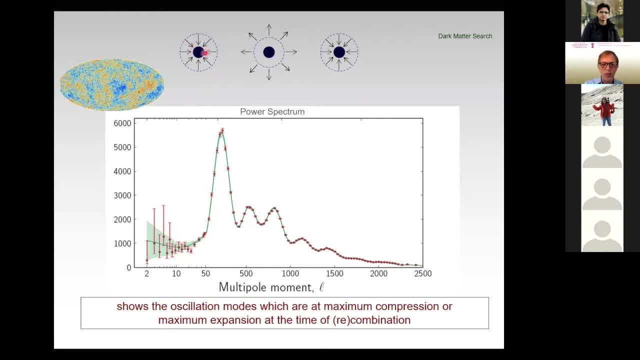 So it looks like this: It's a maximum compression. This is the first peak And it took 400,000 years to do this maximum compression. The second peak is at double the multipole. So this is half the size, double the frequency. 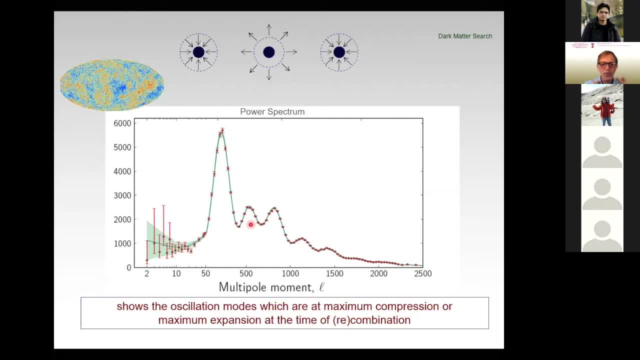 So this means this had enough time to go into maximum compression And back in maximum expansion again. The third peak: three times the multipole compression, expansion and compression again. So we have a compression, decompression, compression, decompression, compression. 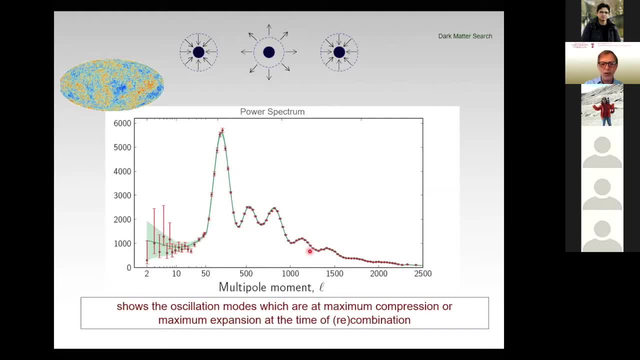 So alternating pattern of compression and decompression peaks in here And on the level of 10 to the minus 5.. And this is the structure basically when hydrogen formed, And we must understand how all the structures we see today have formed from that. 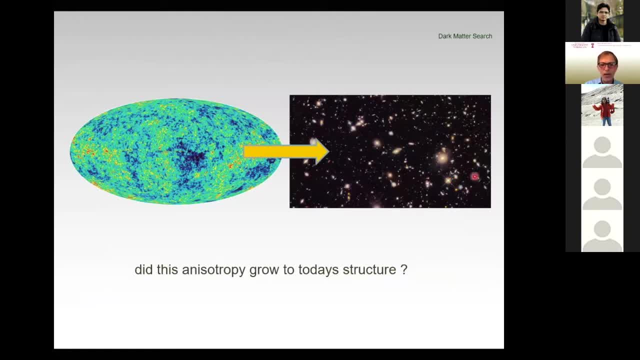 So this is the seed where we started. That's where we are today. And the question is: did this anisotropy grow to today's structure? And you probably know about structure formation. I will do a very short recap on that because to understand how this anisotropy 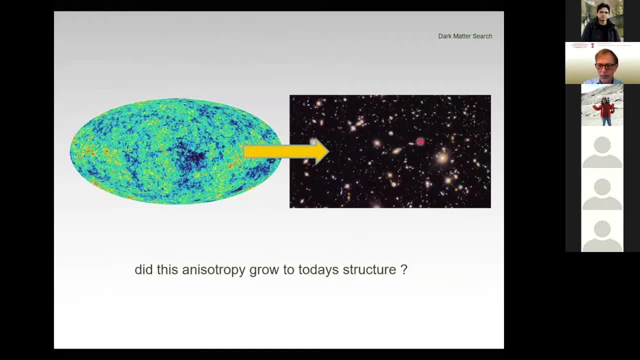 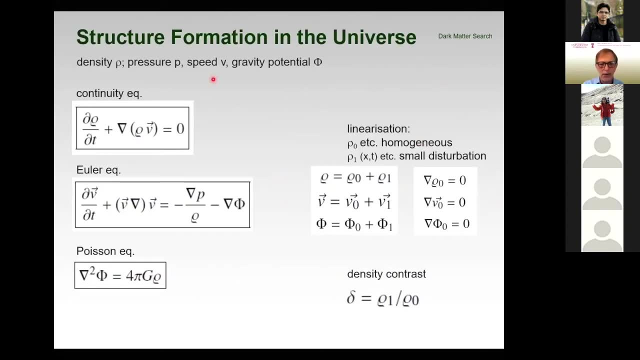 can grow to today's structures. one has to understand a little bit on structure formation And I do it very simple here. It's basically a classical mechanics, Newtonian picture of what I'm doing here. It's basically the same like deriving sound waves in air. 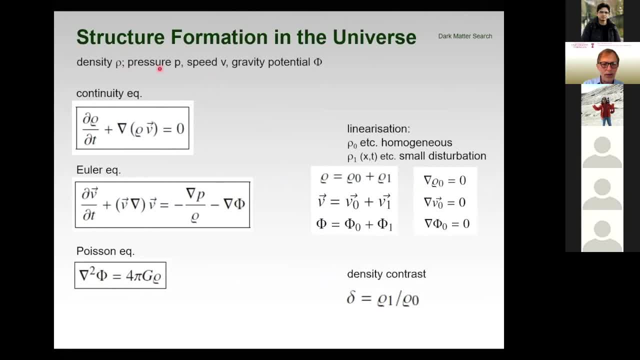 So we describe the universe by a density, by a pressure. The density elements have a speed and there is a gravity potential. So that's different. That's what you usually don't have in aerodynamics or hydrodynamics. So here we have oscillation. 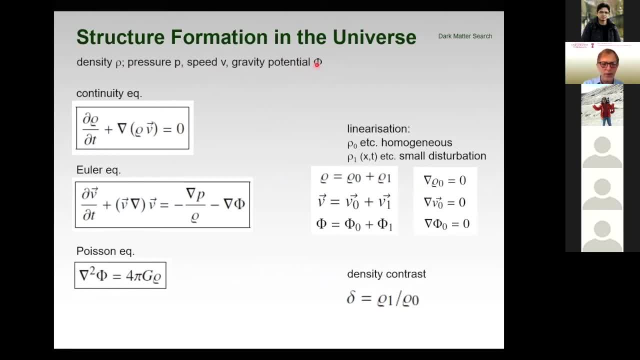 basically sound waves in the presence of a gravity potential. So you have a continuity equation which tells you that the temporal change in the volume element is given by the flux in and out of this volume element. We have the so-called Euler equation, which is nothing else than Newton's law. 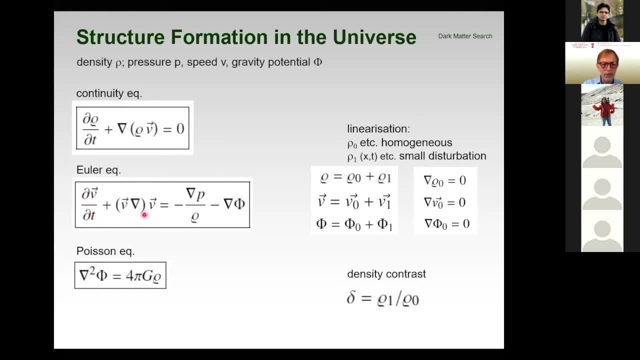 So here's acceleration. It's the derivative of the speed. That's acceleration. Sorry, is there a question? No, Okay, And here are the forces. So this is the pressure gradient and the gradient of the gravity potential. So that's gravitational force. 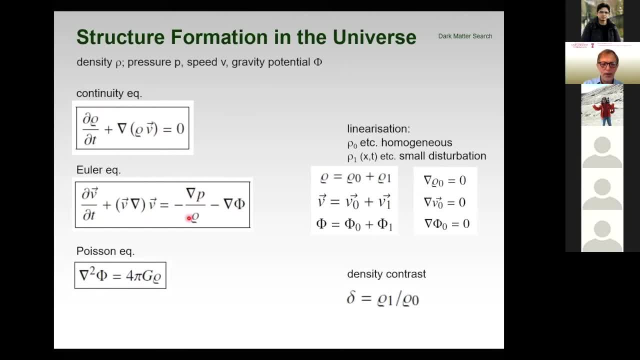 and this is the force given by the pressure. And then we have the Poisson equation, which gives basically the gravity potential independence of the density. So now what you do? you linearize these equations. You say: all these quantities have a solution with the index zero. 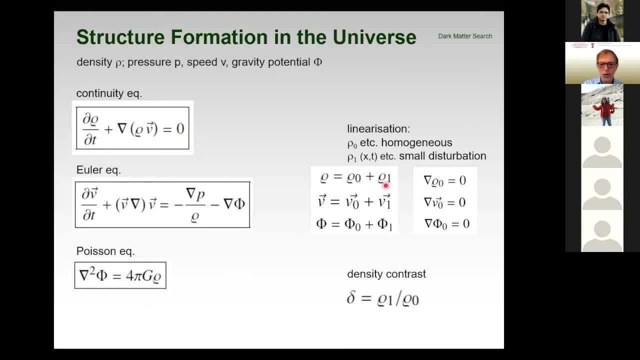 and then there's a small perturbation, So the row one is much smaller than the row zero, And it's true for all of them. and the zeros fulfill these equations. And then we define the so-called density contrast, which is given by the change of the density. 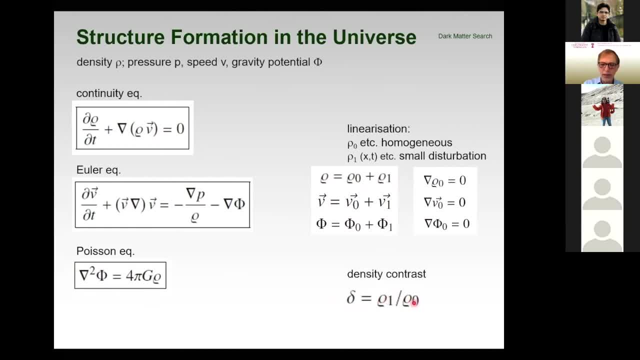 or the small variation given by the average density. So that's the quantity, the density contrast we would like to see to grow from this early 10 to the minus five to today. huge number, because today the density contrast is very big. Okay, If you do your math. 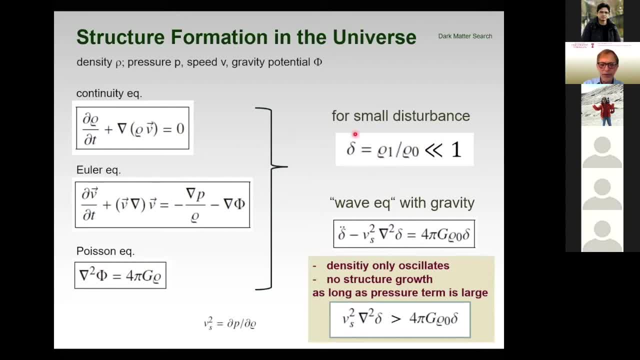 I don't do it here. If you plug it in and you say, okay, this delta is very small, you derive a wave equation for this delta, for this density contrast. It's a classical wave equation. So this is the second derivative in time. 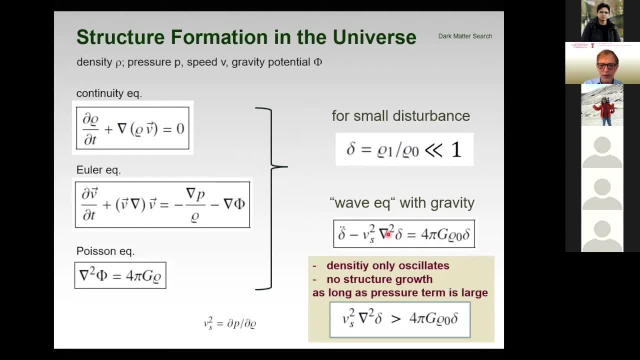 Here's the second derivative in position, Here's the sound speed, And usually you have a zero here. That's when you have sound waves, Then you have just the classical sound equation, wave equation. sorry, The only difference here is that we have this term here. 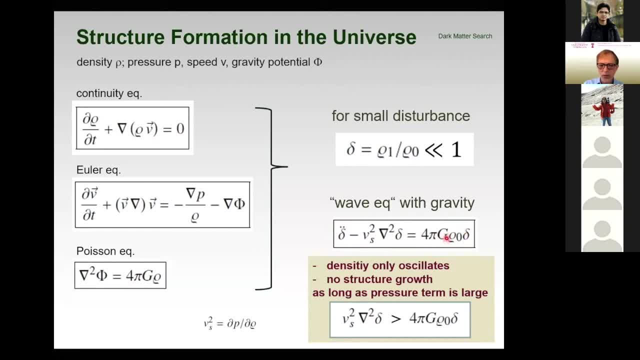 on the right side, which is given by gravity because, different to sound waves, when we have a compression we not only have the pressure to dilute this compression again, we also have gravitational force which would like to let grow this compression. We all know when there is much mass somewhere, 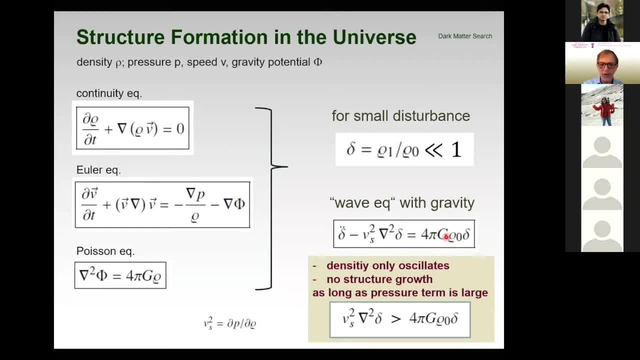 gravity would like to intensify that. So we have two competing forces here. This is the gravity on this side which would like to grow densities, And we have this term here which is basically coming from the pressure, This term here which would like to decrease compressions. 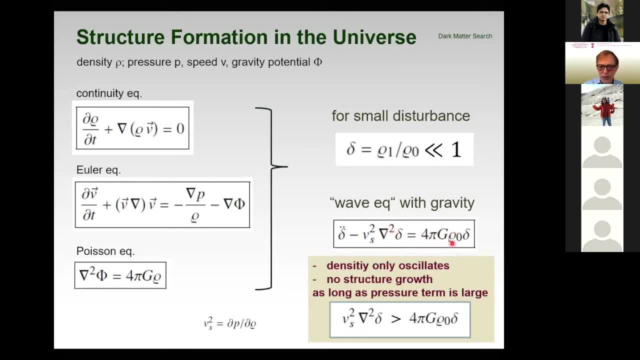 So usually, if there is a zero, here, you only have oscillations, sound waves. And actually when this term here, this pressure term, is bigger than this, here we are in this situation, Then densities only oscillate, We only have sound waves. 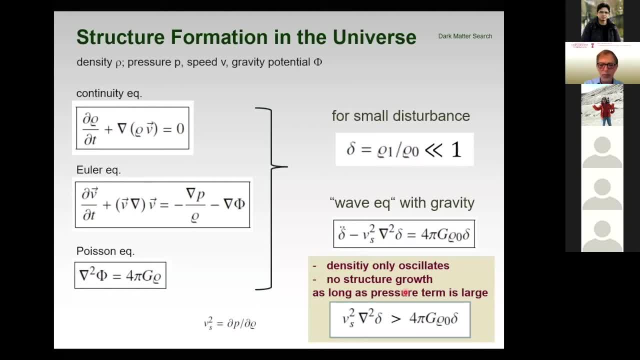 That's what we see in this pattern of the cosmic microwave background And we have no structure growth. Anything which will grow oscillates back and forth, and back and forth. And that's the case as long as if this term, this pressure term, 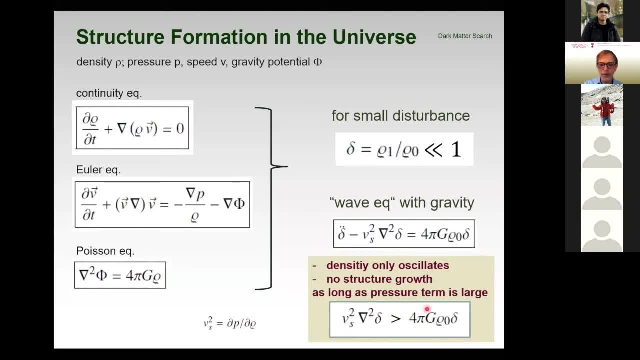 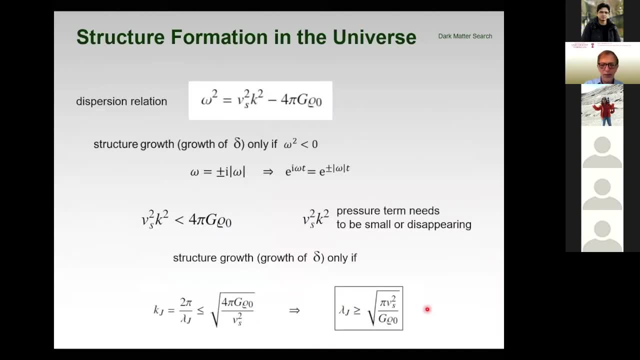 is larger than this term, the gravity term, To make that a little bit more clear. okay, it's just when you, when you go in with into this wave equation, if you go in with plain waves, you find this dispersion relation. 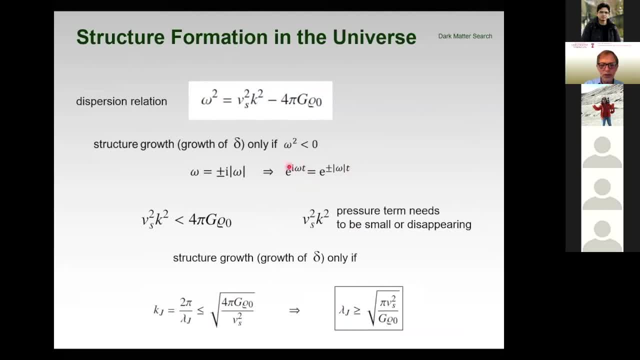 And you see the temporal check behavior which gives you if there are oscillations or not. this omega is positive or negative, or it's imaginary or real, depending if this term is larger than this term or not. This leads you to a maximum k. 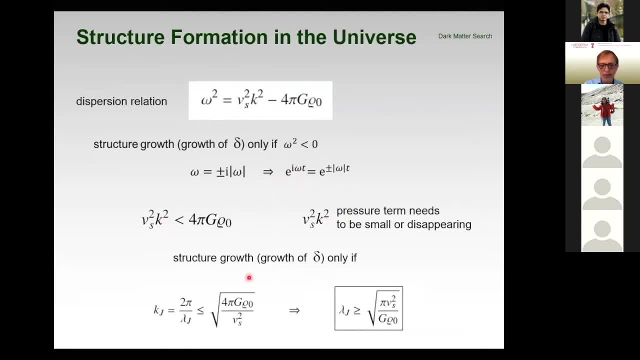 or a minimum lambda, which you might know as the gene's length. So this argument leads you to the gene's length or the gene's mass. You need a certain minimum mass or object mass to have a certain minimum size to collapse, Otherwise, 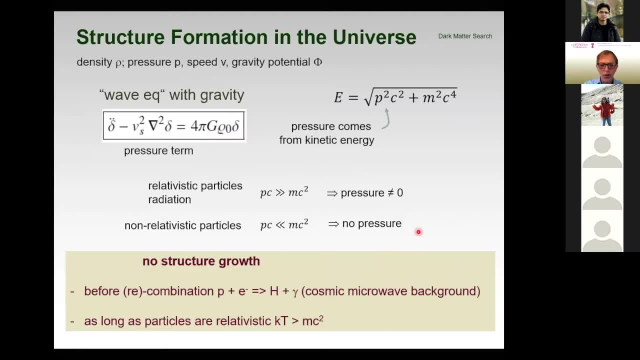 we will not. have. no, have not structured row, Okay, but again. so we have this wave equation and it only oscillates if this term is larger than this term. And this term comes if you look at the particle picture, if you say: 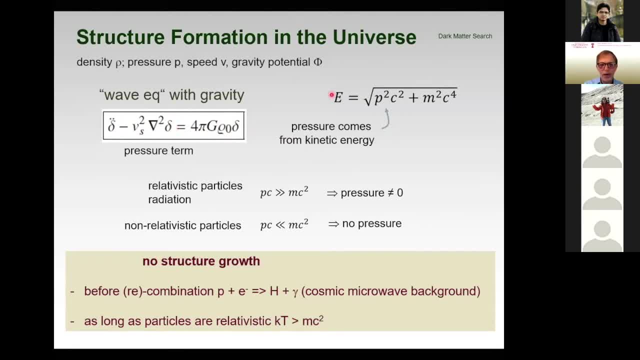 okay, your universe is set up with some particles. these particles have energies, they might, they have kinetic energy and they have rest mass energy, And this term is large when this term, this kinetic energy, dominates. So for relativistic particles we have pressure. 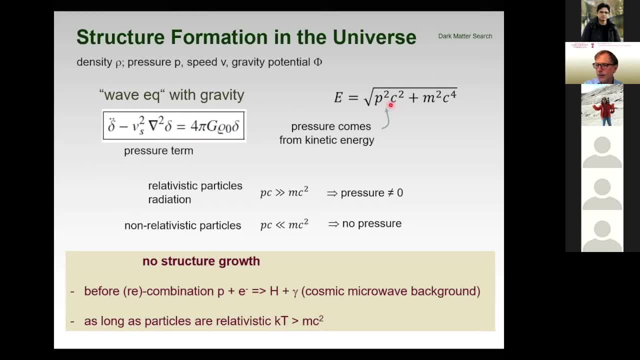 Cosmologists say to relativistic particles: radiation. Everything which is relativistic, it's summarized as radiation, And radiation means this term dominates. So then the pressure term is much larger than the, or the kinetic term is much larger than the rest mass term. 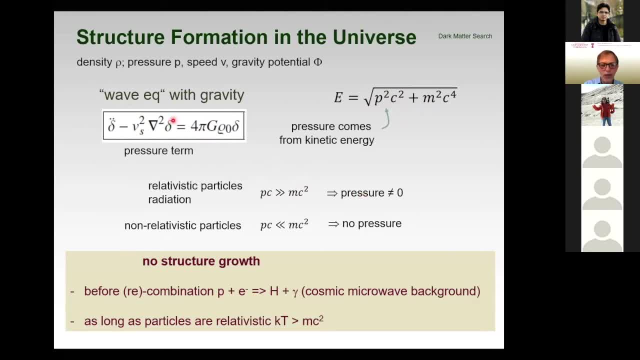 The pressure is unequaled zero and we only have oscillations. If you have non-relativistic particles, when this kinetic energy is much smaller, we have no pressure and then we can have structure growth. So structure growth in the universe is only possible. 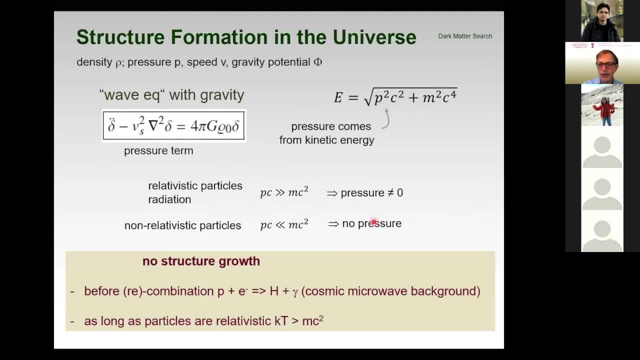 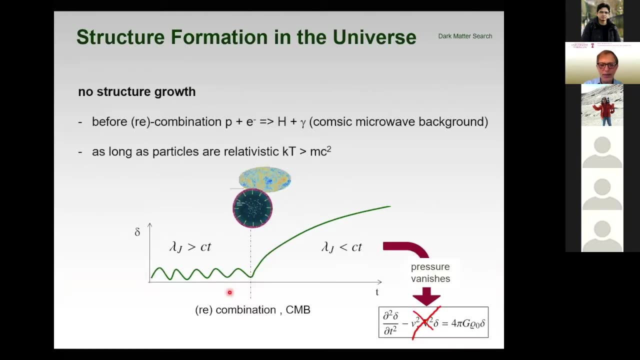 if you have non-relativistic particles and if your particles are not bound to radiation And before a combination. the particles have a high pressure because they are coupled to the radiation, because of their charge, And that means in the baryons we see in the 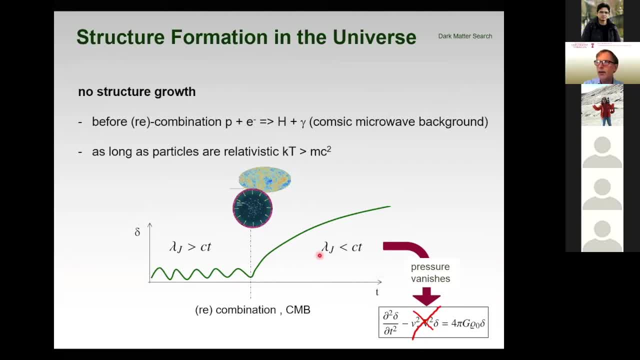 or this matter. we see in the cosmic microwave background are protons and electrons, Everything with a charge, everything with electric charge we would see in the cosmic microwave background. So that's basically all our standard model particles, except neutrinos, are participating in this cosmic microwave background oscillations. 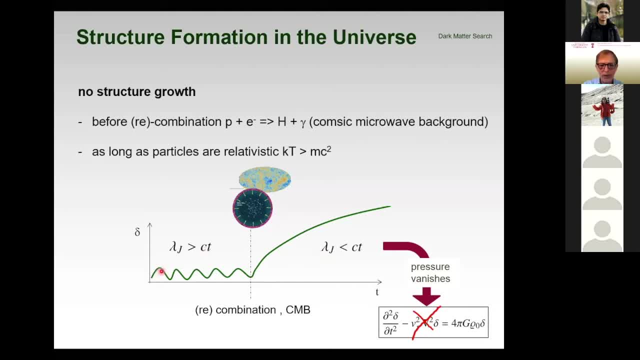 And this can, since they are coupled to radiation. they only oscillate, They oscillate, they oscillate, they oscillate, until the recombination. Then we suddenly have hydrogen non-relativistic, and only then the structure can start to form. 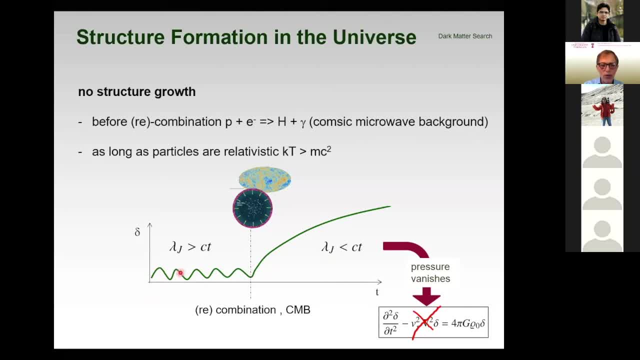 So this is the density contrast Before recombination it only can oscillate, and then it can start to grow. Then this pressure term vanishes and we have an equation like that. So this is a problem. So this means we have to understand. 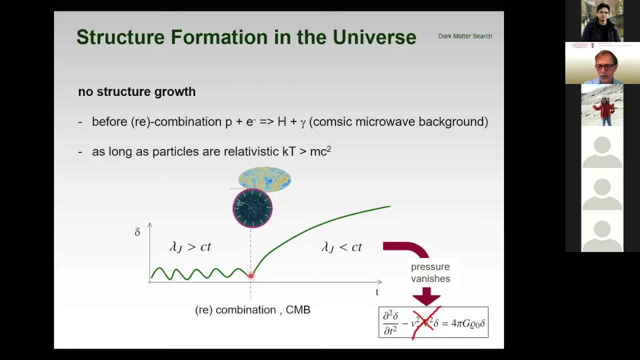 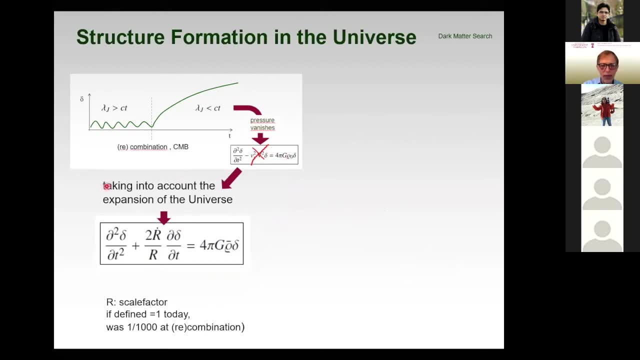 our structure, starting at recombination, And then, if you say okay, at this point, the pressure term vanishes, Okay, but we had a simple picture. We did not take into account the expansion of the universe. If you do that, 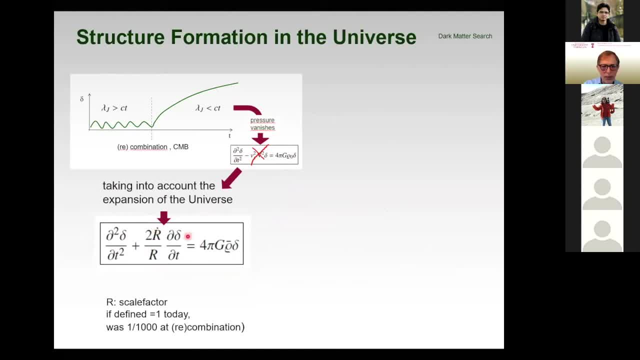 this equation changes a little bit. You get an additional term And then you can solve this equation for the time after recombination and ask the question: how is delta growing now? How does it behave as a function of time? So you plug in r. 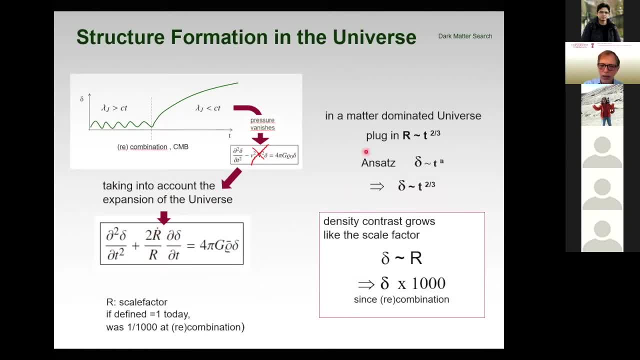 which is the scale factor of the universe. in a meta-dominated universe which we have after this recombination it grows like t to the power of two-third. And then you can solve delta, how delta grows with time And you find it also grows like two-third. 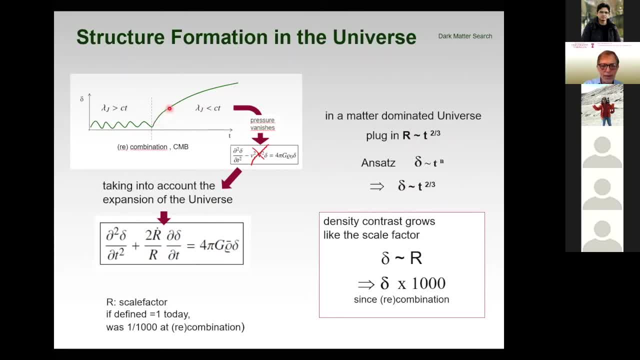 So this means when the density contrast starts to grow, it grows proportional to r. This tells us that since the recombination, r has grown by a factor of 1,000 or 1,100.. So this means delta grows from recombination to today. 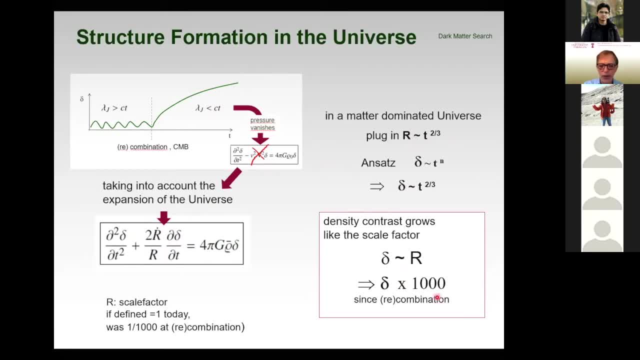 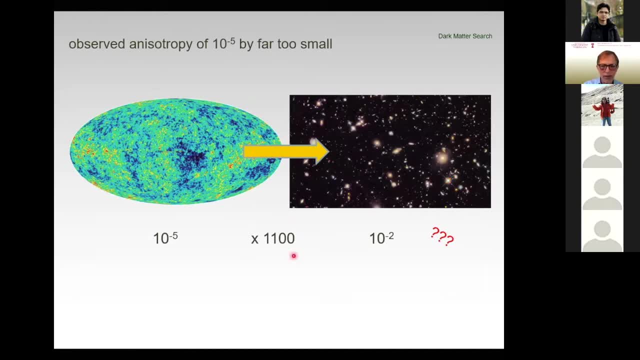 by a factor of 1,000.. Okay, if you take 10 to the minus five, which we see here, times 1,100, you end up at 10 to the minus two, 10 to the minus two. variation in density. 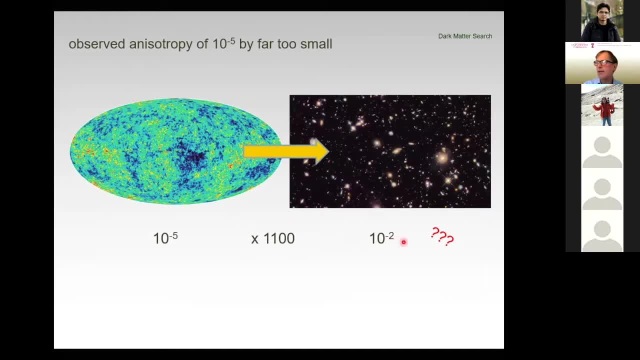 This is a 1% variation on a homogenous otherwise homogenous or a homogenous variable Otherwise homogenous universe. That's not what we see today. We see today a huge number. This number must be 10 to the four. 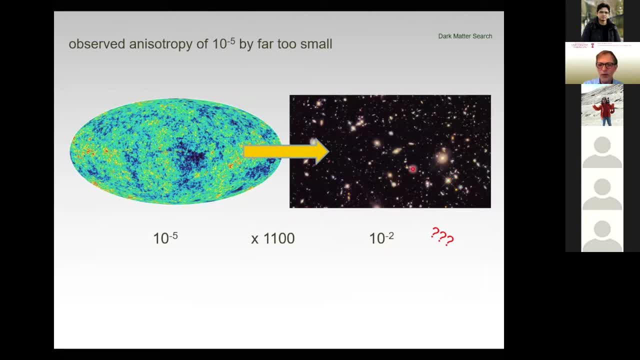 10 to the five, not 10 to the minus two. So from the baryons we see here, we cannot understand how this structure of today can have grown. It's impossible to grow that in that time. So the only way out is: 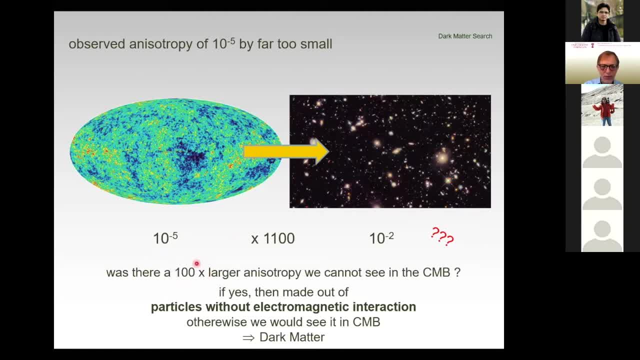 that there must have been at least 100 times a larger anisotropy, which we cannot see in the CMB. If there was such a large anisotropy, if there was already at recombination, then it must be made out of particles. 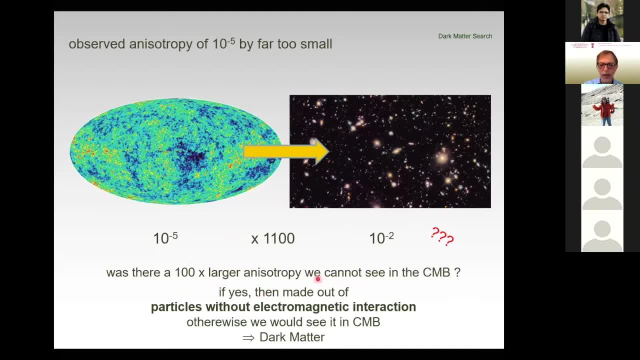 without electromagnetic interaction. Otherwise we could see it in the cosmic microwave background. So the only way out here is that we have a dark matter, meaning a matter without electromagnetic interaction, which started structure formation much earlier. So the picture then is we have this dark matter starting structure formation. 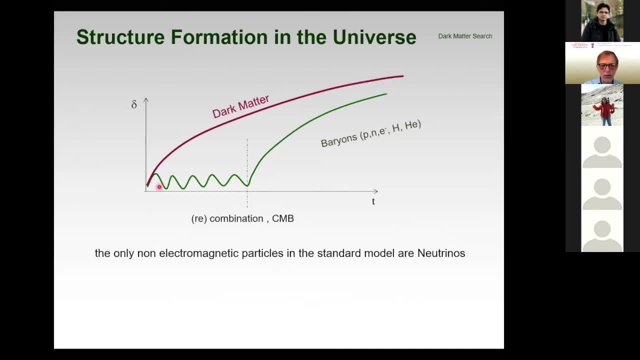 because it had no pressure. Then the electromagnetic interacting matter. cosmologists call that baryonic matter. So the baryonic matter oscillates, oscillates, oscillates, oscillates After recombination. also this baryonic matter can form structures. 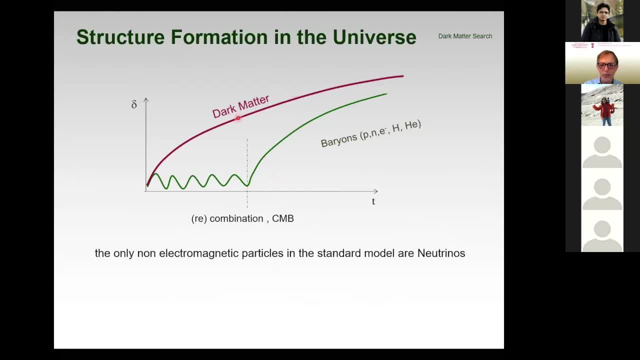 but it falls into the structures the dark matter has already prepared, And the only electromagnetic particles in the standard model are neutrinos. But neutrinos are still relativistic at the time of recombination. Their pressure term is still too big at that time. 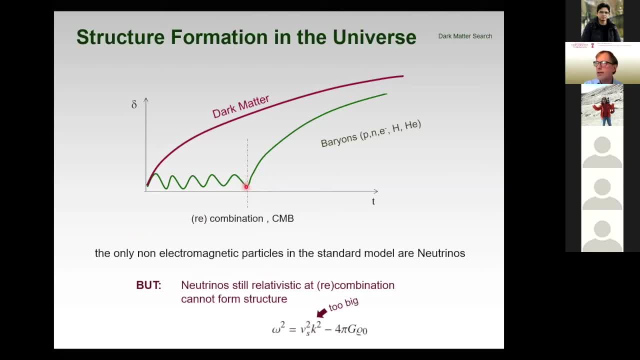 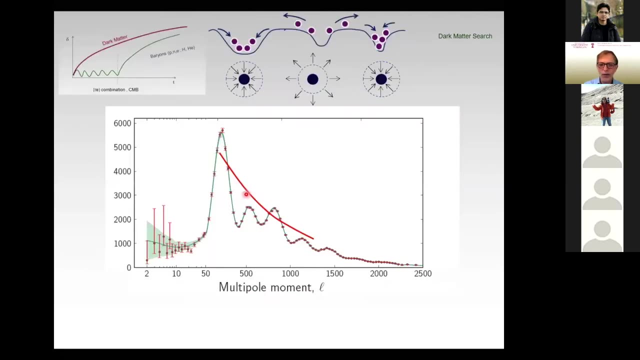 So they cannot be the solution. We need something which is non-relativistic long before that And that usually tells asks for heavier dark matter, or at least dark matter which is non-relativistic at that time. Okay, So if that is the case, 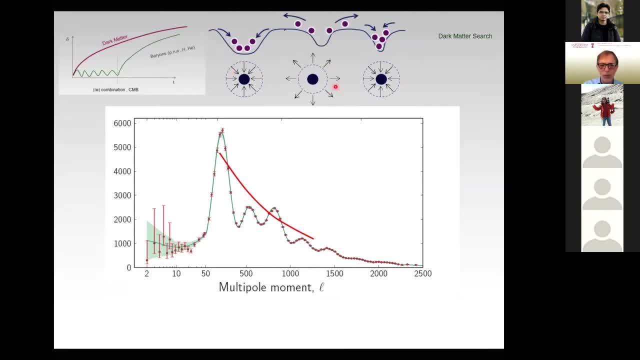 then these oscillations which we saw before, these compressions and these expansions and these compressions, these are compressions of baryons which fall into the potential wells prepared by the dark matter. So there is already a structure which is static, which doesn't oscillate. 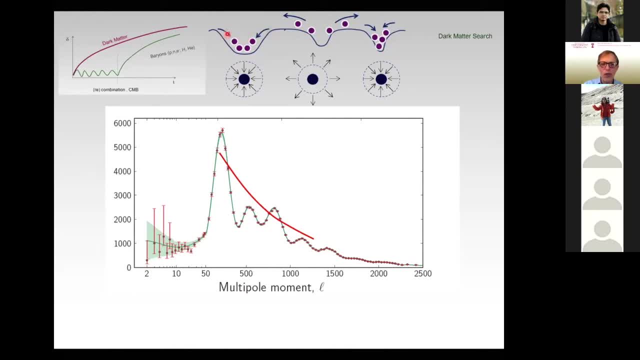 And the baryonic oscillations we see fall into these wells and have to climb out of these wells. So and if you look at the pattern here and you draw an average exponential decay of these peaks, you see that if you draw such a line, 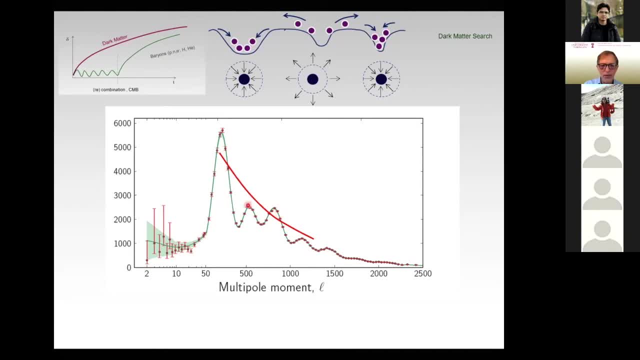 the first and the third peak is higher, the second and the fourth peak is lower, And that shows what I'm saying. that are actually. this is a visible proof of dark matter, actually, Because it tells you that the compression peaks somehow are enhanced by something. 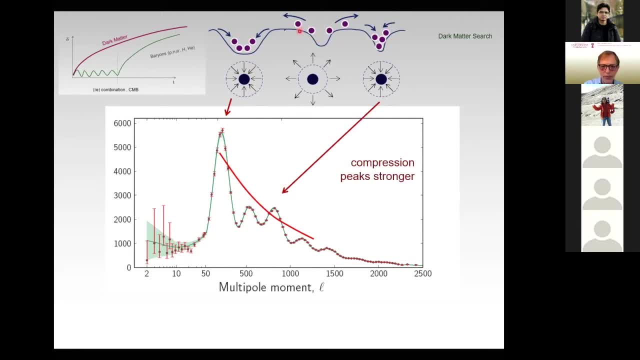 and the decompression peaks are weakened by something. And this discrepancy between the even and the odd peaks shows you that there is a structure, a static structure of non-charged matter already existing when this oscillation happens. So there are charged part, so the charged particles. 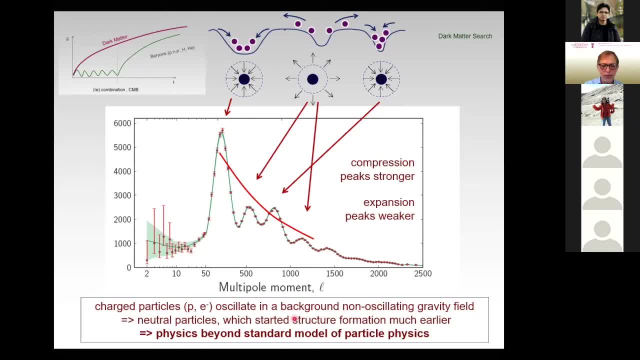 oscillate in the background of non-oscillating gravity field. So this gravity field is made of neutral particles, which started structure formation much, much earlier, And this is a proof. So here you can see dark matter by eye, And that's a proof of physics. 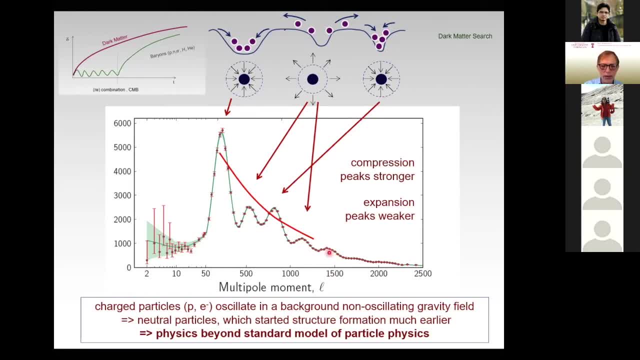 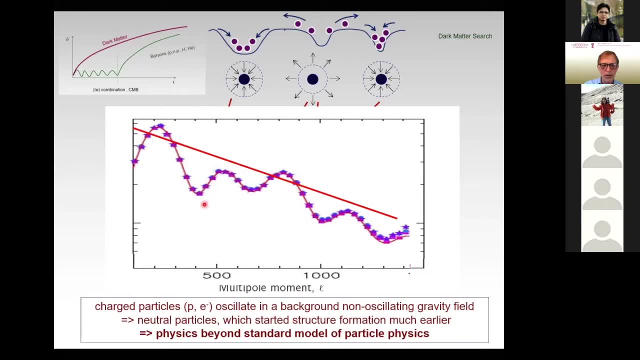 beyond the standard model must be at work here, because the standard model doesn't provide the particles to explain that. Actually, this picture is much, much nicer. if you draw it in a double logarithmic shape, then this exponential decay is a line, And here that's the same picture. 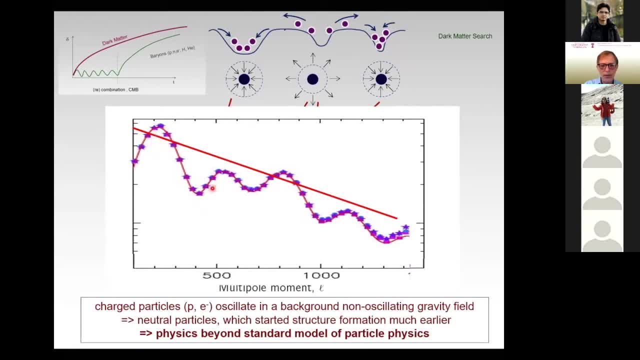 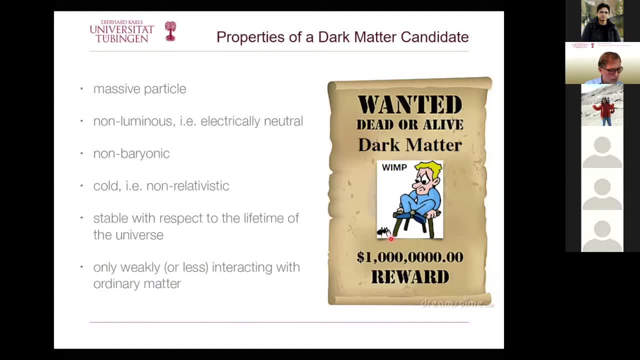 as before, just double logarithmic, And you see this discrepancy between the even and the odd peaks. So what we are looking for are massive particles, non-luminous, non-baryonic cold, which means non-relativistic, either heavy or so heavy. 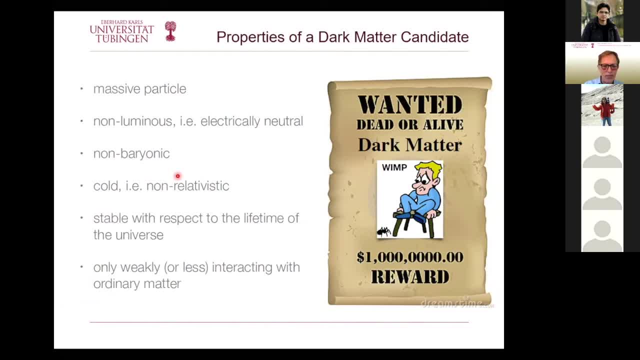 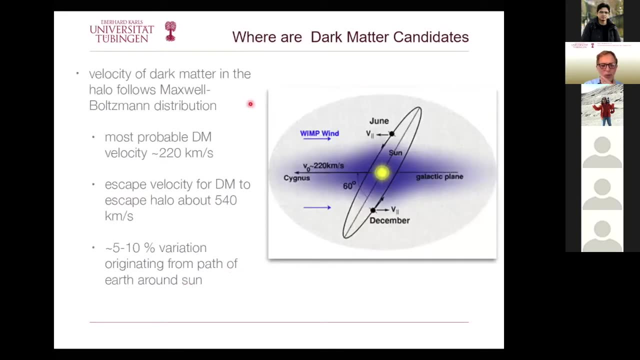 that they are non-relativistic already at that time or non-relativistic born. They must be stable with respect to the lifetime of the universe And they are only weak or less interacting with ordinary matter. Okay, So when we come to the detection, 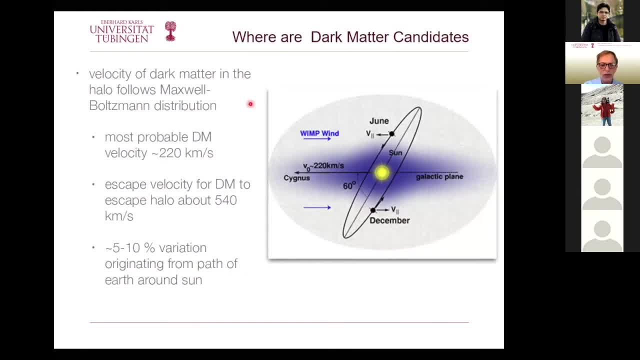 actually the question is: how many dark matter do we have here and what are the properties? So if this is our solar system, we know something. We know that the sun is circulating around the galactic center, So we have a distribution like a halo of dark matter. 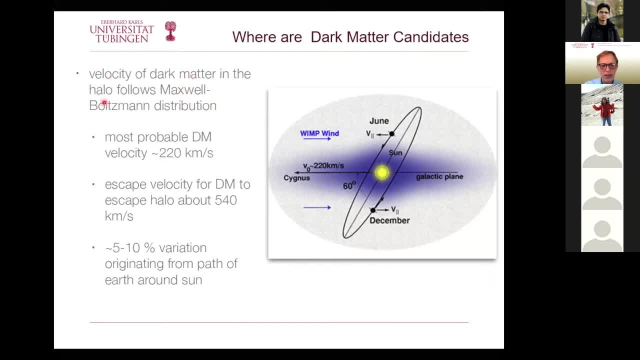 around our galaxy And the speed distribution follows a Maxwell-Boltzmann distribution that comes from the structure formation of the galaxy. So it's actually not a thermal distribution, but it looks like a Maxwell-Boltzmann distribution And the most probable dark matter speed. 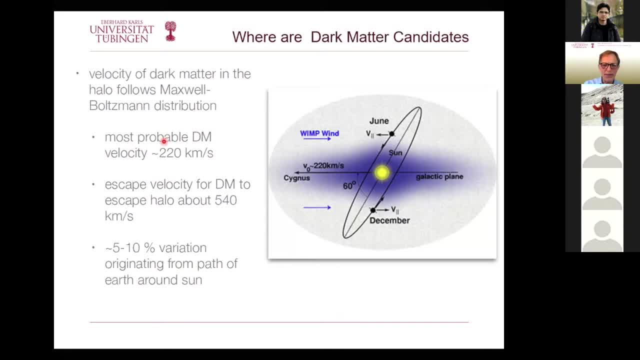 in. that corresponds to the speed the solar system is orbiting around the galactic center, And these are 220 kilometers per second. The escape velocity from our galaxy is 540 kilometers per second, So any particle which is faster than this can evaporate away from our galaxy. 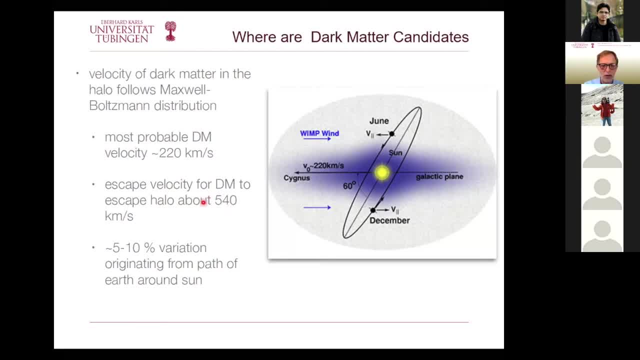 So we assume the distribution to be cut off there. And then there is a variation in the speed distribution of a few percent due to the orbiting Earth around the sun. So in summer our speed adds to the speed of the sun, In winter it is subtracted. 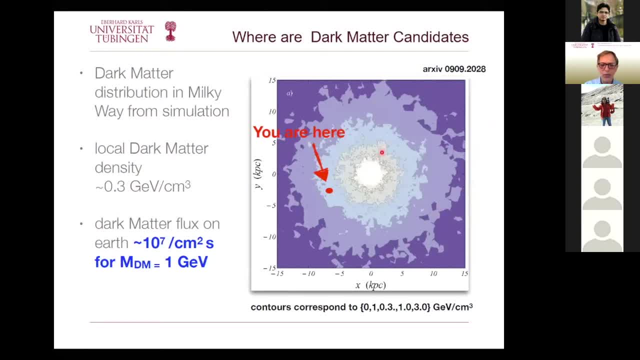 And then, if this is based on the Milky Way, from above, we are somewhere here And from simulations and calculations and measurements of the rotational speeds of objects in our galaxy, we can derive the density of dark matter at our position, And this corresponds to 0.3 GeV. 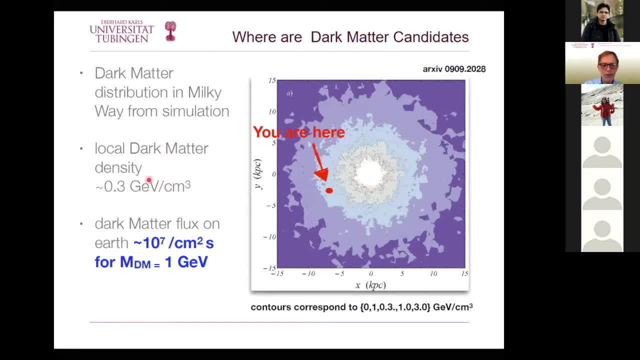 per cubic centimeters. So this means if we have 100 GeV dark matter particle we must have three per liter. So if you have one liter, a bottle of one liter, so this is roughly one liter. And if the dark matter particles, 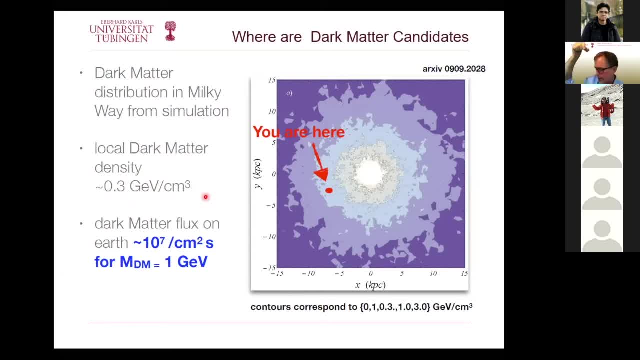 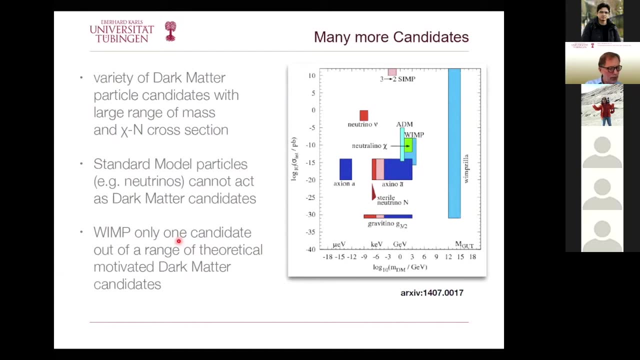 have 100 GeV. there are three particles in this bottle all the time, But they are not static. they have a speed which is given basically by the rotational speed of the Earth around the sun. Okay, the next thing is: what are the candidates? 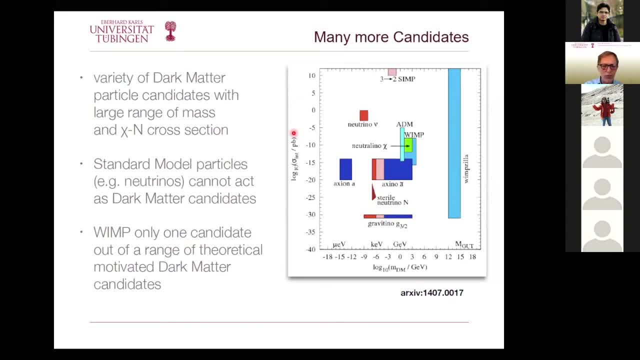 So we know it's beyond the standard model. but what are possible? ideas, of course, And there is a huge variety of ideas. So you know, theoreticians are very imaginative and they can imagine a lot of particles, And some are more motivated. 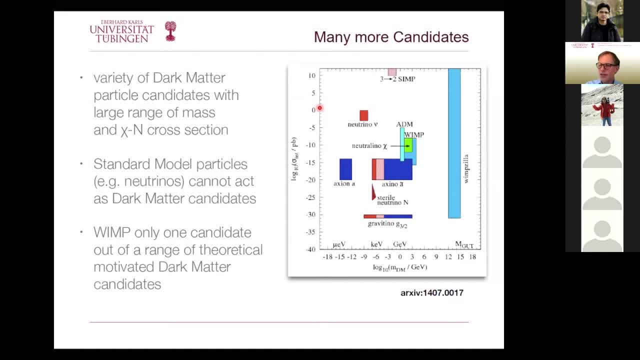 some are a little bit less motivated and the fashions can change from time to time. For example, 20 years ago the classical WIMP was very fashionable because we expected supersymmetry to be at work and the LHC at CERN. 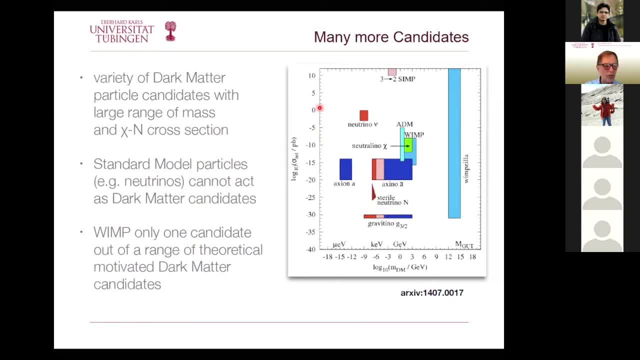 was built to look for supersymmetry, and supersymmetry provides very natural candidates for WIMPs, So WIMPs are here. So these are basically the interaction of this dark matter particle with ordinary matter, and this is the mass of the particles. 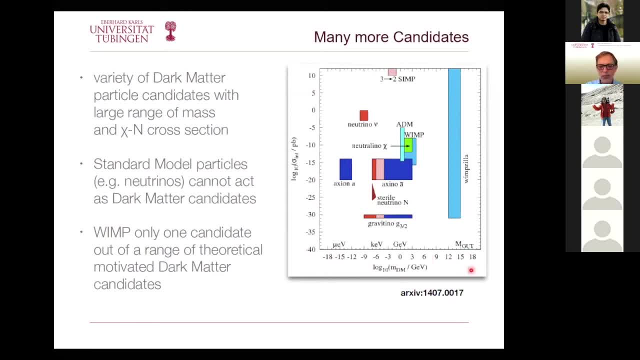 And you see, we have ideas about many, many orders of magnitude in mass and many, many orders of magnitude in the interaction with ordinary matter. And WIMPs are here, and I will talk a little bit about WIMPs. And then there are things like the axion. 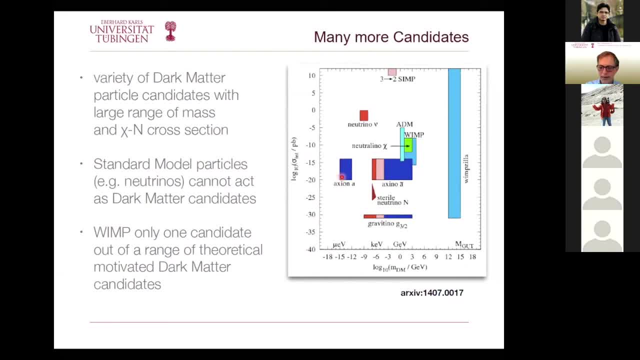 which I think is also extremely well motivated why, at the end, I will talk a little bit about axion as well. So I mainly talk about WIMPs and axions. And okay, there are other particles like the axino. They are from supersymmetry. 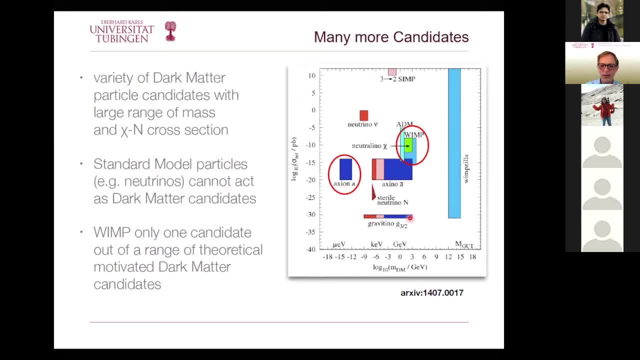 They are no more fashionable anymore. Gravitino is a possibility, which is also from supersymmetry. Then there are very heavy particles. could as well be, but they are very difficult to detect. Here are still neutrinos. They are meanwhile excluded also. 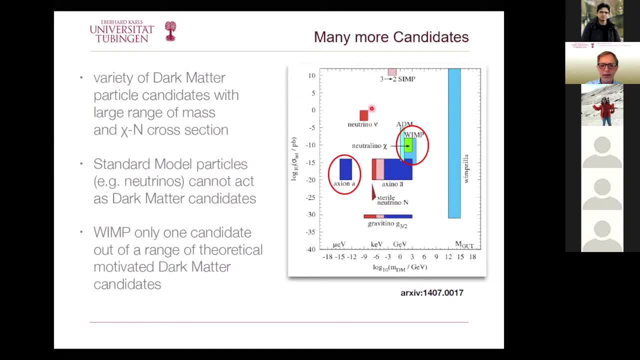 from direct detection experiments And, as I said, they don't help because they are too relativistic, because they are too light. They are too relativistic at the time of recombination and cannot form the structures. Axions actually are even lighter. 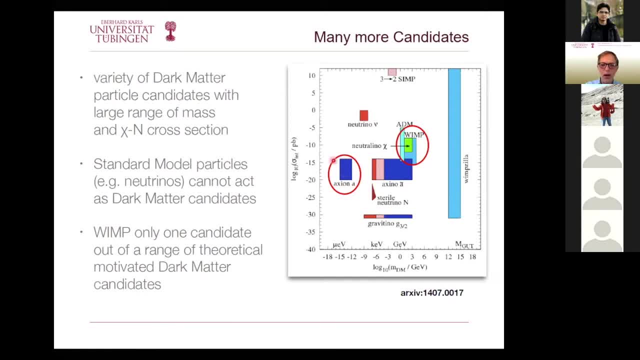 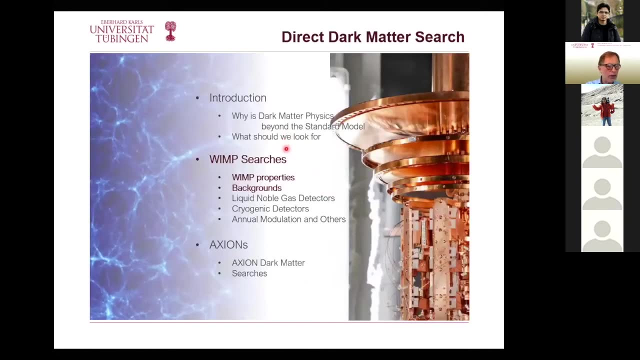 but their production mechanism is such that they are born cold. They are born non-relativistic, So that's an escape from having a light mass but still being a heavy, a cold, dark matter candidate. Okay, So then let's come to the next point. 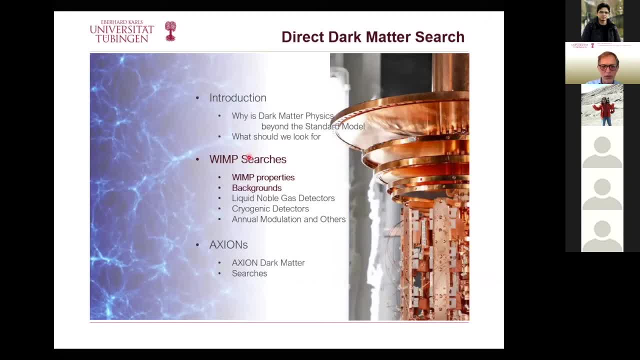 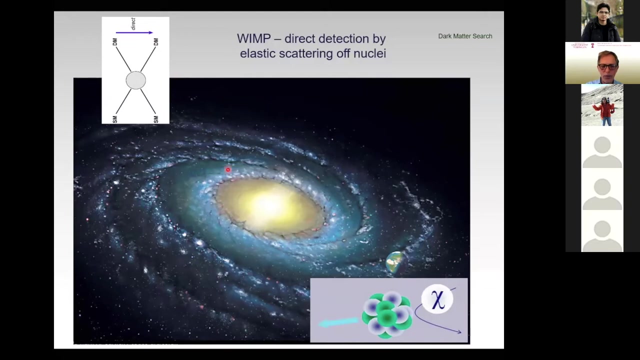 which is WIMP searches. So let me see where we are in time. So I better jump here a little bit, Sorry, Okay, So what are we looking for? We are looking for direct detection means We hope this WIMP is there. 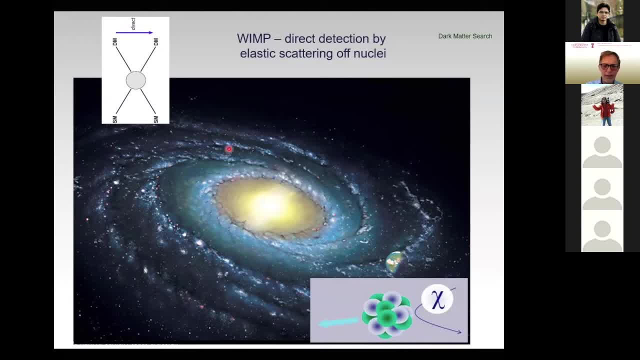 and this hope is justified because the Earth sits in the Milky Way and the Milky Way is embedded in the halo of dark matter. So, if this dark matter has an interaction with ordinary matter- which, by the way, is also well motivated because to bring dark matter 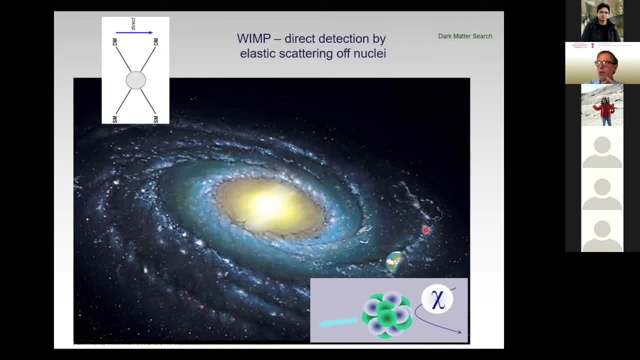 into the universe, in the thermal bath at the Big Bang. you need some interaction with standard model particles. You need some interaction, Otherwise you do not have a production mechanism to bring it into life, to make dark matter existing. And the interesting thing is: 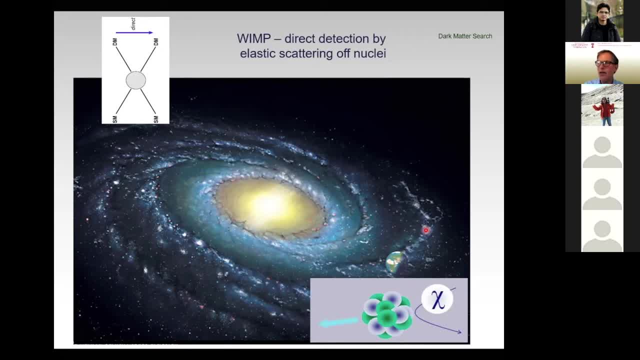 if you make the interaction with ordinary matter weaker, you are left with more of the dark matter particles. So that's why we think if the dark matter would have extremely low interaction with standard model particles, this would mean we would have a huge amount of dark matter. 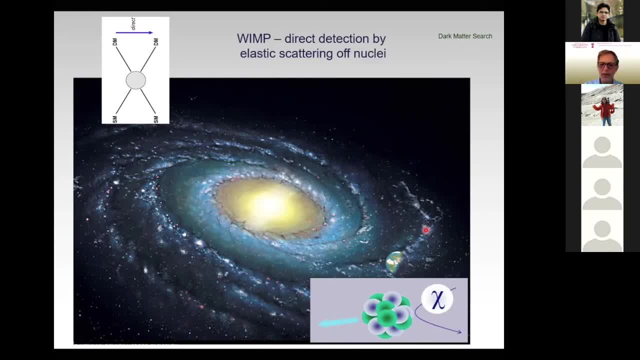 And from the dark matter we see we can even give limits to the interaction with normal matter. So this dark matter must have at least a minimum interaction with ordinary matter, which is in the order of the weak scale. So we could hope that such a dark matter particle. 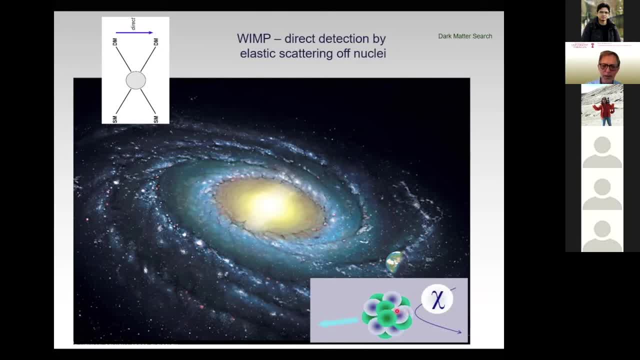 a WIMP can scatter with a nucleus and kick it, give it some speed. So all the standard detection mechanisms like ionization don't work because this particle is not charged. but we can hope for interaction with a nucleus, to give a nucleus a little bit of kinetic energy. 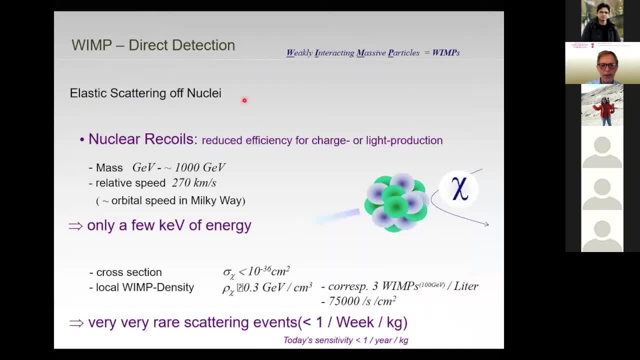 So we look for elastic scattering of nuclei from WIMPs. WIMPs stands for Weakly Interactive Massive Particles, So we need some weak interaction. we need this particle to be massive, to be cold, dark matter, and we want it to scatter elastically. 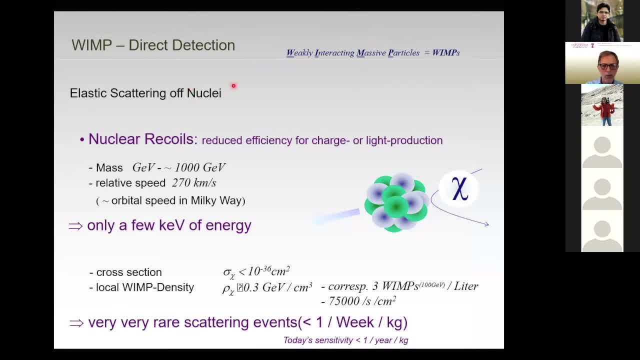 from nuclei. So we look for nuclear recoils and the mass is is in the order of 1 GeV to 1000 GeV, So it is comparable to the nucleus. A nucleus has, let's say, 100 GeV mass. 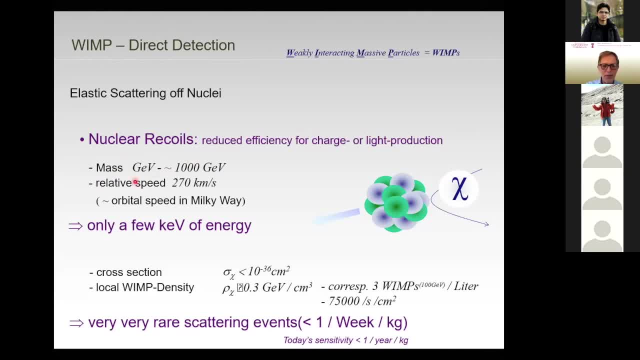 and the WIMP has the same. The relative speed is 270 kilometers per second, which is roughly one thousandth of the light speed. And if this WIMP is as heavy as the nucleus, the maximum kinetic energy transfer is that the WIMP 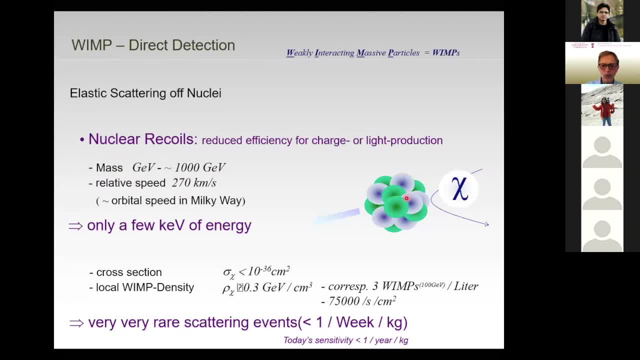 transfers all its kinetic energy to the, to the nucleus, And this is a few KeV of energy. So this is the first big challenge for direct detection. A few KeV energy is a very low energy for detectors. In addition, this is a few KeV of energy. 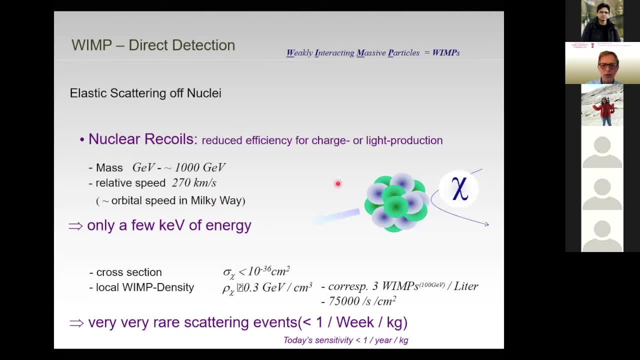 in the nuclear recoil. And the nuclear recoil, other than an electron of this energy or other than a photon of this energy, has a reduced efficiency for charge or light production. All hello, Okay. So if, if there is a problem, 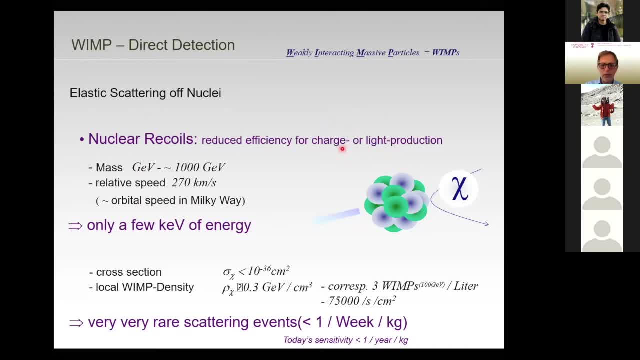 please interrupt me. So the the detectors work with charge or light production. So you ionize a gas or you ionize a semiconductor, or you produce light in a in a scintillator, But these are all interactions from electromagnetic interaction. 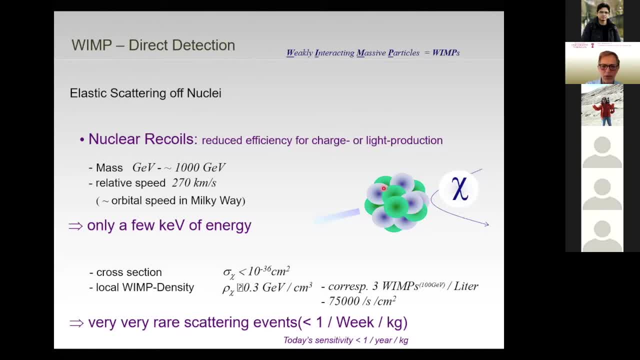 And this is uncharged And this nucleus also is uncharged, So it has a reduced efficiency of charge or light protection. So this makes the detection of a few KeV of energy even harder. The next problem is the rate you can expect. 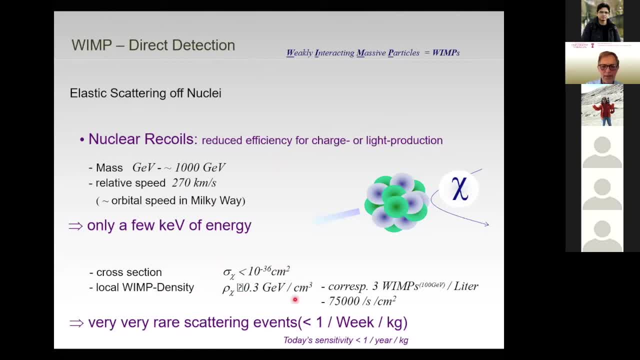 So from the cross sections and the local WIMP density and the local WIMP flux, you can calculate how many scatterings you can expect. And that's a very, very low rate. It's a you immediately end up with one per week per kilogram. 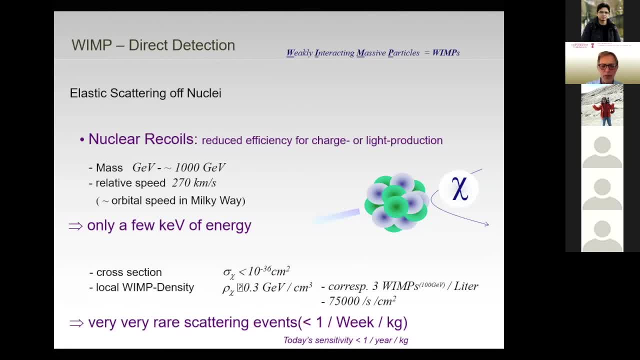 And actually today's sensitivity is much, much better than this. We are down to one per year per kilogram, or even below now, So it's extremely low rate. So low energy, low rate. these are the challenges, And the low rate is a challenge. 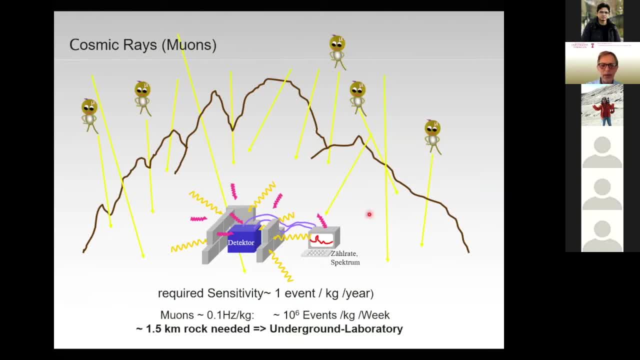 because you need to shield it. You need to shield your experiment from from other radiation which causes signals, And first there is the cosmic radiations. From cosmic rays which hit our atmosphere, there are many, many muons being produced in the atmosphere. 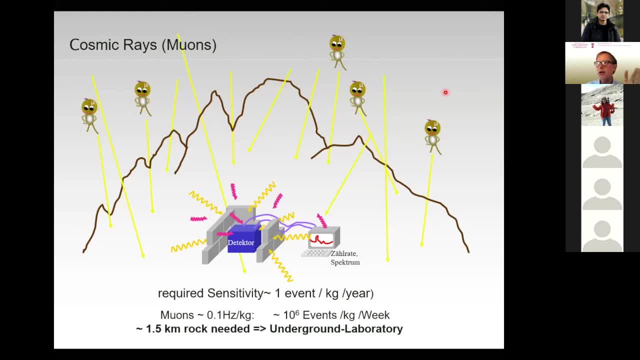 Actually there are 100 per square meter per second on the earth And if you put a detector on in your laboratory it will be hit several times a second by cosmic ray muons And you need to reduce that to a level of one event per year. 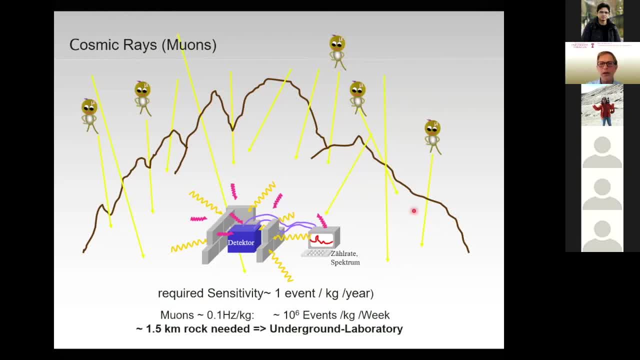 And this means you have to reduce the muon flux by a factor of a million or so, And this requires 1.5 kilometers of rock. Yes, and this means this puts all these direct detection experiments in underground laboratories, Otherwise you are overwhelmed by cosmic rays. 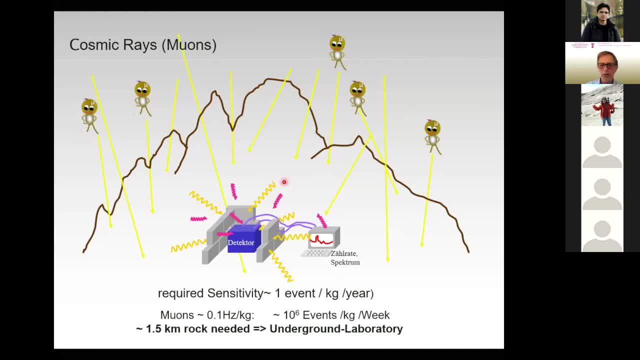 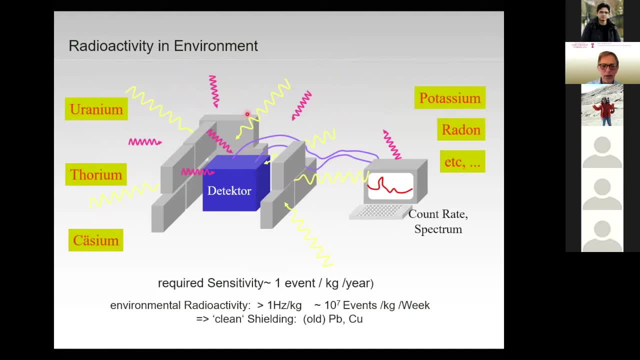 But even then, if you are underground, your detector will fire a lot of signals because of ambient radiation, And this is a very important part of the physical activity. So there is almost no material which doesn't contain some uranium or some thorium. 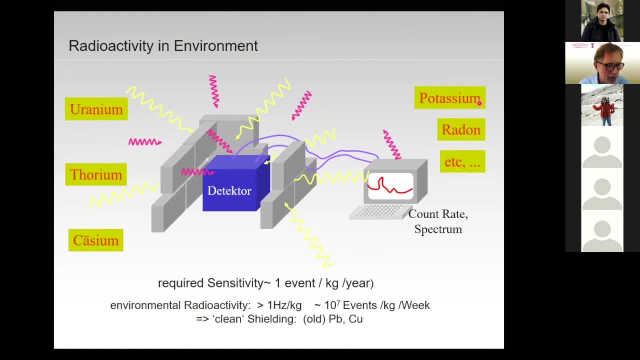 Or potassium, is also abundant. Potassium is also a radioactive element which is even in your body, So the main radioactivity in your body comes from potassium, And if you touch something, your fingerprint contains potassium, which is enough to produce radioactivity. 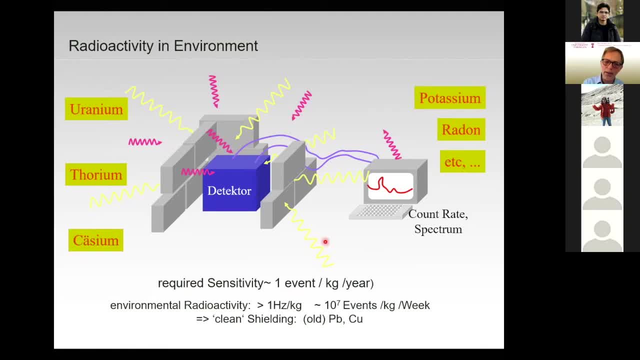 So you need to reduce the environmental radioactivity a lot, And that's why direct detection experiments are an art in selecting materials, in choosing your proper materials. You even need to clean the air from radioactivity And you have to do a very, very careful shielding. 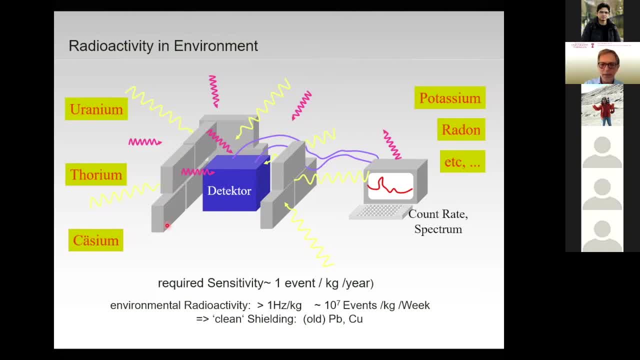 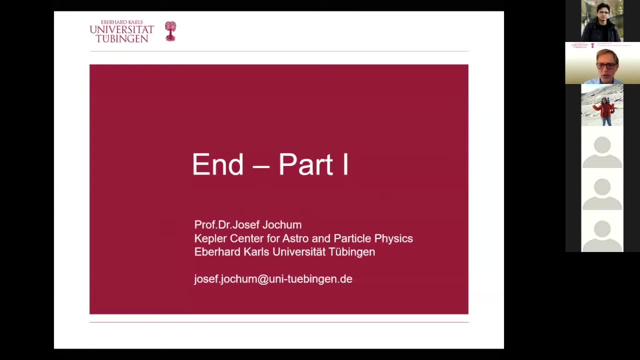 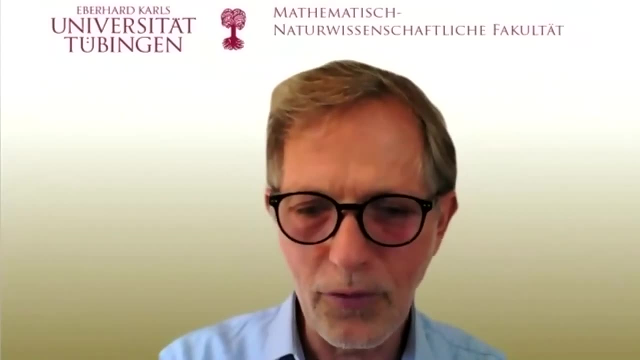 of your detectors from the surrounding. Okay, This is the end of my first part, which means only I have to switch to swap the files. Let me just for a second. Hello, it's me, So if you wish, you could ask questions right now. 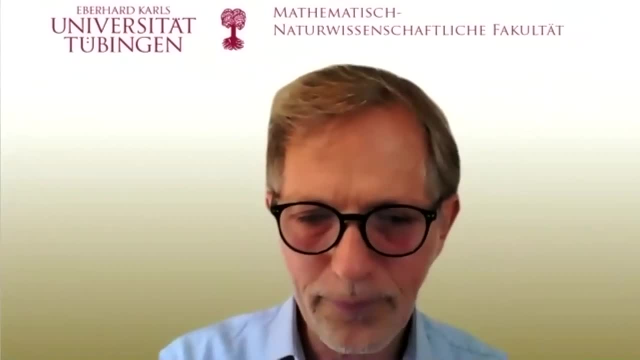 but I will swap the file, which will take only a few seconds. You are still here. I don't hear anybody. Hesti, you are still listening. Yes, We still have no questions. Okay, Okay, That's fine, Okay. 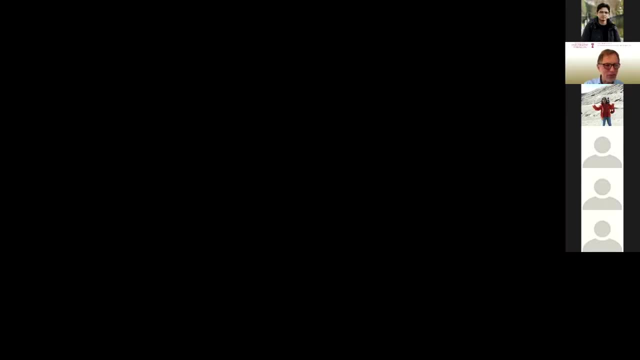 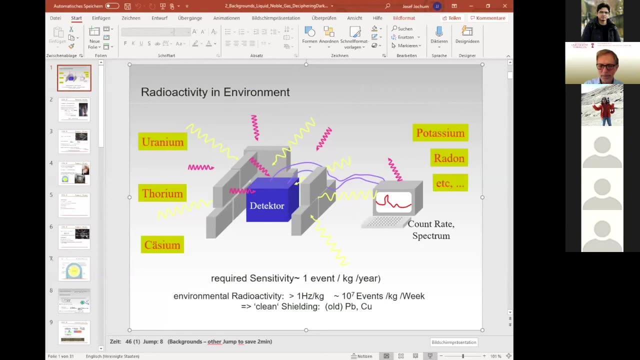 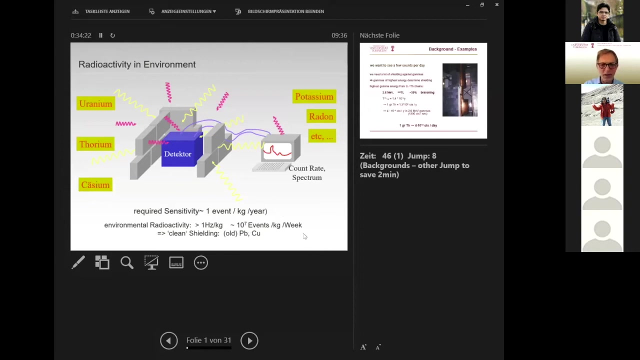 I go ahead. Okay, So I come to the second part right now. So I have always 45 minutes lots of files. That's why, Okay, Now we are in the second part And I think I have time to go into an example of background. 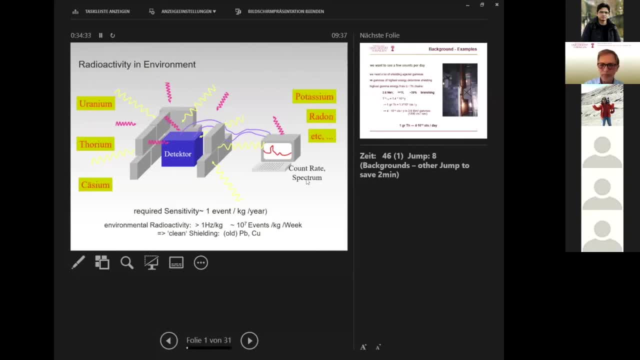 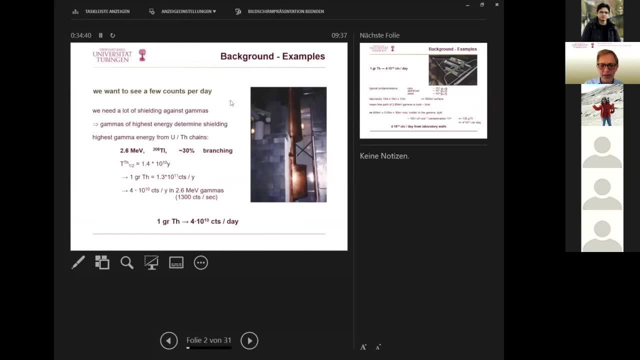 just to illustrate what it means, Let me spend a few minutes on one of the examples. So we want to see a few counts per day in an experiment. That's actually a picture of the CREST experiment. This is a cryostat. 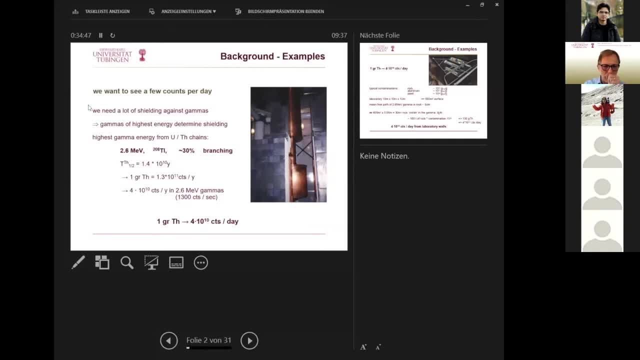 I will come to that later. And so, as I said, the surrounding of your laboratory has uranium in it And we need a lot of shielding against these gammas. Since we need a lot of shielding against gammas anyway, it's enough to consider. the highest energy gamma, Because we need to shield the highest energy gamma, Then the low energy gammas will also be shielded away. So if you have a thick shielding, all the low energy is shielded, but the highest energy is the most penetrating. 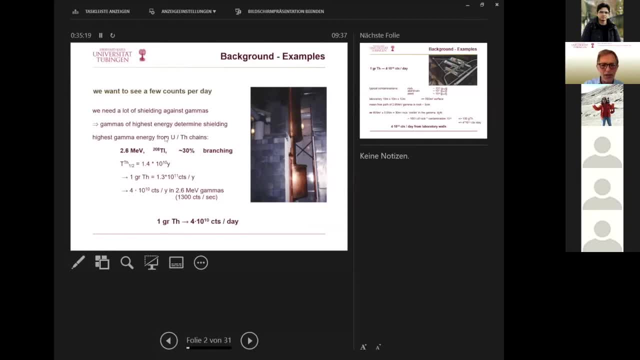 And the highest energy gamma in the uranium-thorium chains is a 2.6 MeV gamma from thallium. And okay, here are the numbers. But if you go through the numbers you will find that one gram of thallium 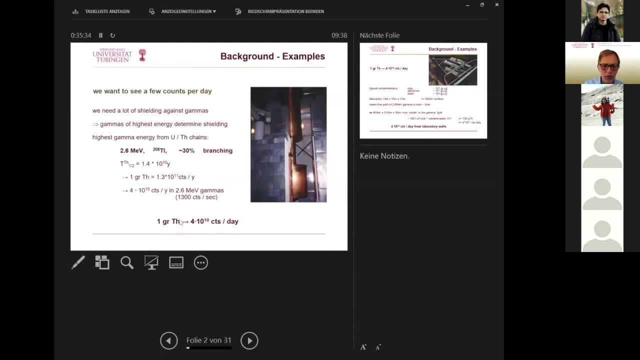 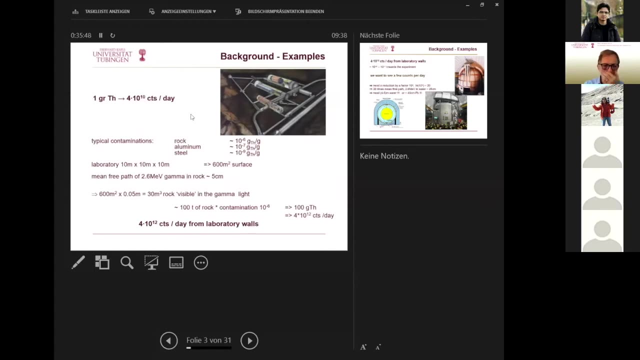 produces four. sorry, one gram of thallium produces, of this, 2.6 MeV. four times 10 to the 10 counts per day. So one gram brings you 40 billion counts per day. So this is the number Now. contaminations of thallium in rock. 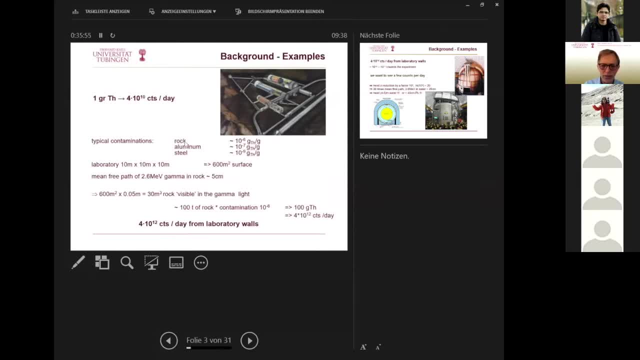 let's look for rock, because we are in an underground laboratory, so we have rock around us. So typical contamination of thallium in rock is 10 to the minus six grams per gram, So one gram in one ton of material. So the laboratory. 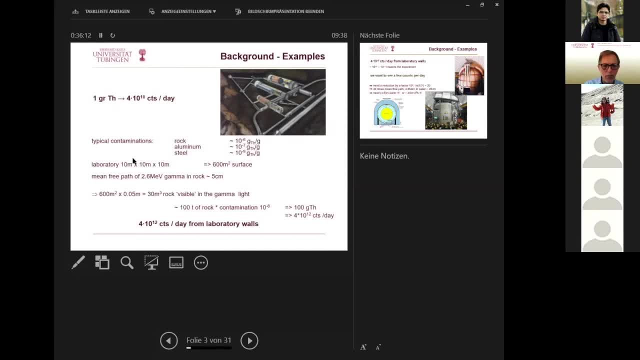 let's have the laboratory. make it simple, Let be the laboratory a cube of 10 by 10 by 10 meters. This means we see 600 square meters. Can you change the mode Because we can see your notes? Ah, we see. 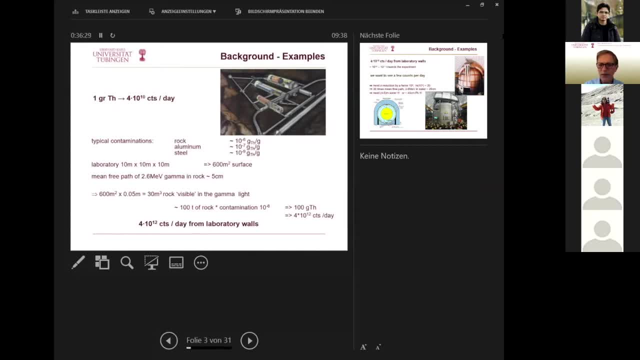 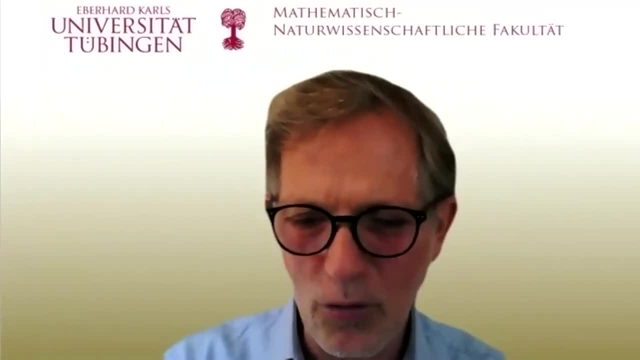 Ah, sorry, This is okay. Sorry, You see my notes. Okay, let me just stop. Okay, you're right, Thank you, I should have realized. I see, I don't know why this happened, but let's see. 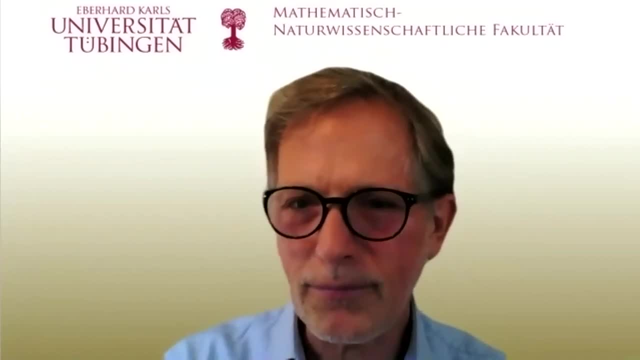 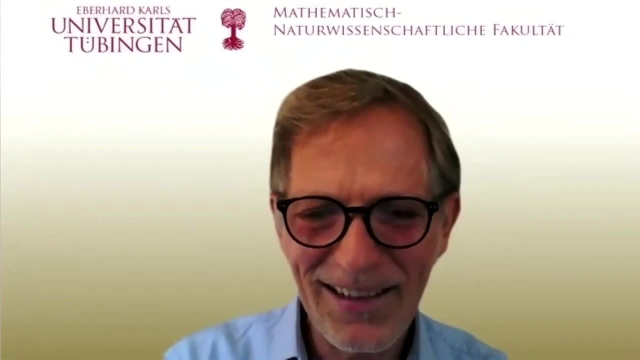 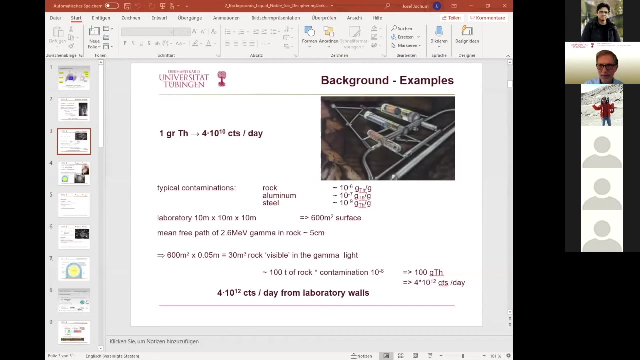 I have to stop this, I guess. Okay, Thanks for telling me. So that's okay, let me try again. Let me go back to the background. So now, Okay, Well, it's still. you still see, and I 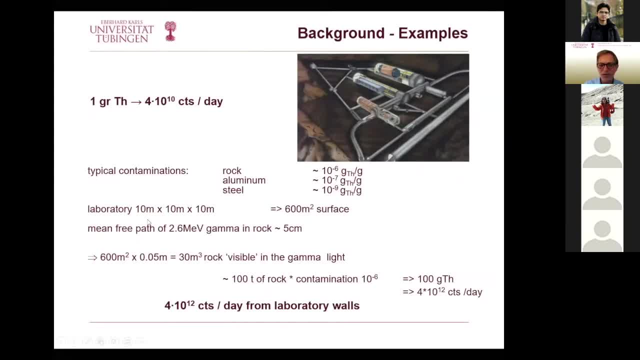 but I need my, I need this to you. So now you should. now it's fine, all right, Yes, Okay, Okay, Thank you. So let me, let me go back again. So we? I told you that one gram of thorium. 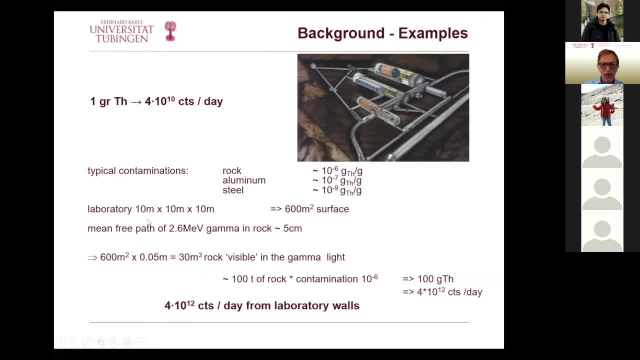 produces these four times 10 to 10 counts, And then a rock has a contamination of 10 to the minus six grams of thorium per gram of rock. Then the lab has a size of 10 by 10 by 10 meters. 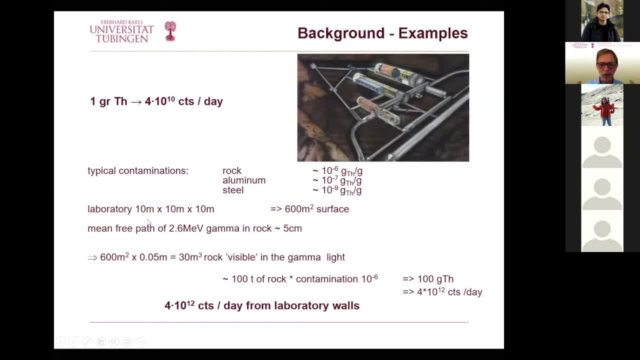 which means we see 600 square meters of rock around us. At 2.6 MeV, gamma has in rock roughly a mean free pass of five centimeters, So we see the rock in this light of this photon five centimeter deep. 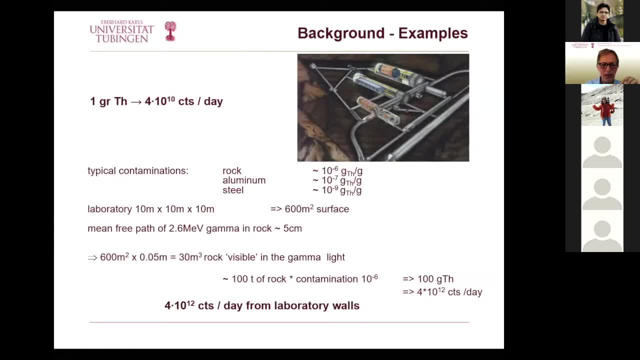 So we see 600 square meters by five centimeters. We basically see these are 30 cubic meters of rock are visible in this gamma light. So these are 200 tons of rock around us emitting these photons with the contamination of 10 to the minus six. 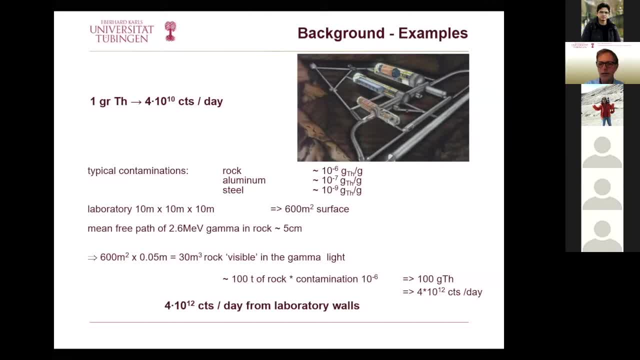 we have a hundred grams thorium around us. So that's, that's normal. That's also in any building. you have that around you. So this brings us to four times 10 to 12 counts from the laboratory walls in this 2.6 MeV gamma. 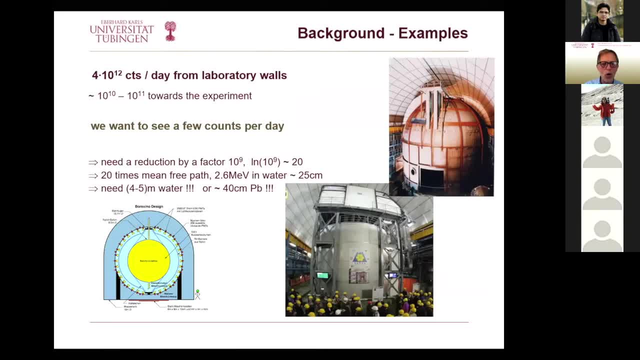 So this number here, So let's assume 1% of this goes into the direction of your experiment. Most of them go in all directions. They don't hit your experiment, but let's, let's assume a 1%. So this still gives us a number of 10 to the 10.. 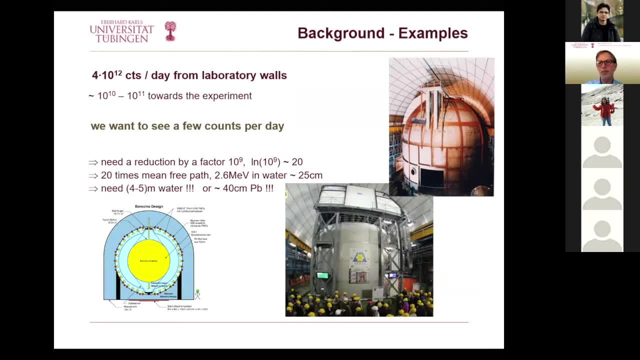 And we want to see a few counts per day. And this already tells you that you need to reduce the photons, these 2.6 MeV gammas, by a factor of 10 to the nine, or 10 to the 10 or so. 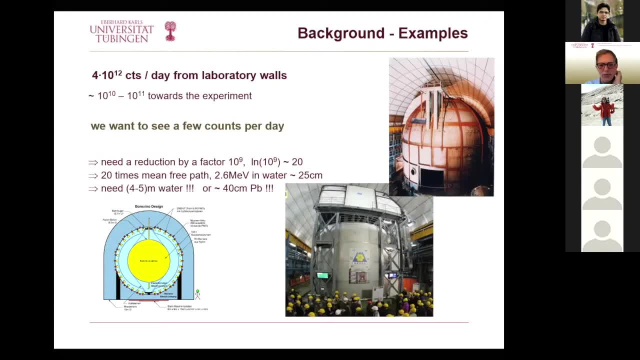 So you need to reduce it by nine, 10 orders of magnitude. The logarithm of 10 to the nine, the natural logarithm is roughly 20.. This means we need 20 times the mean free pass of this photon. And the simplest way to shield your experiment. 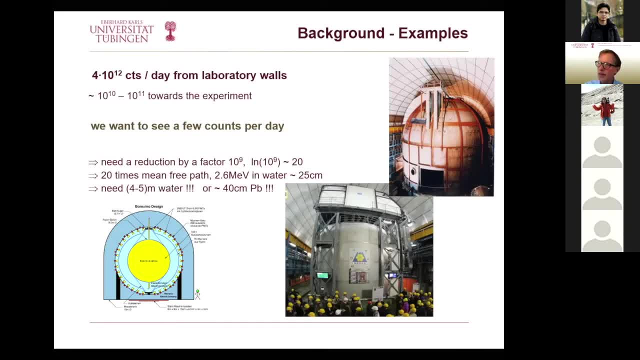 is by using water, because that's an inexpensive shielding material. In water, the 2.6 MeV photon has a mean free pass of 25 centimeters. You need 20 times this way, So you need four to five meters of water. 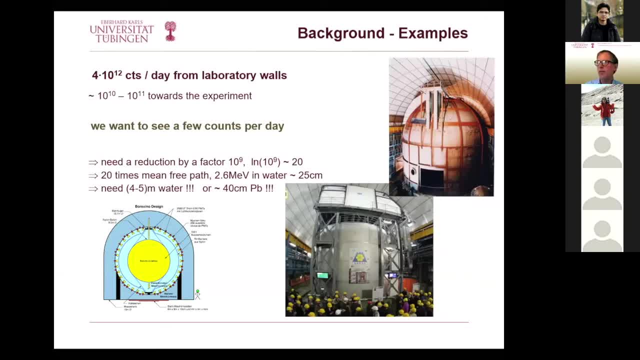 around you to shield your experiment. So that's why all these experiments, or most of these experiments today, sit in huge 10 meter diameter water tanks. You start with a 10 meter diameter water tank and put your experiment inside, And that's because of mainly two of these gammas. 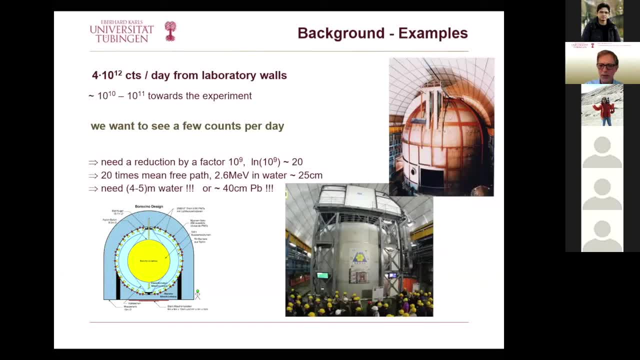 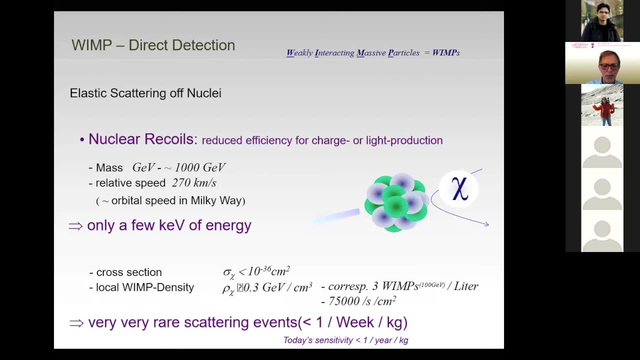 to reduce them to the level which we want to see. Okay, So now let me see where I go. Okay, Okay. So this was the question of the low scattering rate. Now let's come to the low energy, which is also a challenge. 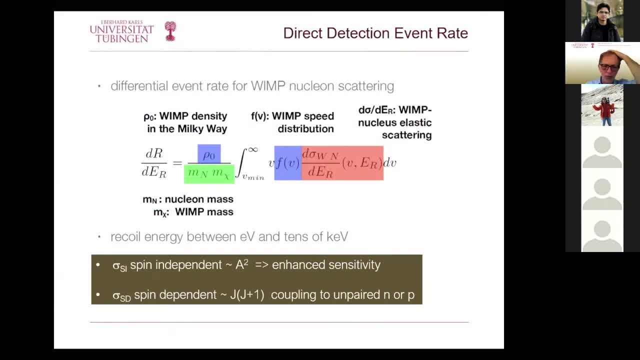 If you look to the, if you calculate the energy spectrum you expect, so which is the rate per recoil energy? So this is the spectrum you expect. You can calculate that And the calculation is basically given by. okay, it's a cross section. 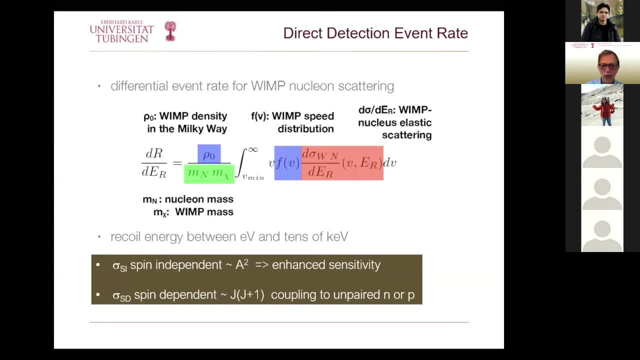 So this is particle physics. Here your model of the WIMP in particle physics goes in. It tells you which cross section you have. Then you take the speed distribution of the particles around the Milky Way. So that's astrophysics. So that's basically the halo distribution. 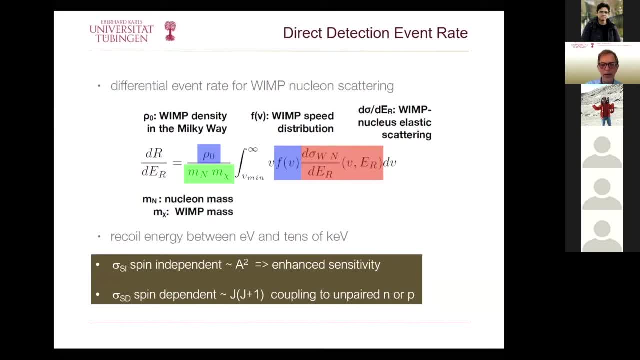 This is also astrophysics And you convolute that and you get a spectrum. Before I show you the spectrum again, it gives you a recoil energy in the EV to KEV range. But what I want to say here still is that 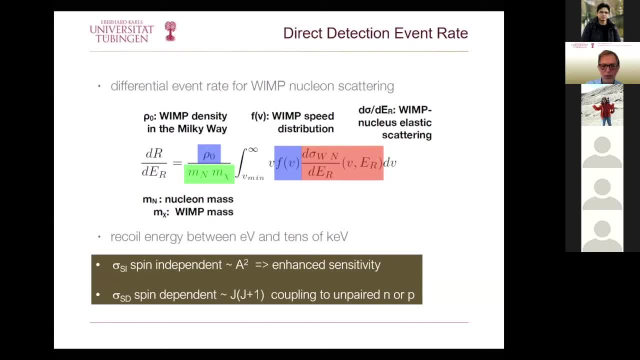 given this cross section, you can have two possibilities which are mainly considered. So usually we add low energies, we are non-relativistic, We assume an energy independent cross section And it can be spin independent. This means you scatter coherently. 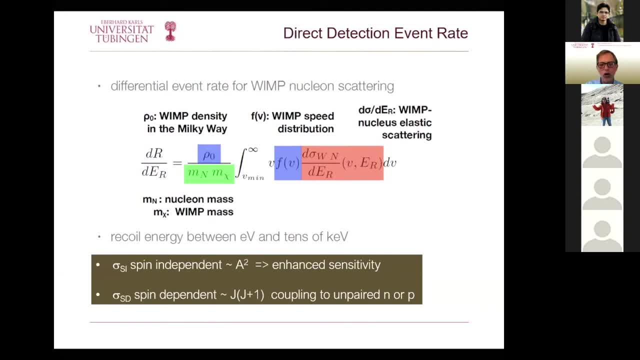 on all nucleons or on all quarks in your nucleus, And this gives you a coherence factor of A squared, Because the energies are so low that the wavelength, the proly wavelength, is larger than the nucleus. So you get the coherence factor and this enhances the sensitivity. 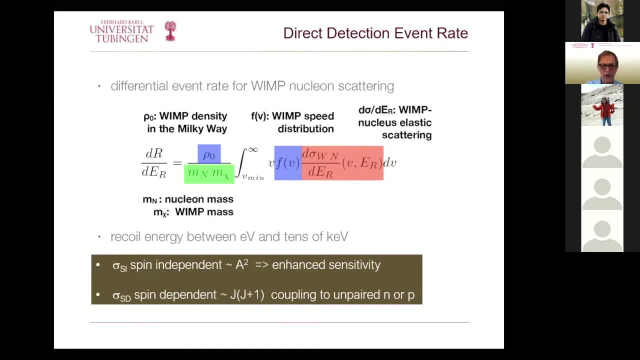 So you have a higher cross section here if you have larger nuclei. That's why usually this is the most popular looked at in dark matter searches. But you can also be spin dependent depending on the properties of your WIMP. you are looking at And then only one nucleon. 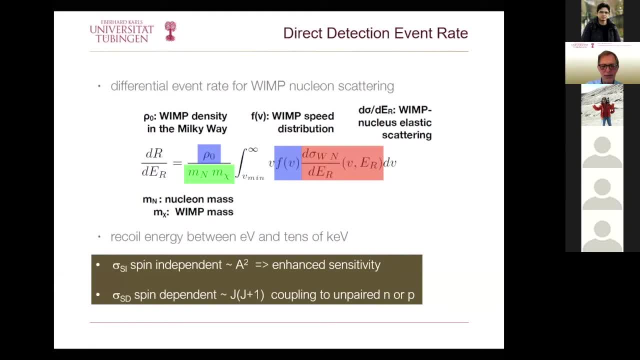 the unpaired nucleon is responsible for the scattering. This could be an unpaired neutron or unpaired proton, And you are much less sensitive, But you look to different kinds of WIMP particles, So that's why both are looked at. 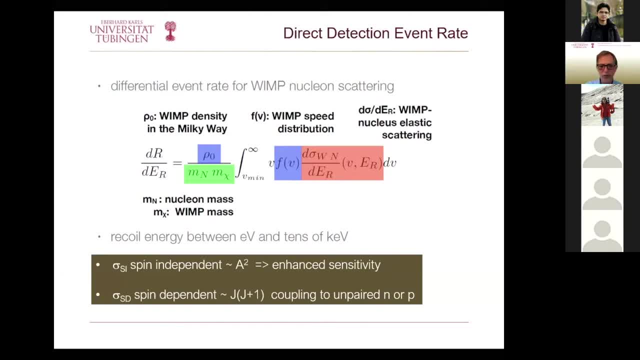 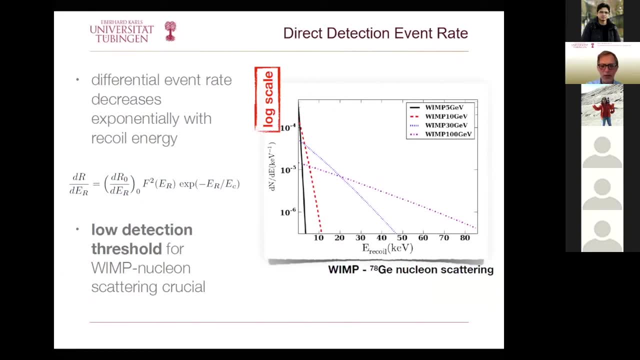 But this is the most, yes, the most fashionable one. Okay, the spectra, they look featureless on a logarithmic scale. The recalled spectra just look exponential. So they look like a line, So they look exponential, So this is exponential spectrum. 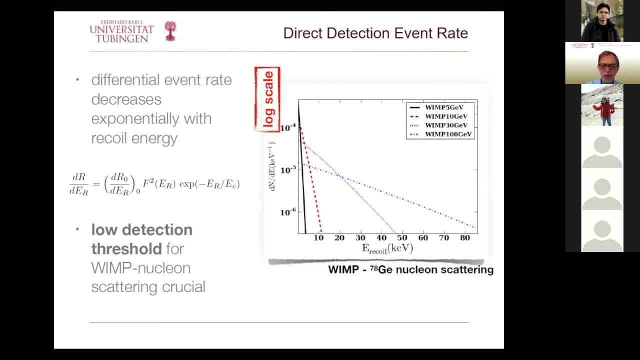 in a semi-logarithmic plot. This is a line. It's peaking towards low energy. And if you make the WIMP lighter and lighter, so you go here from pink to black, the WIMP gets lighter and lighter and lighter. 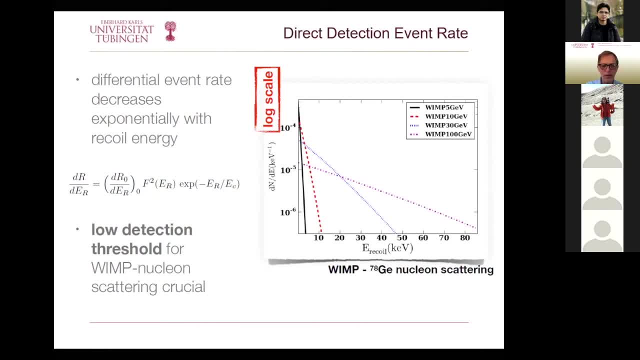 The recall. energies get lower and lower and lower, So you need to be able to see these low energy scatters. And they are even lower as lower the WIMP mass is. So a low detection threshold is the thing you need for WIMP nucleon scattering. 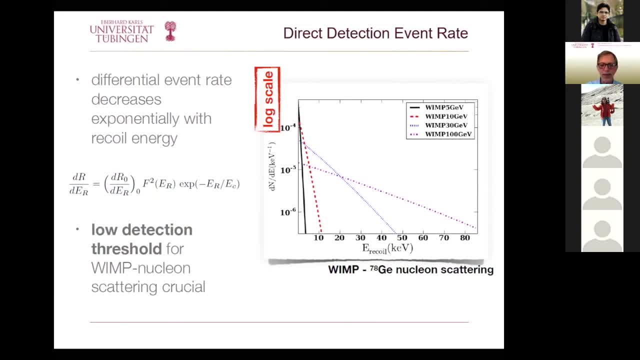 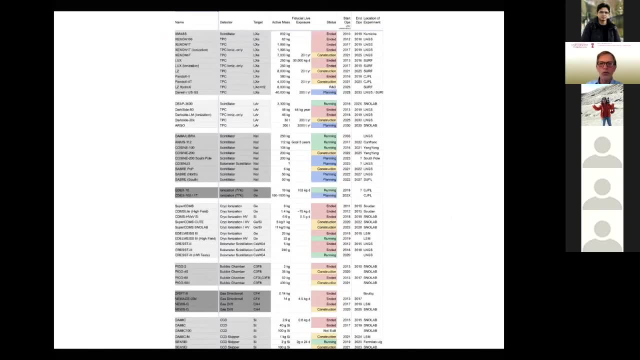 It's crucial for scattering Okay because the techniques are so challenging. there is a huge variety of dark matter searches And I do not want you to read this here. This is just the list of present running dark matter experiments And you can understand from this list. 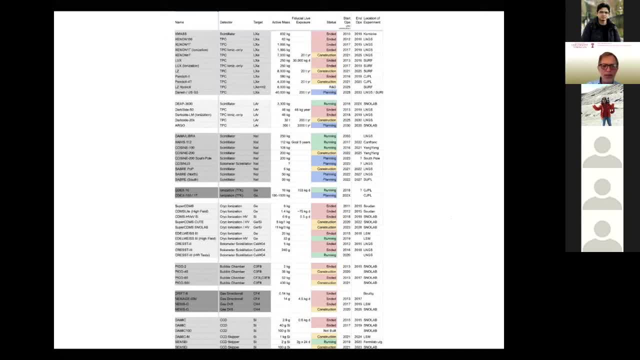 that I cannot go through all of them. So there are liquid xenon experiments, there are liquid argon experiments, there are sodium iodine experiments, there are germanium experiments, there are cryogenic experiments, there are bubble chamber experiments, there are gaseous experiments. 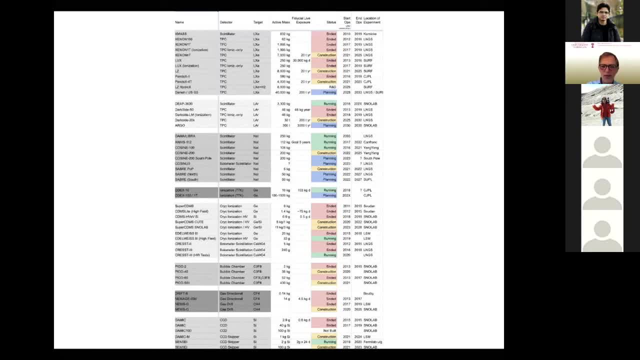 and there are solid-state CZD experiments. So there's a huge variety, and this variety is good, because we do not know what we look for. and all these have their advantages and disadvantages. I will show you the main two ones: the liquid noble gas detectors. 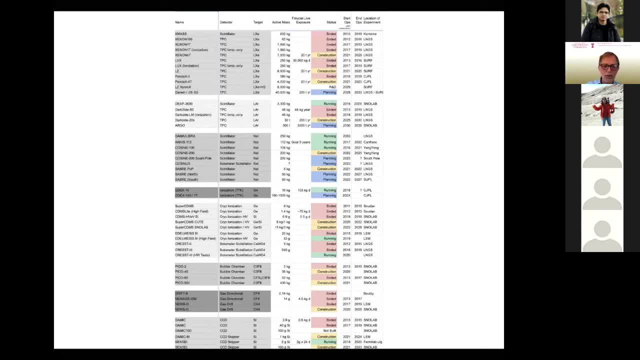 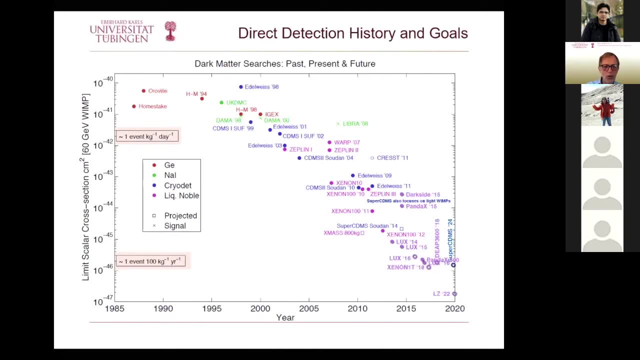 and the cryogenic detectors. and a few words on sodium iodine as well. So this is a plot which shows you the year versus the sensitivity or the limit on the cross-section which was reached in that year, And you see there is impressive progress. 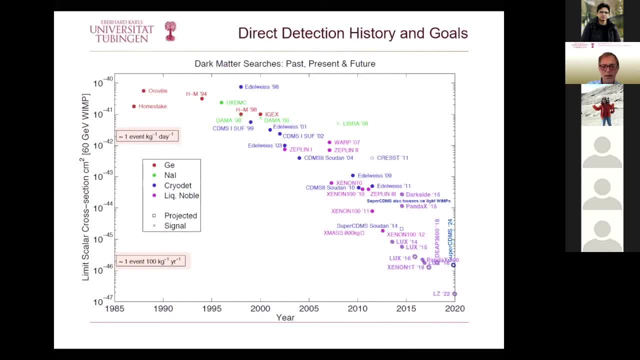 being done over the years, where the detectors get better and better and better, And the slope started in the 90s or so and this came because of the development of techniques to largely reduce the background by the detection, And this is the reason why. 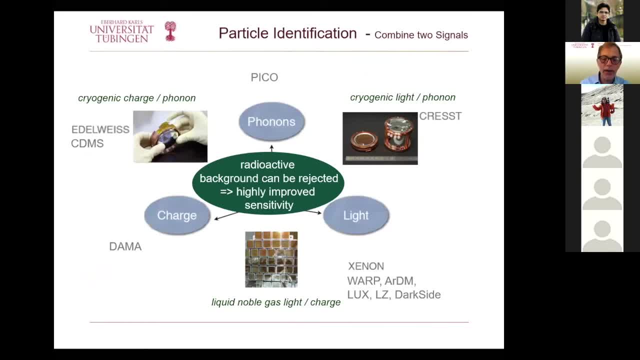 we have these detectors themselves and they have to do with particle identification And I told you that it's a disadvantage that nuclear recoils- the signal we are looking at- produce less light or less ionization than electromagnetic interacting particles. This is a disadvantage because it pushes 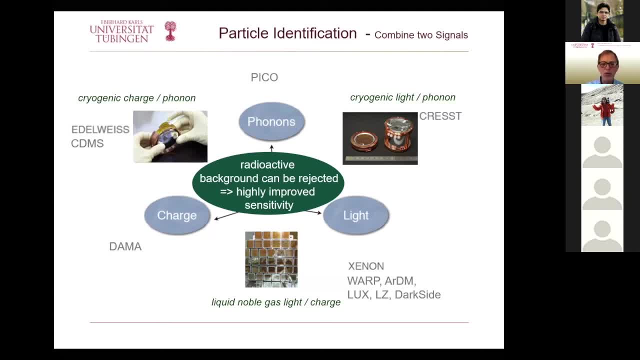 the recoil energy spectrum to even lower energies. but it can be used to recognize distinguish nuclear recoils from radioactivity, Because radioactivity is mainly alpha- it's alpha, beta and gamma radiation. they have a high yield in ionization and scintillation light. 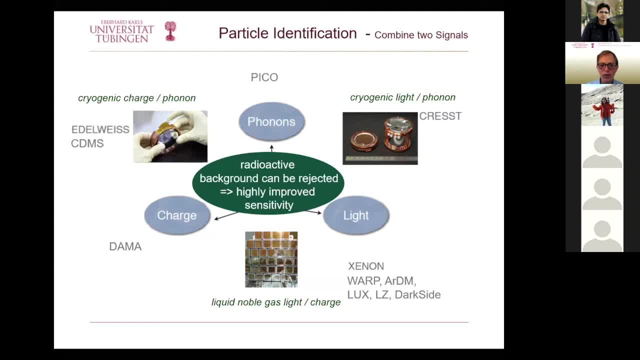 And if you can measure this yield, you can distinguish between the two. So you can reject most of the background. And to reject the background is you use different detection channels. So the classical detection channel is using charge. So this is ionization detection. 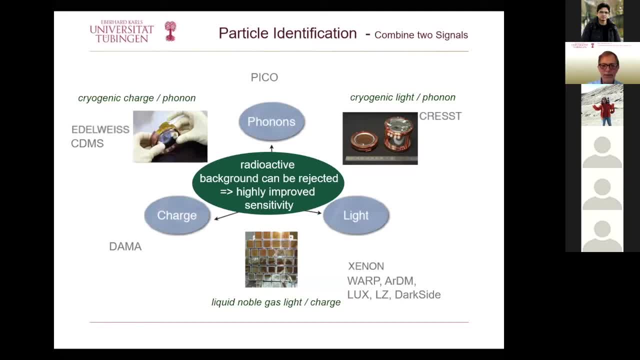 This is light, This is scintillation detectors- A new player which was developed actually for dark matter searches- are cryogenic detectors which look for phonons. Basically, they do either calorimetry or they look for the phonons. 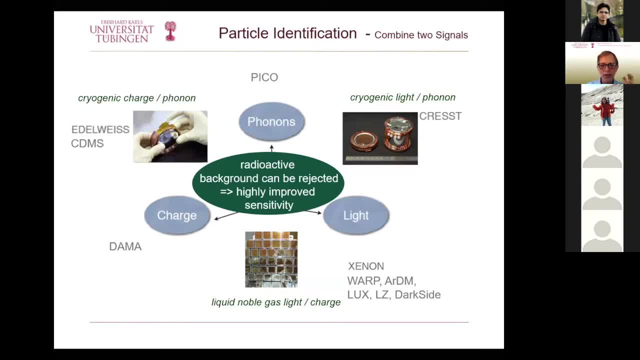 the lattice vibration in a solid created by this nuclear recoil. And if you combine the two, if you combine two of them, you can measure the ratio between the two. So you not only measure then the energy, you also measure the ratio between the two. 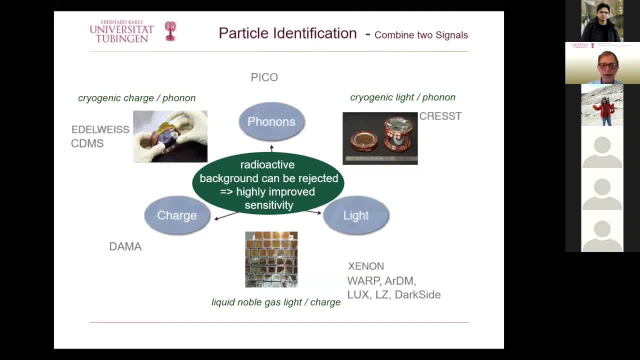 So you can measure the ratio between phonons and charge or the ratio between phonons and light, And this ratio depends on the ionization yield, And this is then a tool to distinguish between nuclear recoils and electromagnetic interactions, which are the background. 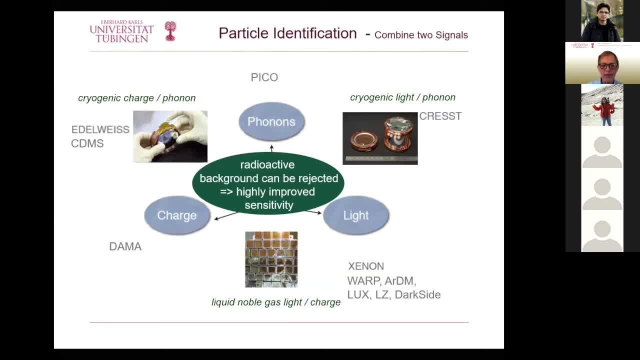 And this development started in the 90s and this caused then this steep increase in the sensitivities And phonons and charge whenever there is phonons involved. these are cryogenic detectors and they are detectors using phonons and charge. 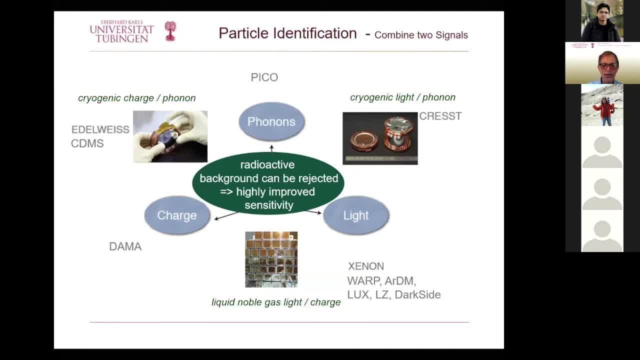 and they are detectors using phonon and light. And then charge and light is the domain of the liquid noble gas detectors which lead the field at present because they, as I will show you, they are the easiest to scale up to large, large detector volumes. 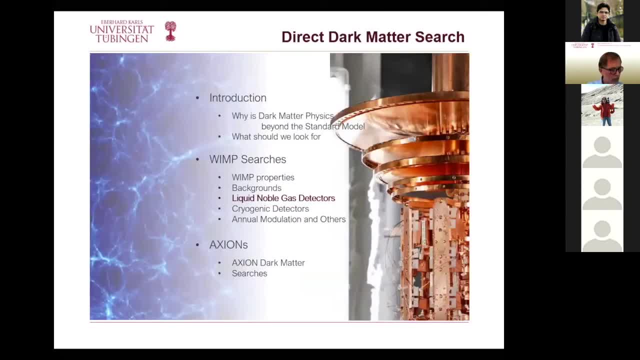 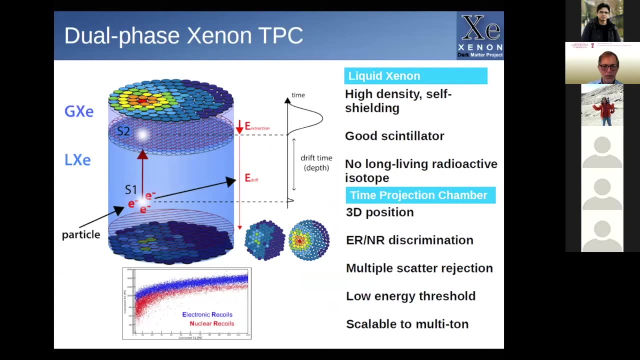 Okay, that's why I now come to the liquid noble gas detectors. Okay, so liquid noble gas is. let's assume you have a container which is filled with liquid argon or liquid xenon. These are the two layers, So this is the liquid here. 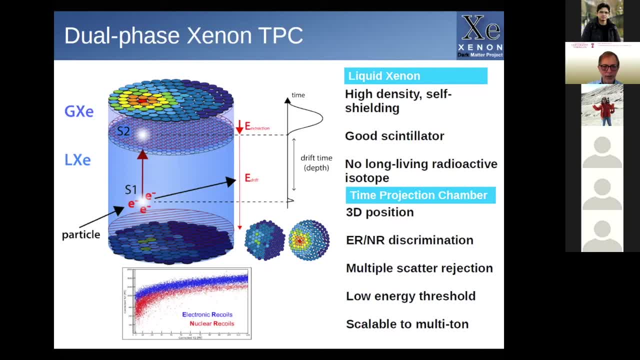 And then you have a gas above it, Then you, if there is a particle interacting in this liquid. there is the nice feature of this liquid noble gases that they scintillate And you produce also free electrons, So you ionize this liquid noble gas. 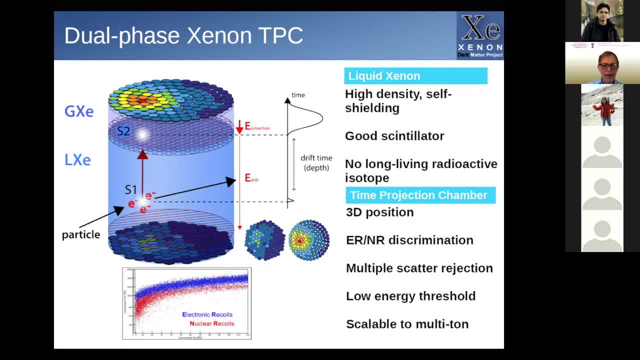 and you produce light. The light you can immediately detect with photomultipliers. So there is a photomultiplier array at the top and there is a photomultiplier array at the bottom. And you can see at the top and the bottom. 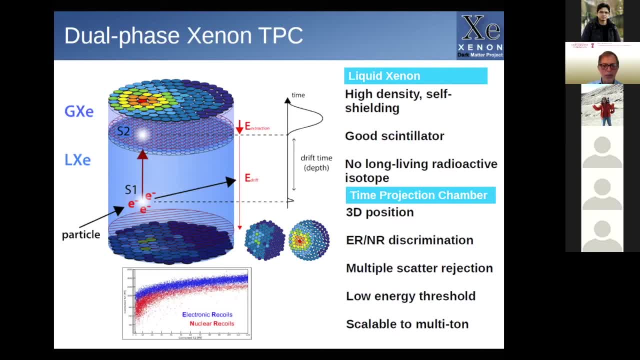 you see the hip pattern of the photons being emitted from this event. So you have already an immediate signal of the event. So here is time going from bottom to top. You have the immediate scintillation signal, But you also produce charges. And now, if you manage to measure these charges as well, 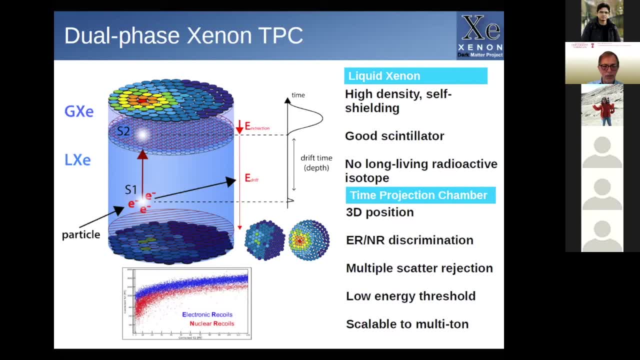 and then you get a second signal which measures the ionization, And this is done by applying an electric field to this liquid. and then these charges drift, Yes, And if they drift to the surface of the liquid, you can extract them out of the liquid. 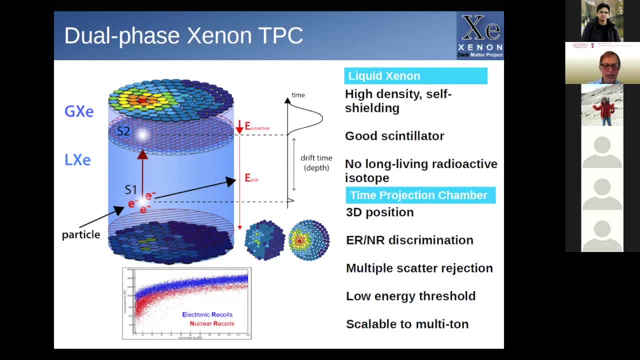 and then they make the gaseous noble gas scintillate. So you get a second scintillation signal from the gas when the charges are drifted into the gaseous phase And this takes some time. This takes the drift time for the charges to reach the surface. 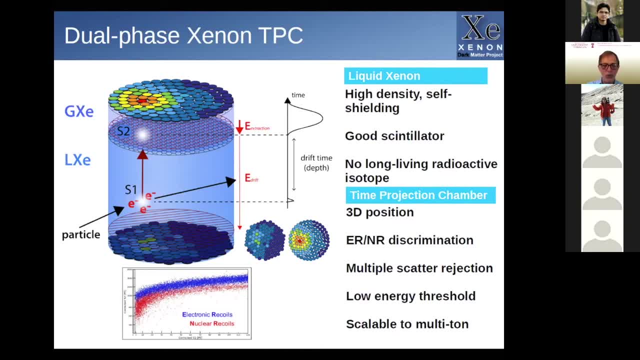 And then you get a second signal which actually is larger than the first one. So you get two signals And the nice thing is that the ratio between the two signals depends on the ionization yield, And nuclear recoils and electronic recoils have a different ratio between the two signals. 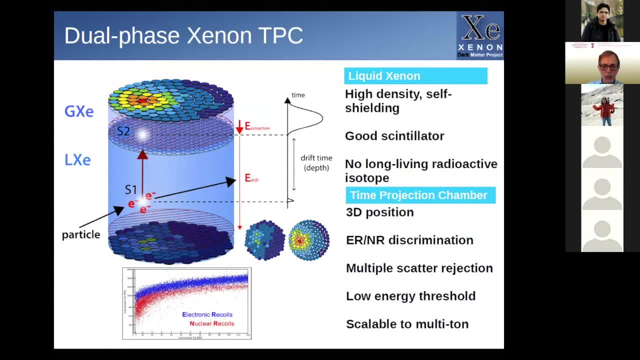 So from the ratio of the two signals you can say this was a nuclear recoil or this was a radioactivity. And if you plot that, I'm sorry you cannot read the axis. but this is a number which basically is the ratio between: 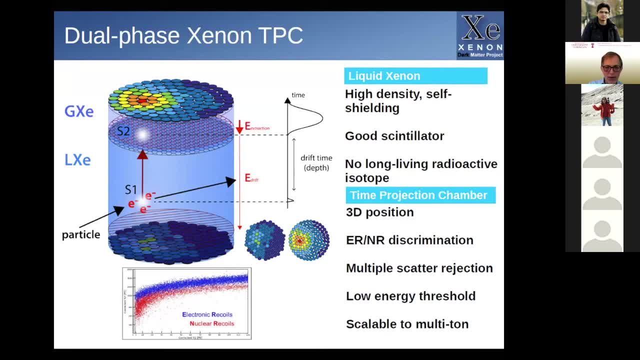 signal one and signal two, And this is the energy here. And blue are electronic recoils so caused by alpha, beta gamma rays, And red are nuclear recoils which you can measure in the experiment in using a neutron source, If you apply a neutron source, 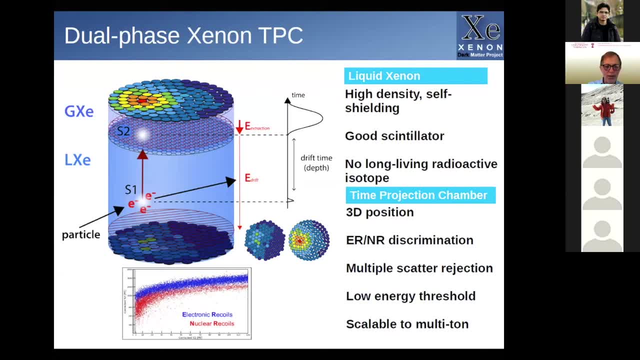 to your detector. you produce nuclear recoils and then you can measure the response of your detector And you see red and blue are not laying over each other. The one is higher, the one is lower and you can separate the two. 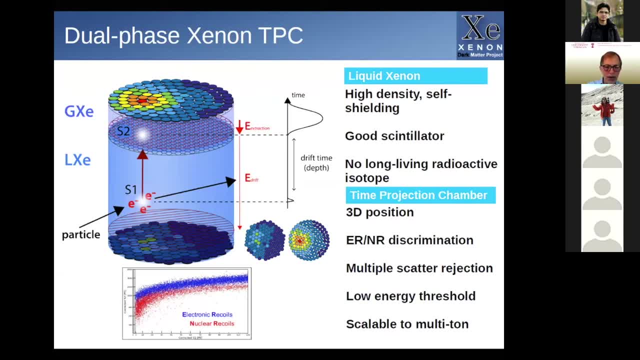 at least a little bit. You know there is an overlap, but down here you are in a clean nuclear recoil region and up here you are in a clean electronic recoil region. So this is the trick you use here. And, by the way, 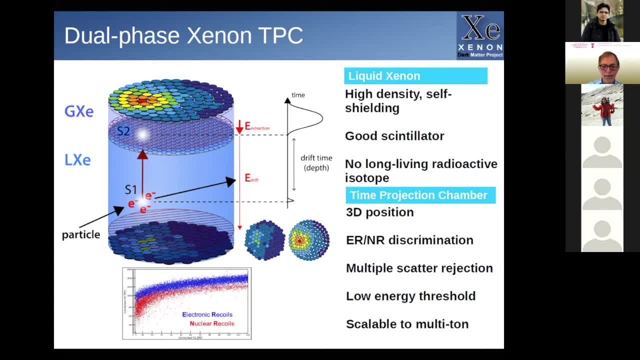 you also. by this light pattern you get the position in xy direction and by this drift time, the time between the first- sorry, the first- and the second signal, you get the set position. So you can even see where in 3D. 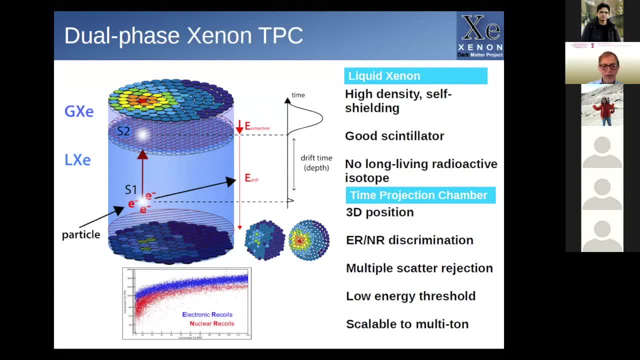 where your signal was in this detector. And the big advantage of liquid xenon detectors or liquid argon detectors is they can easily be scaled up, So it's easier to build a huge. it's very easy to build a bigger, bigger experiment. 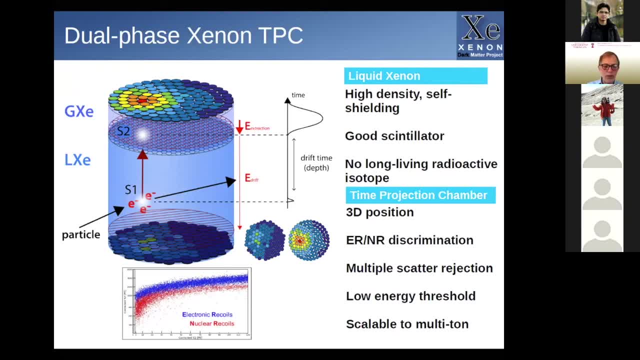 As long as you can make the charges drift to the liquid. So this is the challenge there: If you make the detector bigger, your drift paths get longer and this might cause you a problem, But okay, that's the only challenge then. 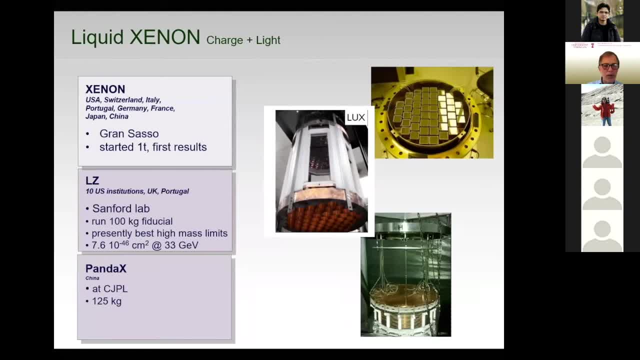 Okay, And the experiments are: the xenon experiment, which is a US-European collaboration, and it's at Gran Sasso. It has already results of a one-ton detector and is presently preparing several ton detectors, And there are other several ton detectors. in preparation. One is LSET at US. This is led by US and UK institutions, And then there's PandaX in China. This is xenon experiments. There are also argon experiments, Namely most famous is the DarkSight. 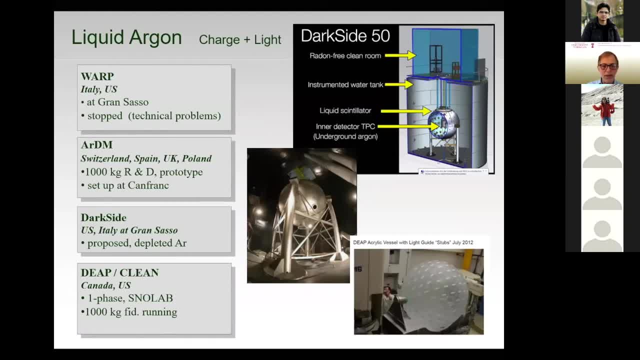 also proposing a ton scale liquid argon detector. It's being set up at Gran Sasso And they're steep clean. at Snow Lab They have already a one-ton detector running. Okay, But as an example I would like to show you the xenon experiment. 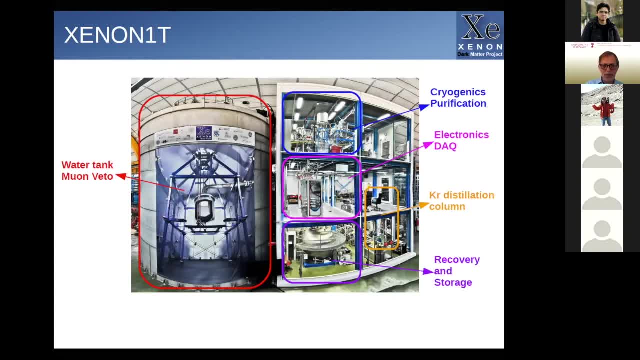 Okay, I'm a little late, I guess. Okay, It's a xenon experiment. This is sketch. So this is the tank where the detector sits in the water. So this is the 10-meter tank. The detector is in here. 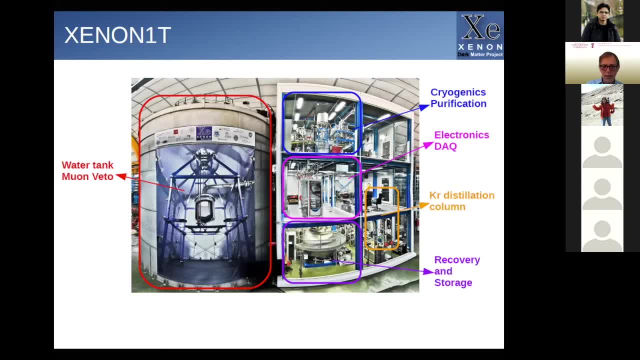 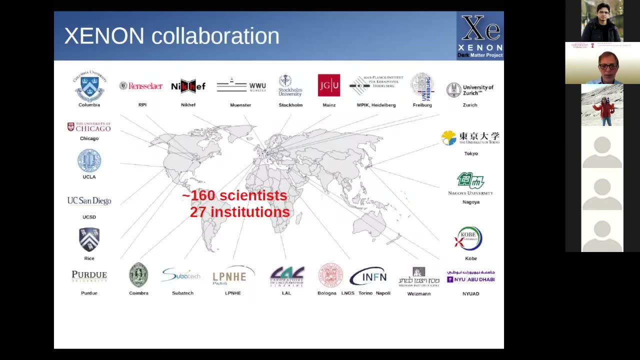 well shielded through the water. Then there is additional housing which contains a purification system. So another advantage of liquids is you can circulate a liquid and continuously purify it. Then you have a data acquisition and some storage. Xenon is an experiment. 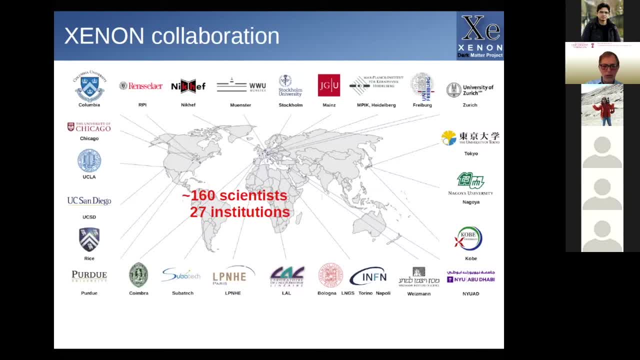 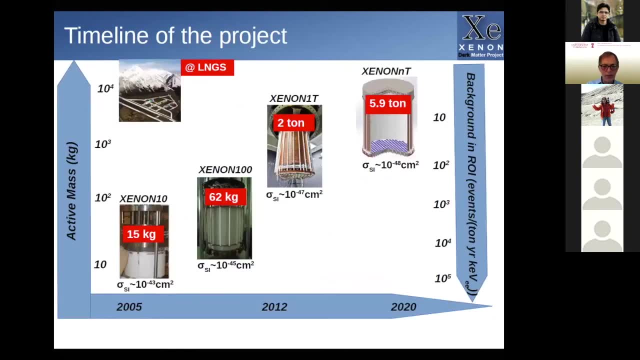 It's a huge experiment. There's a worldwide collaboration of, you see, almost 30 institutions, And it started already, yes, 15 years ago or 20 years ago, with a 15-kilogram prototype. Then it increased in size. 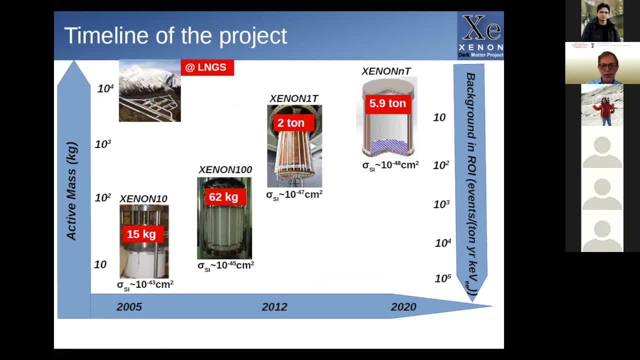 We are presently here and they are preparing this six-ton device at Gran Sasso in Italy. And while the active mass increased the sensitivity, so the background was reduced and reduced, and reduced. And you see, here we are on a level. 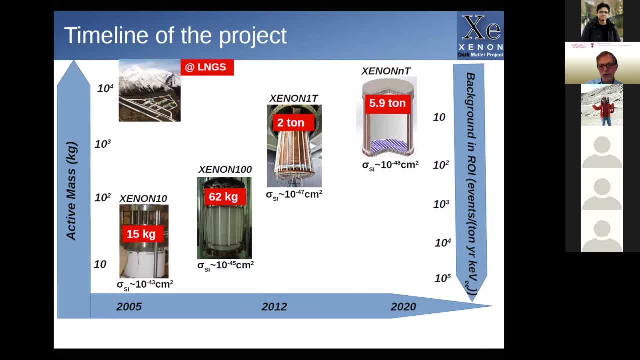 This says background in the region of interest in events per ton per year. per keV We are on the level of a few hundred events per ton per year. So this is less than one count per year in a kilogram detector. 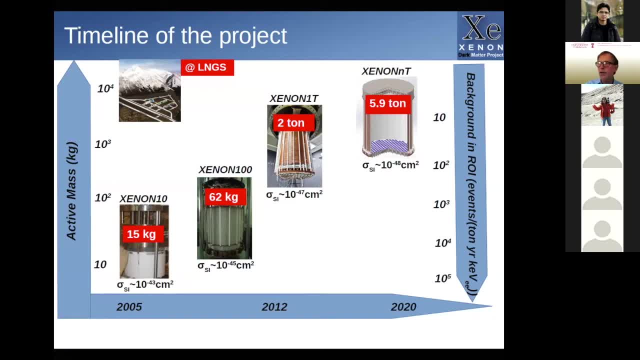 This is fantastic. If you run a kilogram of detector in your lab at the university, you have a thousand counts per second And they have less than one per year. So this is a huge achievement in sensitivity, And that's what you need. 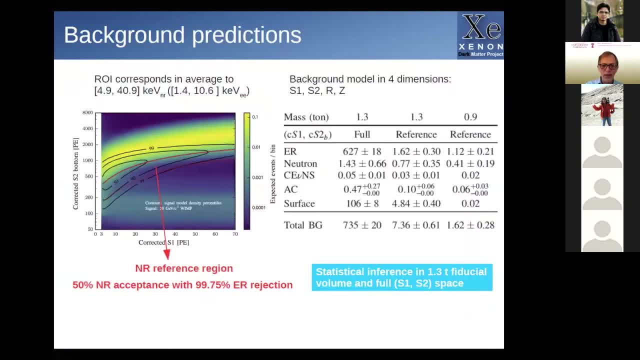 to look for dark matter particles. Okay, what they do? they measure a while and then they have this plane of the ratio of these two signals and the nuclear recoil energy. They have a region where they expect background and they have a region. 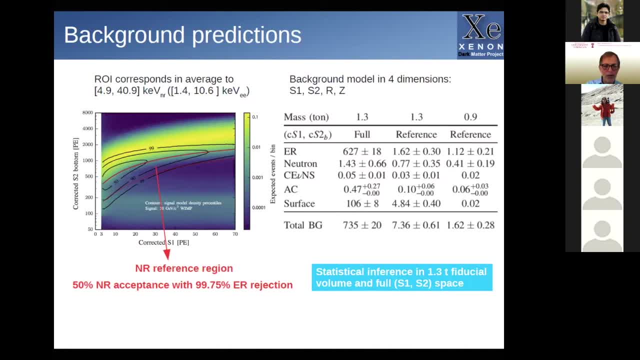 where they expect the WIMPs. These are these black lines, these black contours and these yellow issues where they expect the background. Then they can study. what backgrounds do they expect? They expect electronic recoils, They expect neutrons, also neutrons. 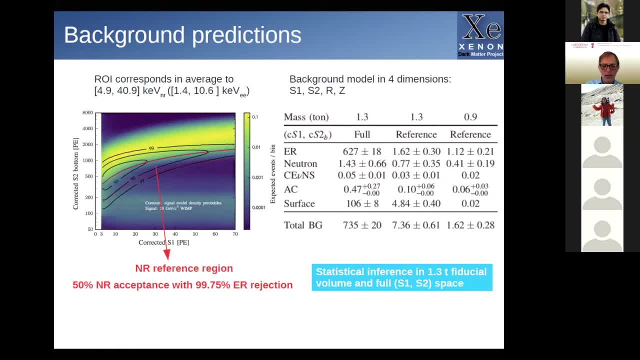 so radioactivity in the surrounding laboratory wall produces neutrons. They expect neutrinos from the sun. The solar neutrinos also can scatter in these detectors And maybe in 10 years from now this will be a background. Today it's still. 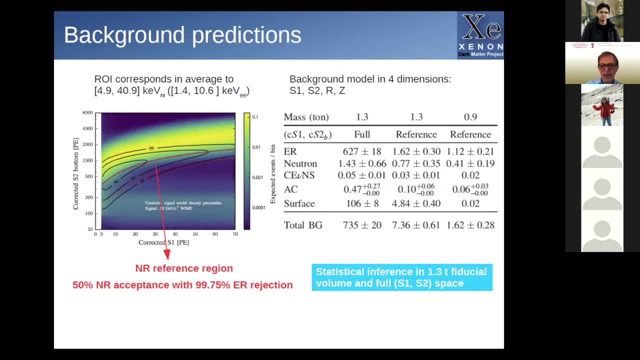 So here do you see the numbers they expect. They expect very low numbers, so less than one count. But from electron recoils they expect something, and these different columns here is if they use the full detector or if they do a cut in the positioning. 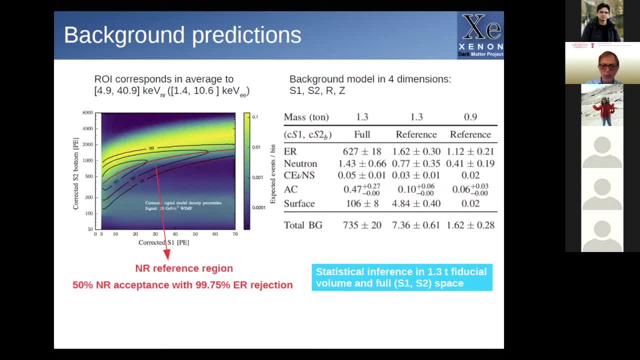 So if you cut away the surfaces, most of the background, the electron recoils mainly come from the surface of the detector. They come from outside into the tank. So you see, if you take the full tank they have this number. 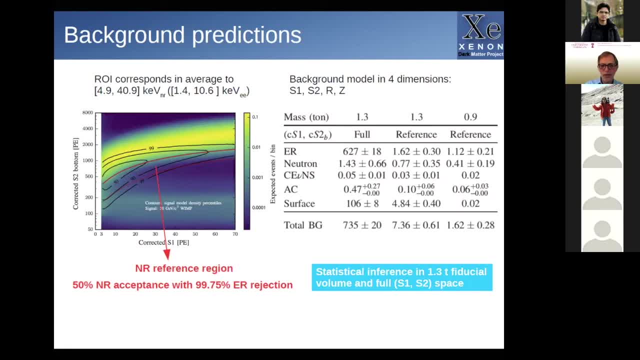 But if they cut and take a smaller radius, they can do that because they have this 3D position resolution, and so the number goes much, much lower. The number goes much, much down, Okay, and from the expectations, how these backgrounds are distributed and so on. 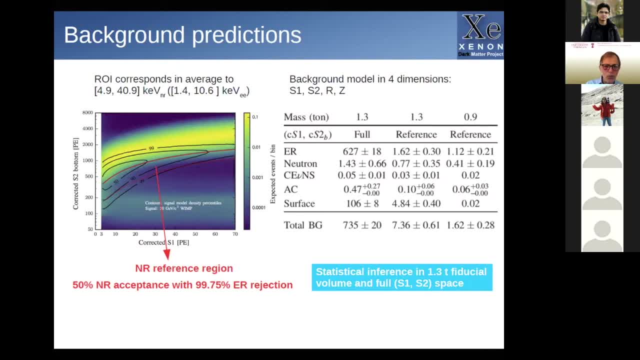 they do a likelihood analysis where they have the best chances to see a WIMPS versus the background, and then they define a region of interest in this plot. So these are these two red lines here. Sorry, you do not see it. I use my pointer. 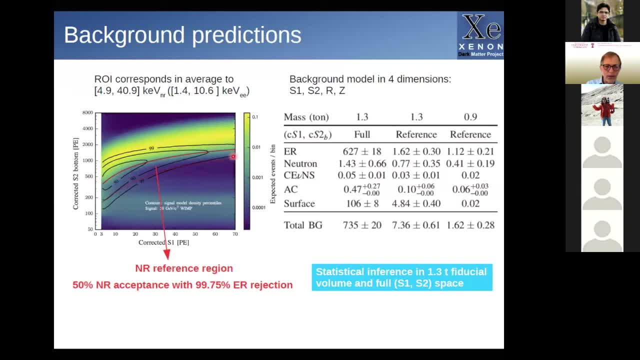 So these are these two red lines here where they expect the WIMPS And these are the backgrounds here. So this is the best region where they expect the WIMPS And what they do. so this is the data. So they expose their one-ton detector. 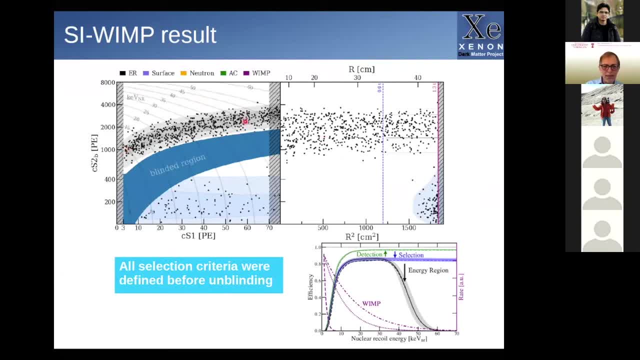 for two years or so And this is the data they get. So this is the data in terms of this ratio of the signals and the energy And this is the 3D position resolution. And you see these electron recoils here. They are distributed all over the detector. 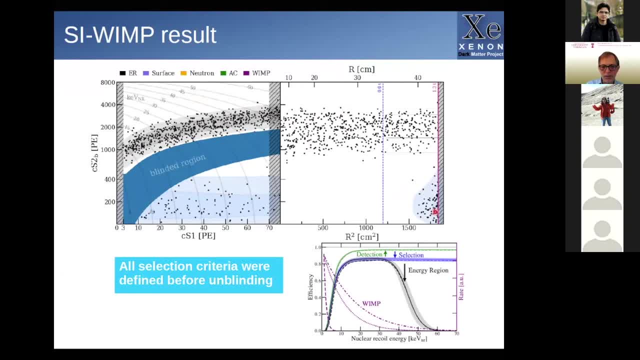 These low energy events here they come from the surface, So if they do a cut, they get rid of a lot of the background, And this is the region where they expect the WIMPS And they do a so-called blind analysis. 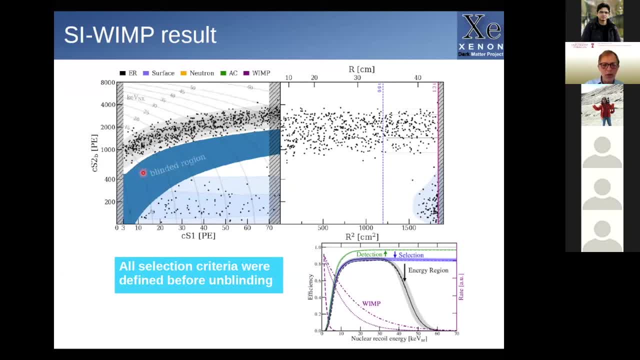 That's state of the art for all of these experiments right now. So your region of interest is blinded while you do the analysis. So nobody in the collaboration sees signals in this region. But one has to define all the procedures, how the data is analyzed. 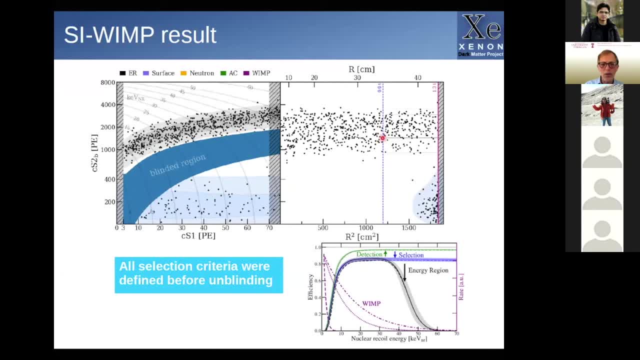 One has to decide where one does the cut in radius, One has to decide when one does cut against noise. And all these selection criteria are defined before you unblind this region, Then you unblind. So this is to avoid a bias. to avoid a bias, to enhance a signal. 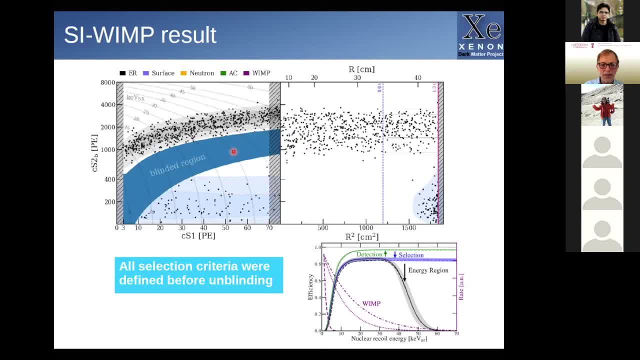 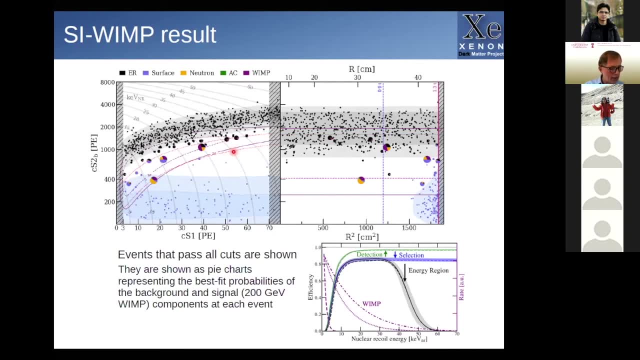 which is not there, for example. So that's why a blind analysis is state of the art right now, And then you unblind and what you find are some counts. So these are these numbers here And from their likelihood, of all the backgrounds. 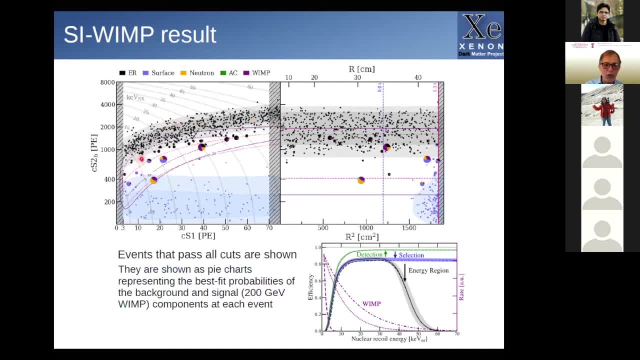 and the likelihood of electron recalls the distribution they have in this plane and the likelihood of WIMPS in this plane. they even can give a likelihood of each count whether it's a WIMP or not. So you see, in each count here 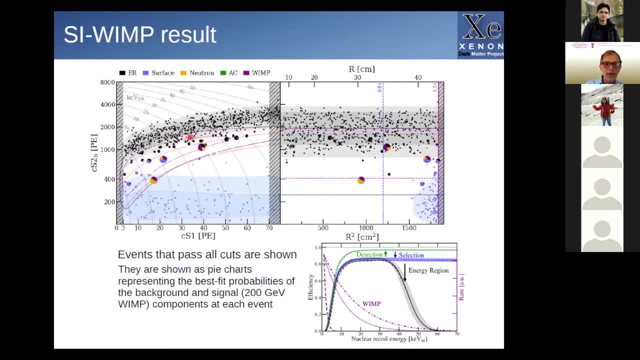 it has a pie chart pattern And this tells you. so this has a highlight likelihood of being a WIMP. This has a higher likelihood coming from the surface and so on. So this, for example, is certainly coming from the surface, So it has a very low likelihood being a WIMP. 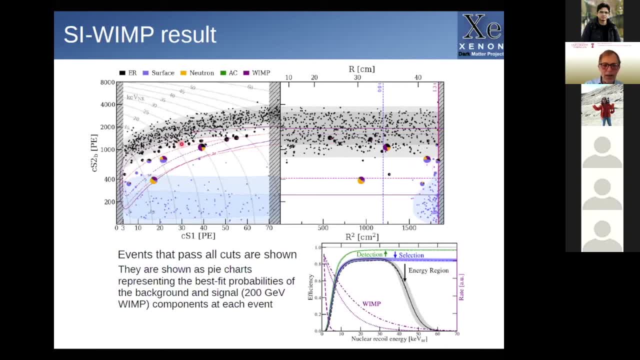 And from all these likelihoods they get. so they have several counts here and they can tell then in the end, okay, maybe maximum five of this could be from WIMPs or so, And this allows them to put limits on the cross sections. 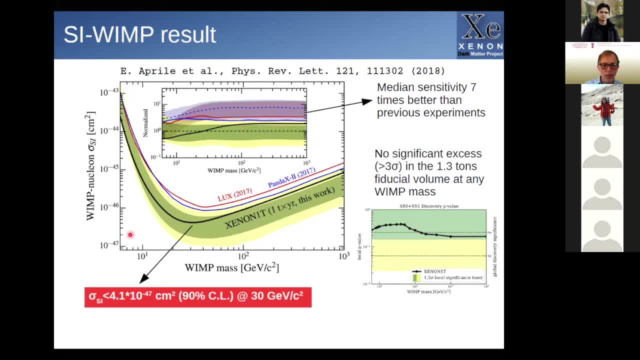 of the WIMPs in the dark matter And this is then the final result they can publish. So this is the axis of the WIMP mass And this is of axis of the interaction strengths between the WIMP and the nucleus. So this is the spin independent cross section. 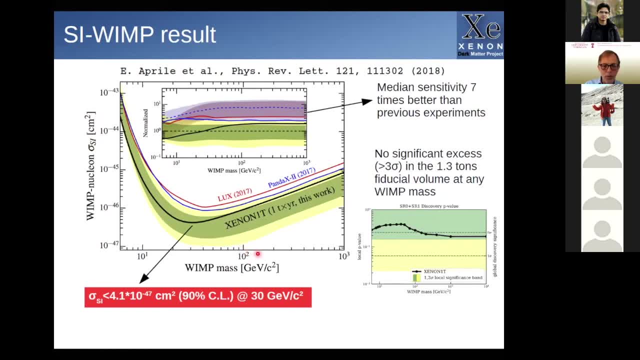 with the nucleus And you pick a certain WIMP mass, let's say 100 GeV, And then you increase the cross section more and more and more, And then at some point you would say, okay, now with this high cross section. 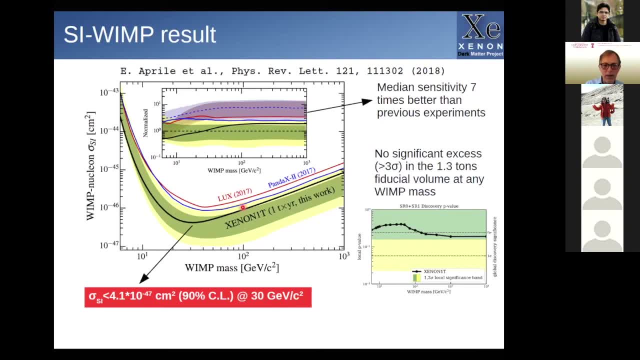 I would see more signals than I have seen in my experiment. That's why you can exclude all the cross sections here. You cannot exclude cross sections below this line And you do that for each WIMP mass And this gives you this line of exclusion. 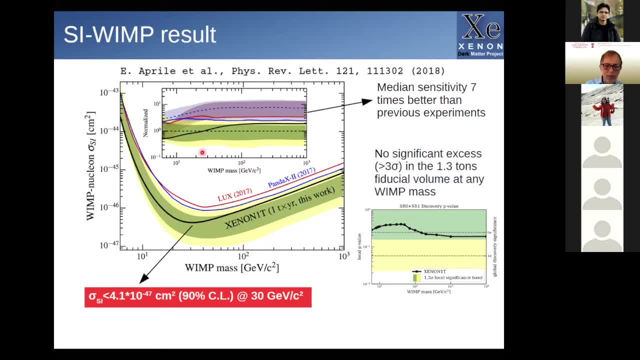 So this is the limit line. Everything above is excluded, Everything below is allowed. So this is then the final result. That's a limit. So none of the experiments yet has found a WIMP, but they give better and better exclusion lines like this: 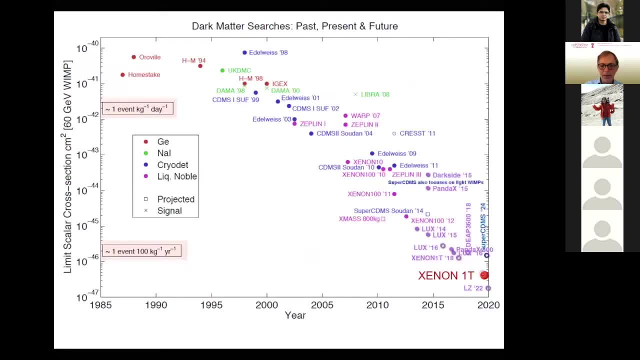 And in this plot I showed before, this puts xenon-1-ton to the top here at the beginning. So this here are projects, So these open circles are all projects, but xenon-1-ton is here with the real data, so with the real result. 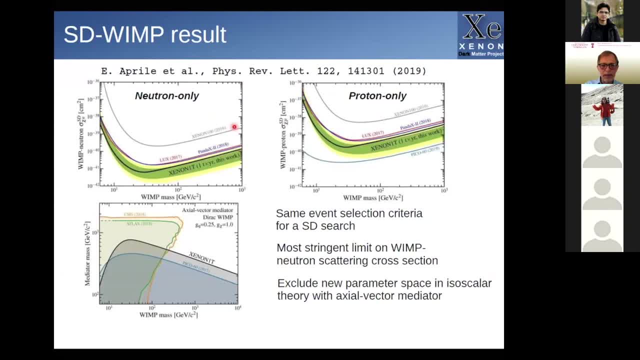 Okay, and, as explained before, they can also do spin dependent analysis. So there, the limit cross section are not yet the numbers are not so good, But you can do this for neutrons, for unpaired neutrons or unpaired protons. 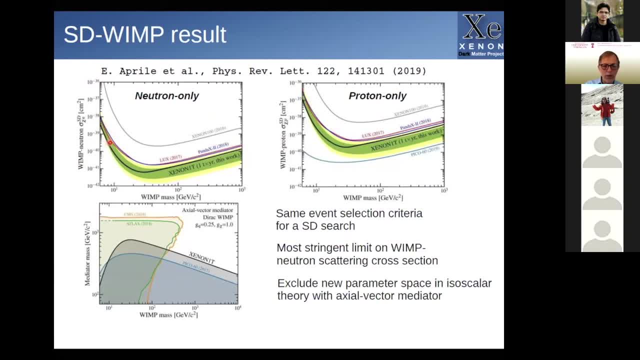 And also there, xenon is world leading and has the best limits. So these are, oh no, not here. In the neutrons only they have the best limits. In protons only the PICO experiment is a little bit better. 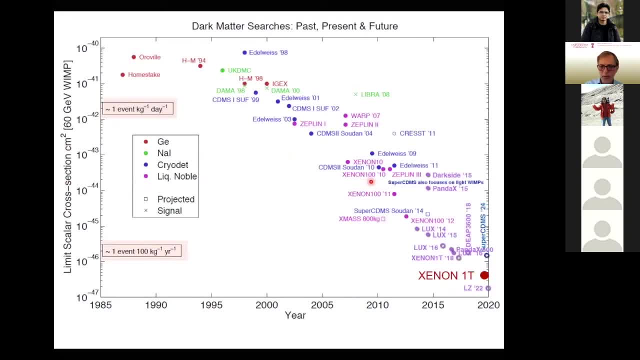 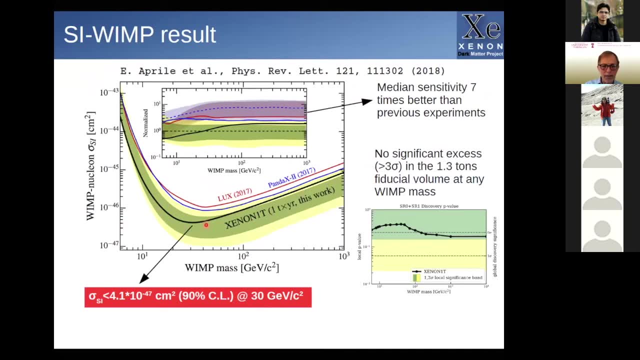 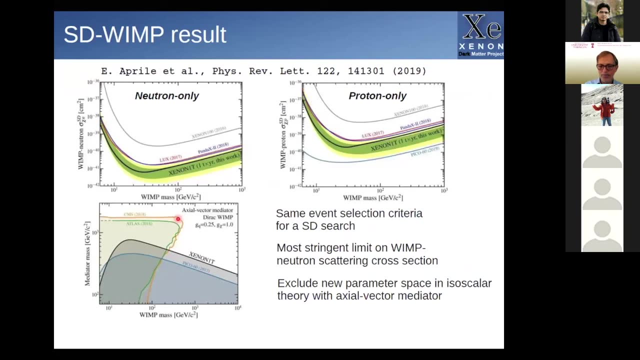 But of course, in this, here in the standard space spin independent analysis, xenon has by far the best limits And given the sensitivity here at this, wimp mass is the world leading sensitivity at the moment. Okay, So what's the future of liquid noble gas detectors? 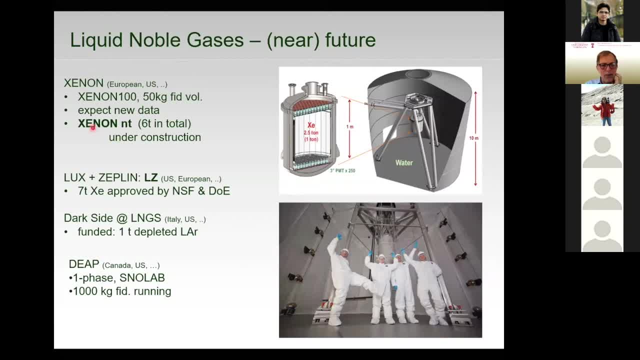 As I said, xenon is setting up a six-ton experiment. It's called xenon-n-ton And it's under construction and will start data taking Very soon. Then there's the LSAT experiment, which is actually a combination of the previous LUX and Zeppelin experiments. 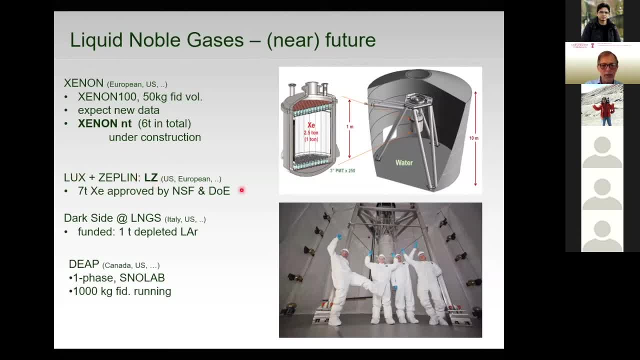 And they have funding for a seven-ton xenon experiment in the US. There's the dark side liquid argon experiment- one ton being set up at Gran Sasso, And there's the one ton liquid argon set up also at SNOLAB. 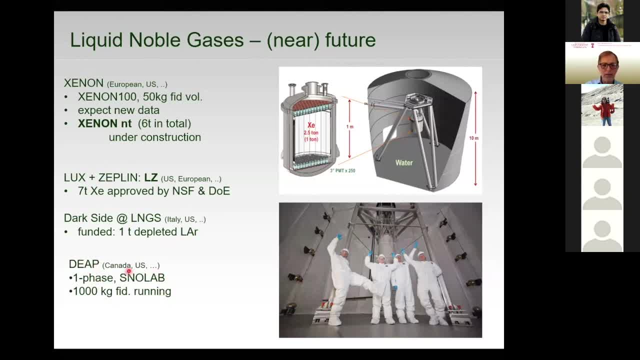 which is mainly Canadian experiment. So there's a lot of activity going on And these are the most promising in the wimp mass region of around 100 GeV. So that's the classical wimp region actually, And that's why these experiments. 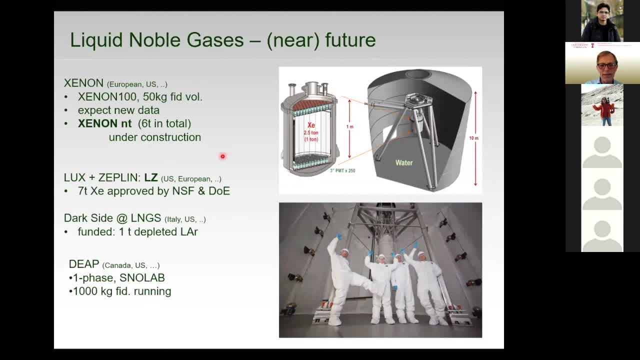 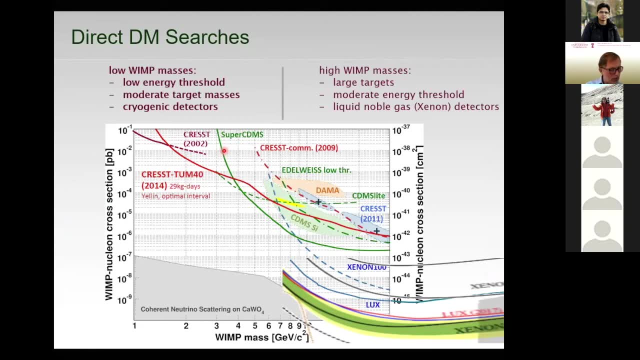 especially the xenon experiment, are the most cited ones at the moment. Okay, Now I'm. I think something went wrong. I'm even faster, Hesti. Okay, So then this is the same plot as before. So this is wimp nucleus. 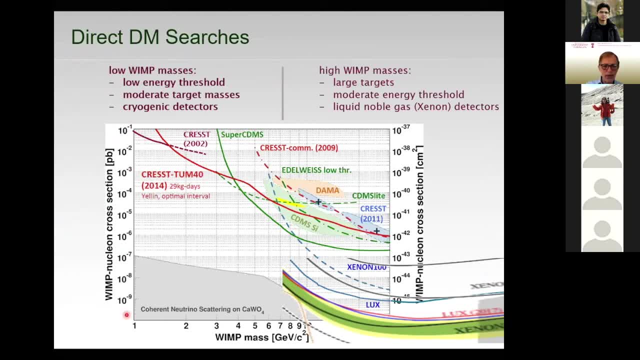 So this is wimp nucleon cross-section And this is wimp mass And. But it's now on a logarithmic scale. So that's why the xenon limit here is only in this corner here And you see all the experiment before. 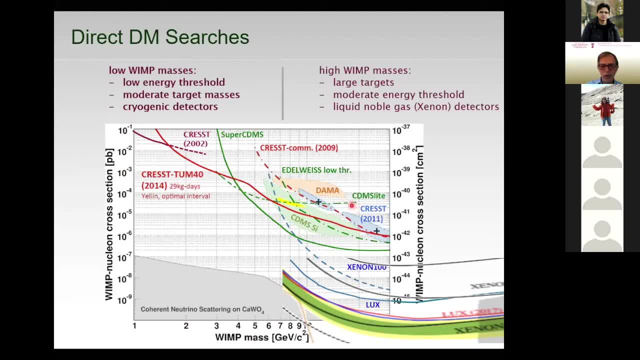 So you see how, What a huge progress was done, orders of magnitude So at the beginning. so this is where the CDMS experiments- at the time it was the best one. Then the xenon experiments came up, putting this line, this line, this line. 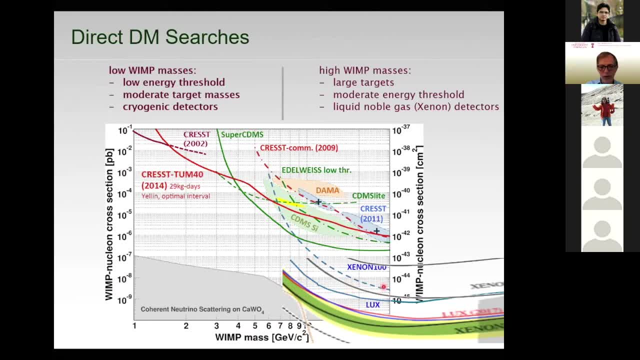 So over the years in this region above 10 GeV there was a lot of progress being made And it's led by the liquid noble gas experiments. But if there's also growing interest in low mass wimps, so at lower and below 10 GeV. 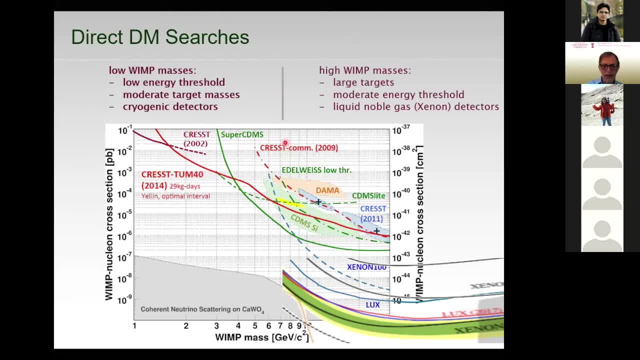 And This is There you need, as I will show you, you need a lower and lower energy threshold, And this is still the domain mainly of cryogenic detectors. You see experiments here like super CDMS, and you see the CREST experiments. 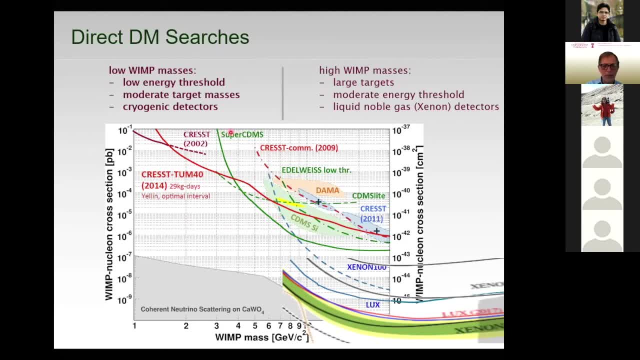 And I will tell you in the next section about these experiments, about the cryogenic experiments, And at, let's say, 10 years ago, they were leading the field. They were then overtaken by the liquid xenon experiments in the high mass region. 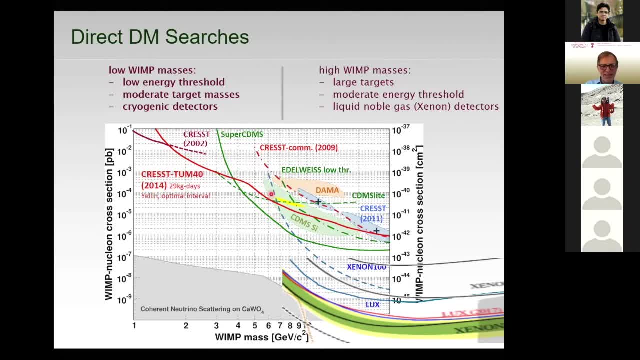 but they are now left, put to the corner, let's say here to the low mass wimp region. And the interesting thing is this low mass wimp region also. it was absolutely unfashionable at the times when one believed in supersymmetry. Because from the accelerator one was assuming the wimp mass should be higher and higher. because the accelerators went up in energy, didn't find anything, so the wimp mass went higher And 20 years ago nobody believed that the wimp can be lighter. 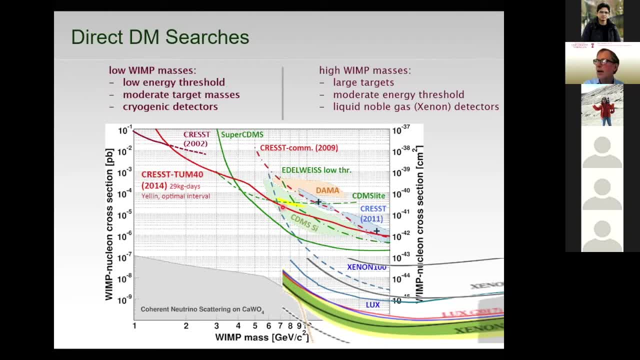 than, let's say, 50 GeV. But after LHC looking for supersymmetry, not finding anything, the ideas about One has to develop newer and newer ideas on the dark matter properties And actually there were new ideas coming for low mass wimps. 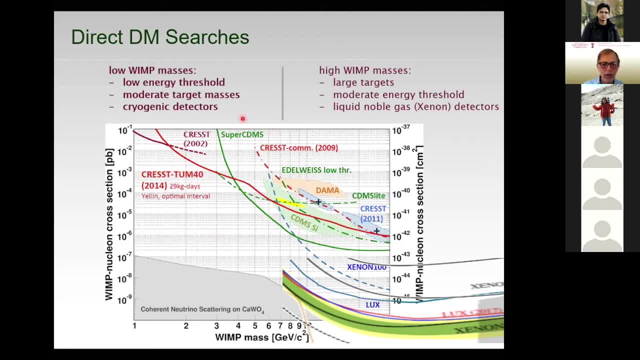 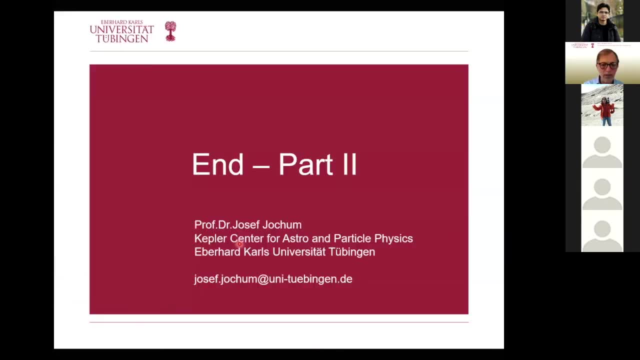 And I will explain that a little bit to give a motivation why we look for low mass wimps and then explain how these cryogenic detectors work. Okay, actually I'm at the end of part two. right now We could do a questionnaire section. 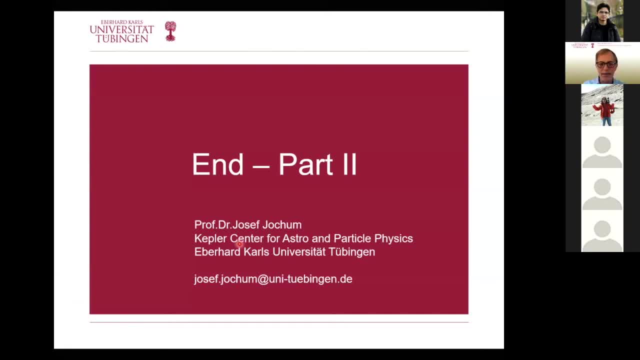 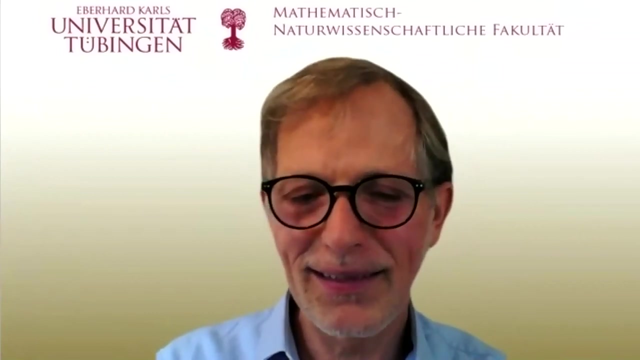 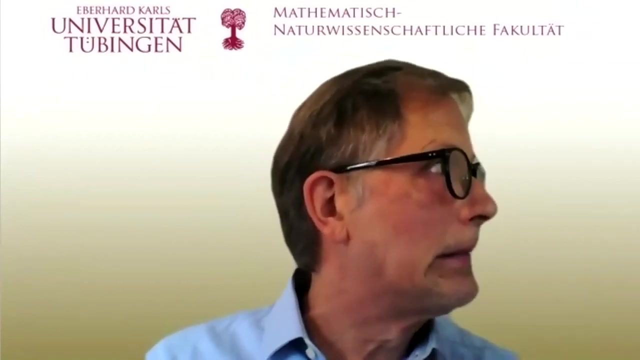 or I could continue for a few minutes. Hestie, that's up to you to decide. Okay, We still have Two questions here. Maybe I'll ask: Let's see. Oops, Wait, Is it STC? So maybe the first question. 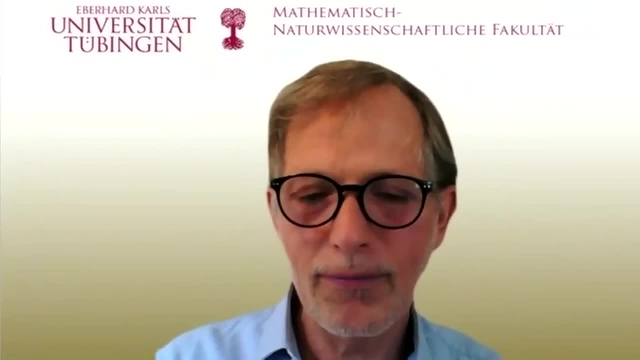 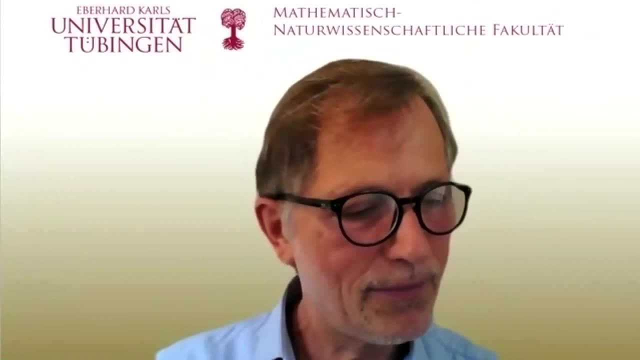 From Hasan Zaki. Hello, Can you hear me? Yes, Hello, You want to ask your question by yourself? Yeah, I got my question, but I think it's already answered The? Okay, I'm going to refresh, I think. 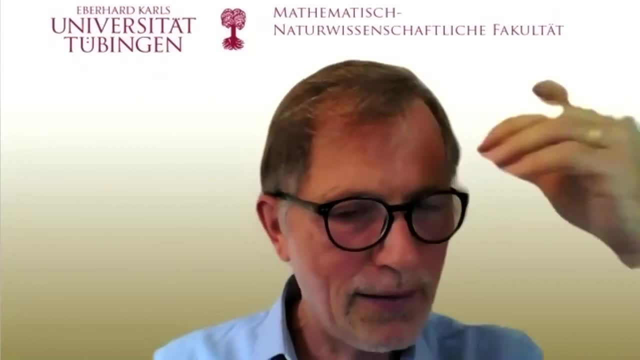 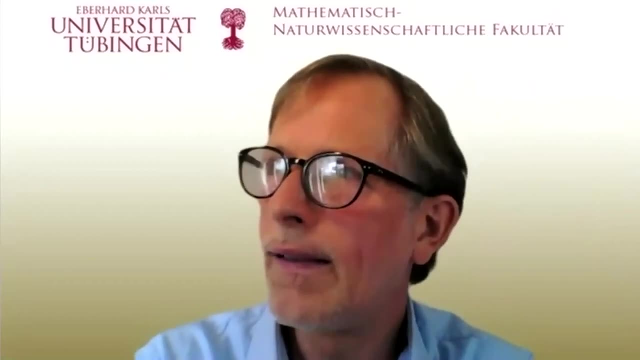 to the question: Is there any megaprojects, such as CERN, LIGO, that try to find dark matter by direct detection right now, Because I'm trying to Maybe try to follow, see the story. what are they doing? 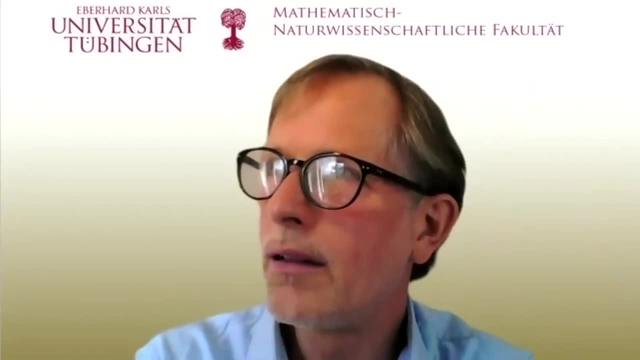 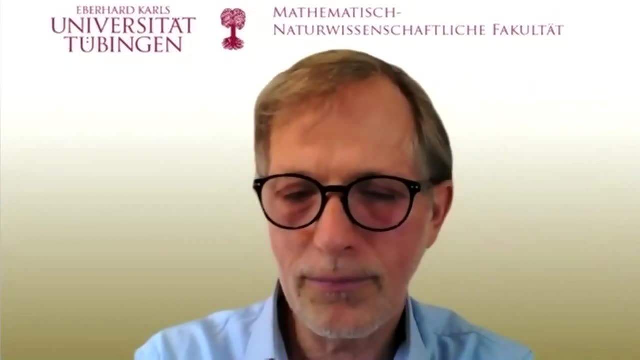 try to find further information about it, But you already said about Xenon and stuff, but maybe, if you want to say it again, it's up to you. Yes, But I think you already answered the question. Yeah, So the biggest projects at the moment are Xenon. 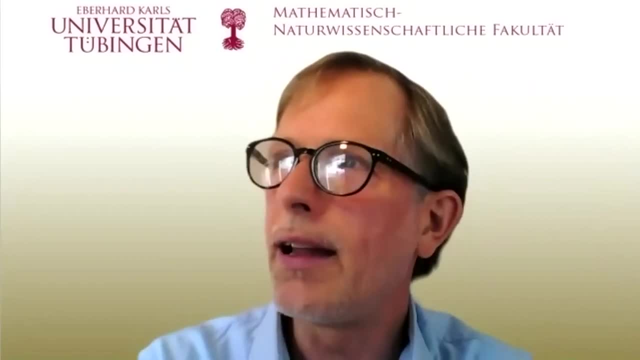 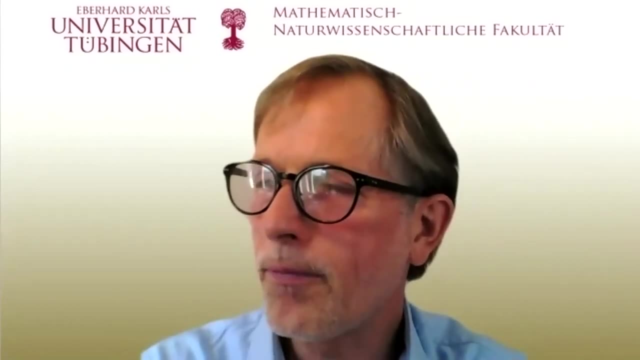 LSAT and DarkSight, And actually there is something beyond which I didn't mention yet. So there are plans. There are plans to put after the next round, so when all the experiments have finished, they are, let's say, 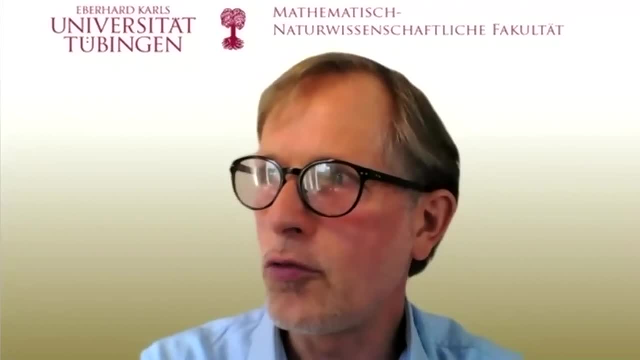 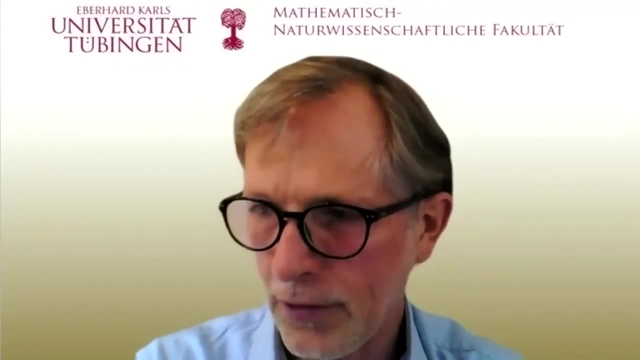 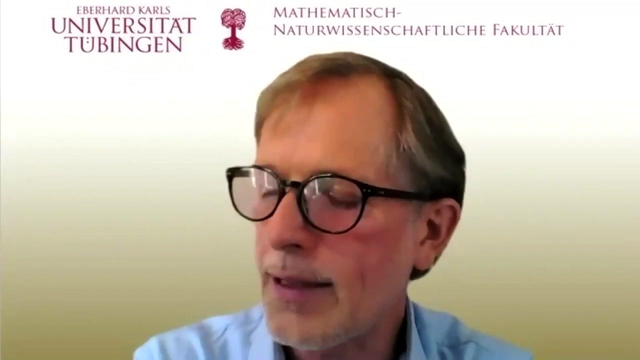 five ton or six ton detectors. there are plans to put all the efforts together, Actually all the experiments would like to combine their forces afterwards to build a huge, let's say several 10 tons, 30 ton detector, And that's called Darwin. 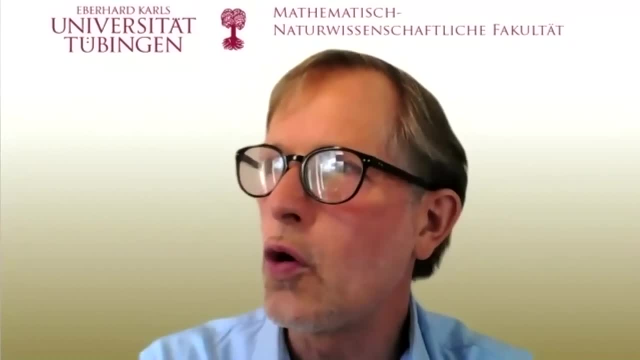 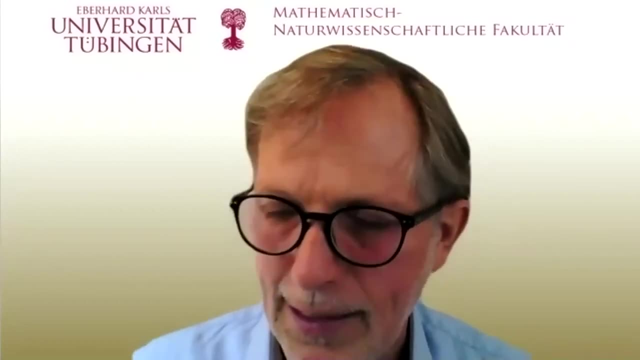 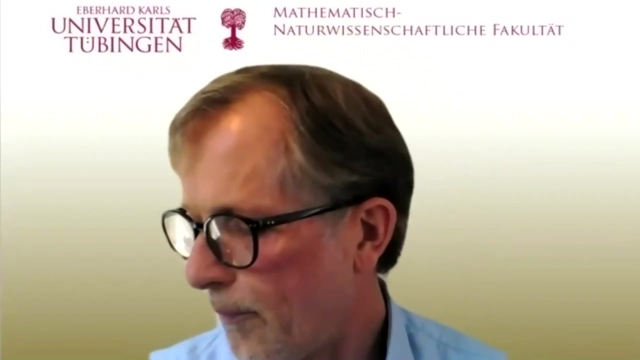 Darwin, Darwin, Yes, If you Google Darwin, dark matter searches. this is still Okay. this is still an idea, It's still in the design phase, but it's being prepared and there's already funding for it. So if you would like to do a career in dark matter searches, 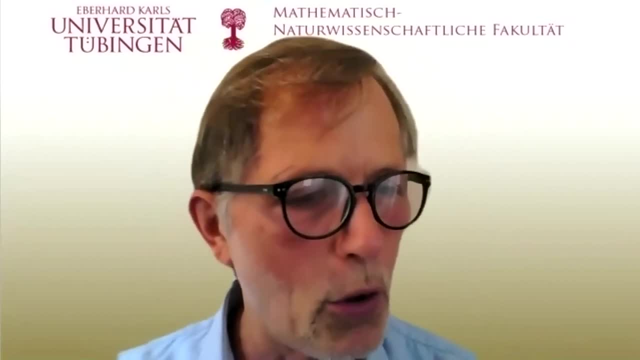 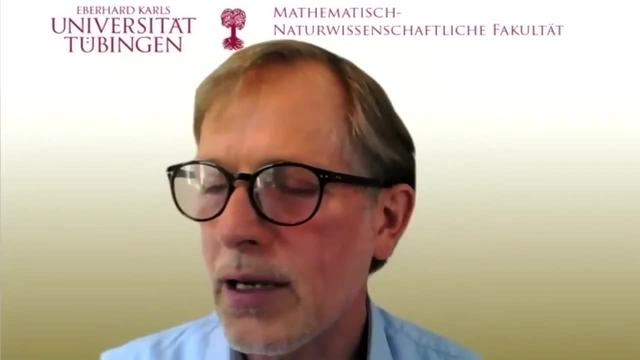 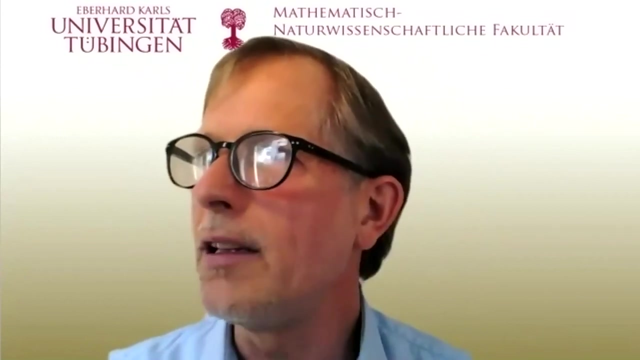 in direct detection. you should probably look to Darwin. Yes, That's good news, Thank you, Yes, And the idea is to go even bigger, Yes, And then to do a 10 ton experiment or a 20 ton experiment, And it's still open if it's xenon. 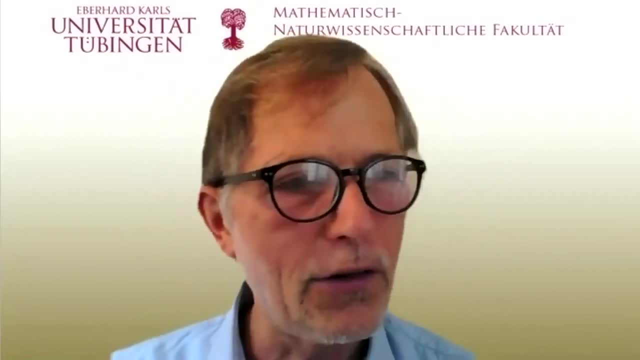 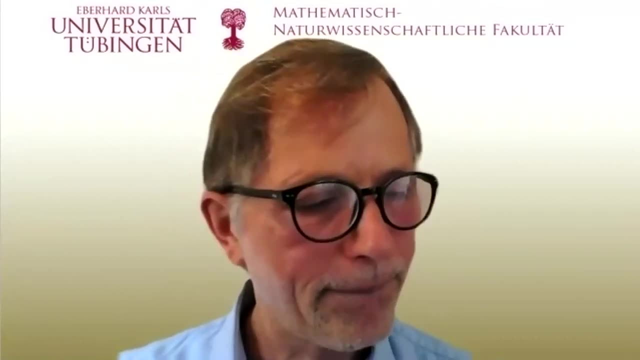 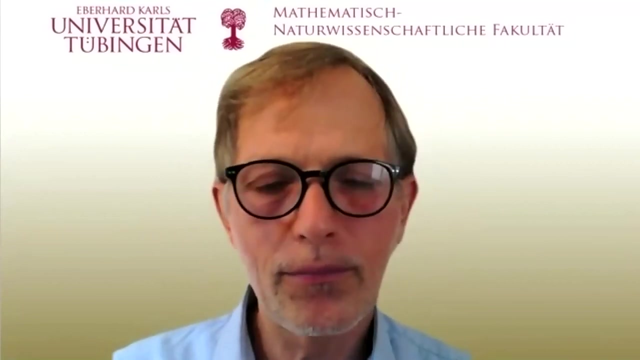 Of course, there are experimental issues between xenon and argon, So this is still open. if it's xenon or argon in the end, Okay. Second question is from Nishal Maharjan. Nishal Maharjan, are you here? 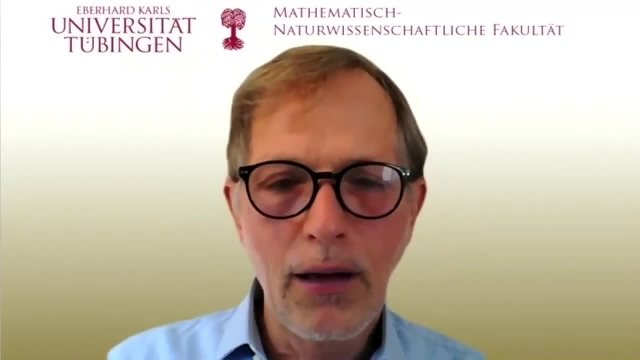 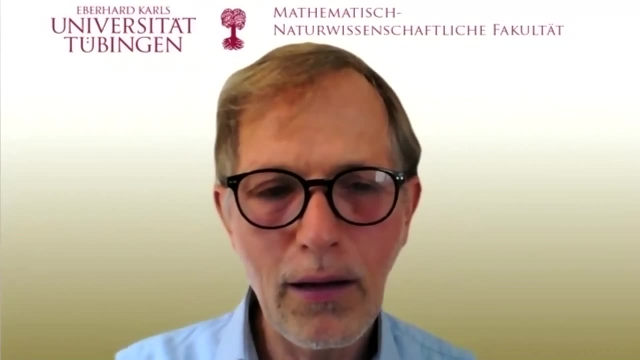 Yes, please. Thank you, Professor, for such a wonderful. So my question is: how confident can we be in the results produced by xenon experiments if we only get few counts per ton per year? What does the statistics look like in such experiments? 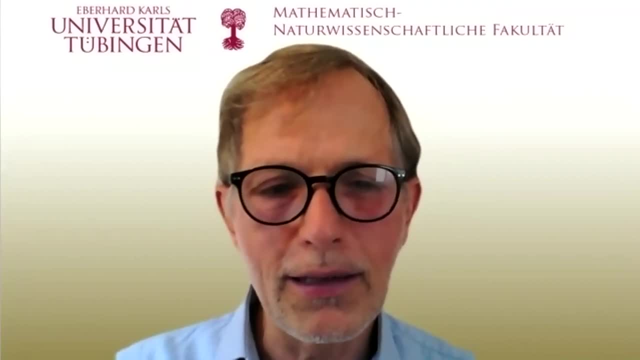 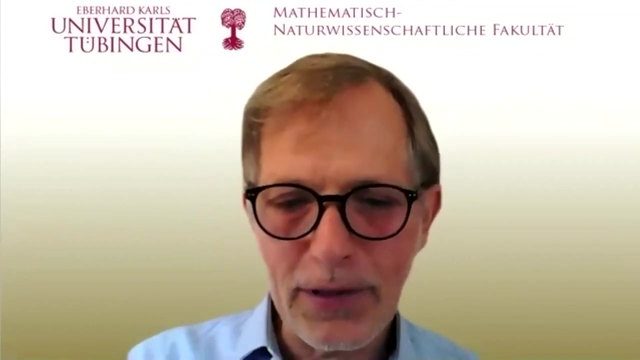 Thank you. Okay, That's an interesting question. So so you ask, how confident can we be if we have only a few counts? So the thing is, maybe I go back. let's let me see. I try to go back a little bit. 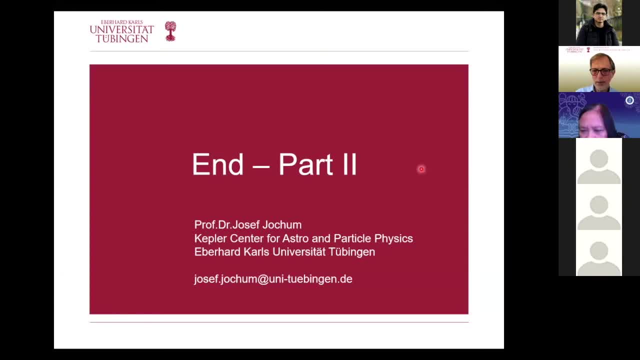 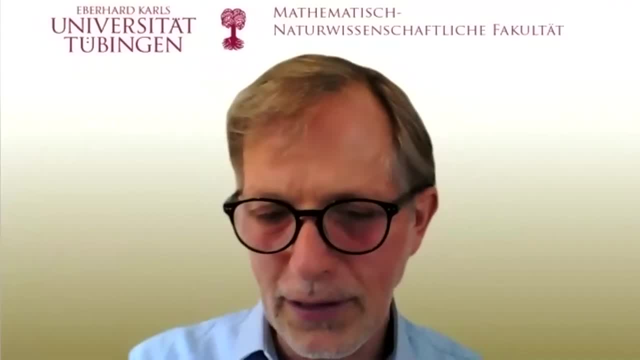 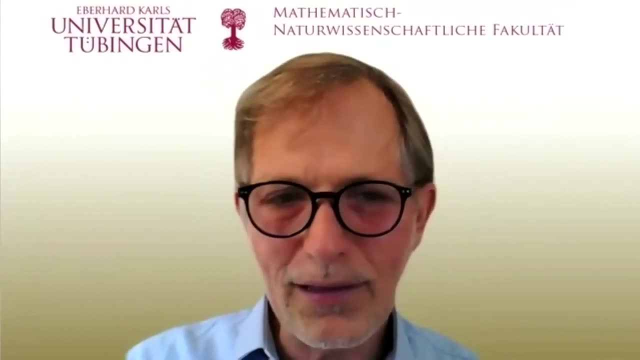 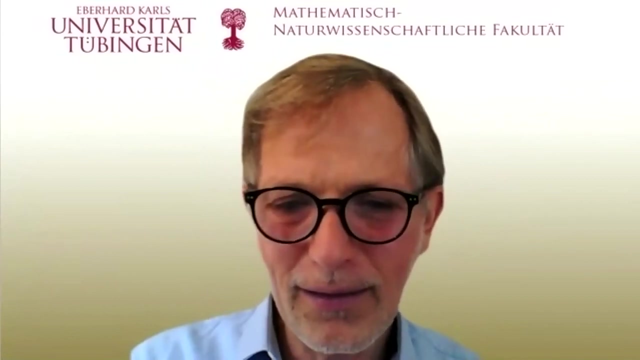 So if I- Okay, sorry, I have a problem here. I cannot Just a second. I have to stop something here. Sorry about that. I am back in a second. Okay, let's see Where are we here. Okay. 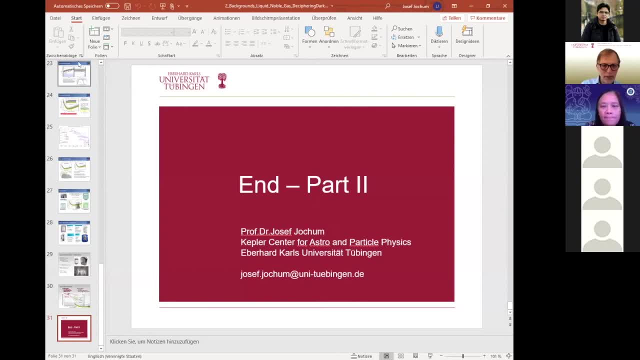 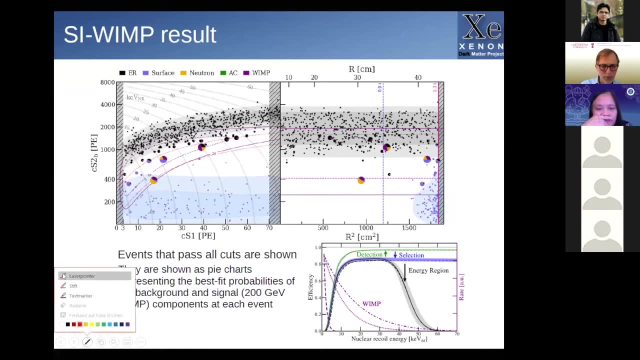 if you look at this picture here. Okay, few, So okay. so this is basically the result of the experiment. This is the ratio of the two signals And this is the energy they measure. And the good thing is, you have counts everywhere here. 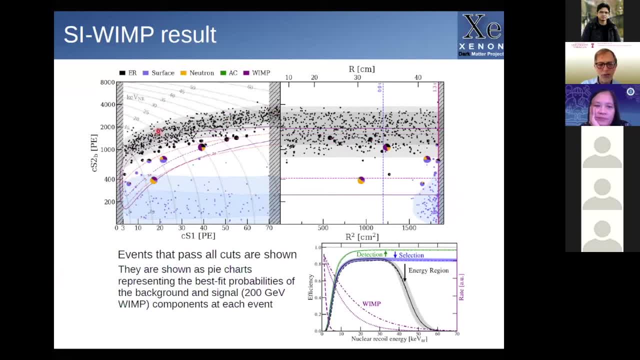 You have counts here. You have counts here. Of course, this is all background. You dislike that, But uh, we have some understanding of this background And actually so. so from the study of the spectrum of this background and the temporal behavior and so on. 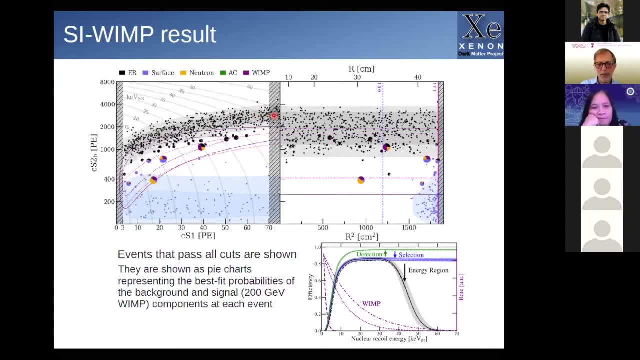 you can compare it to simulations- What you expect from the backgrounds, And from that you can then see: okay, this looks exactly from what you expect. So you expect this distribution in space. You have some problems at the surface, So 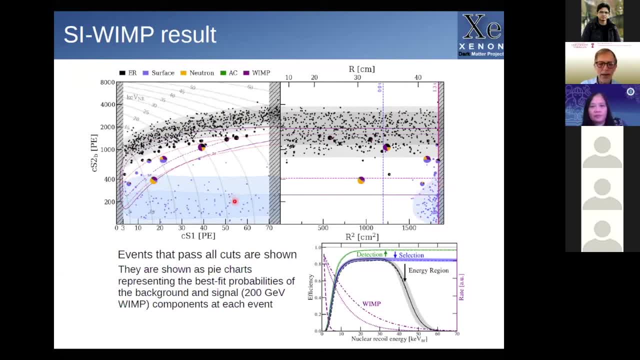 but you expect that And that's here at the surface And an energy is distributed everywhere. So this, this background, it's a nuisance, But it tells you the detector works, It functions, And it tells you you would see a WIMP scatter. 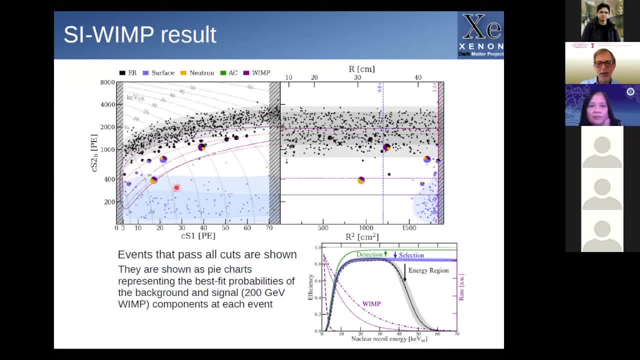 If a WIMP would scatter a nucleus, you would see it, And you would see it in this region. So from this you can be extremely confident. You can not only be confident, you can prove it by experiment In using neutron sources. 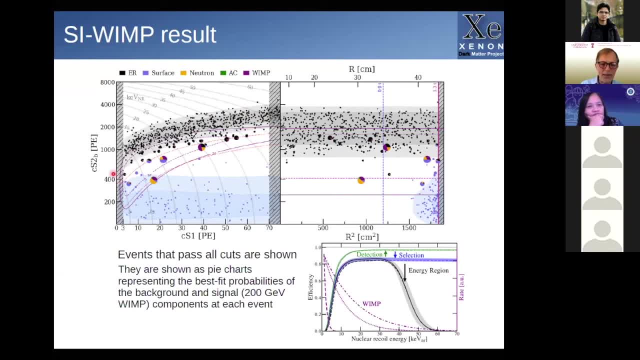 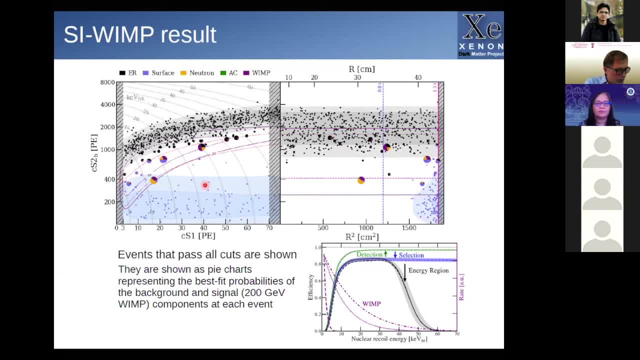 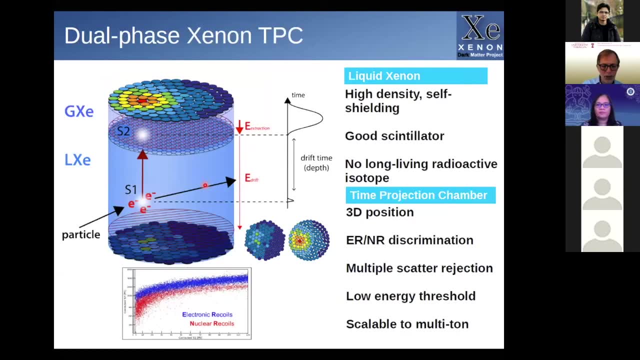 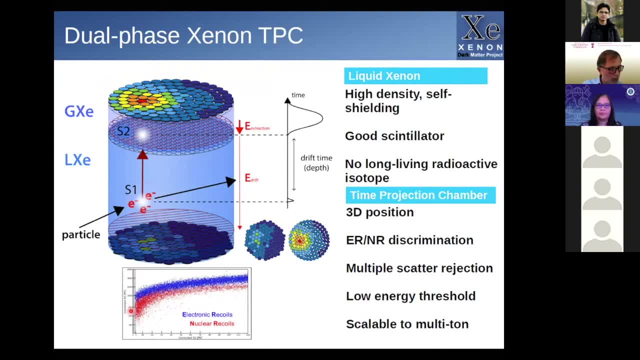 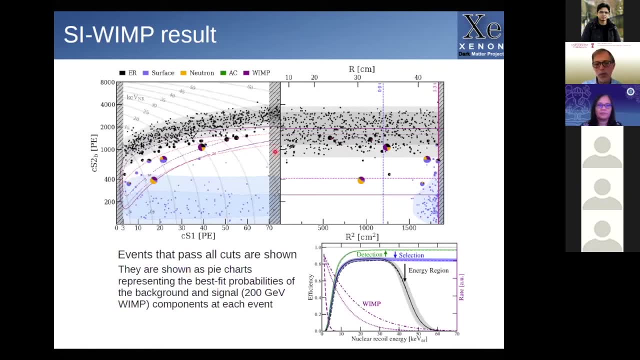 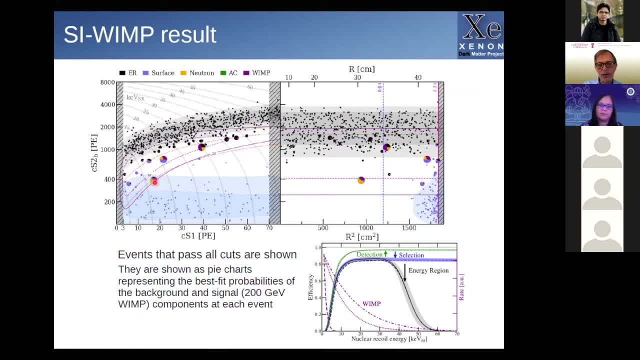 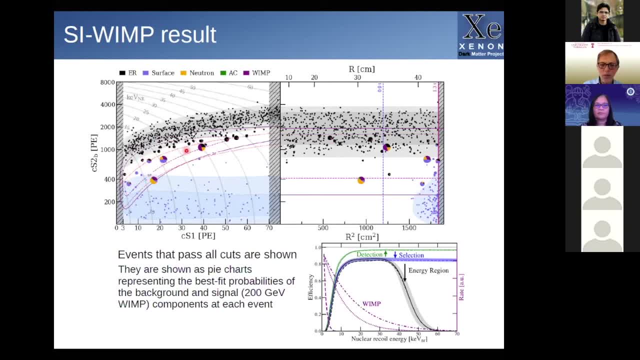 this could be background, but if the WIMP would scatter more and more, it would be. it would show a higher rate. So you can. so if you see five counts, you can exclude that the WIMP does 50, or, yes, that's, you can exclude. 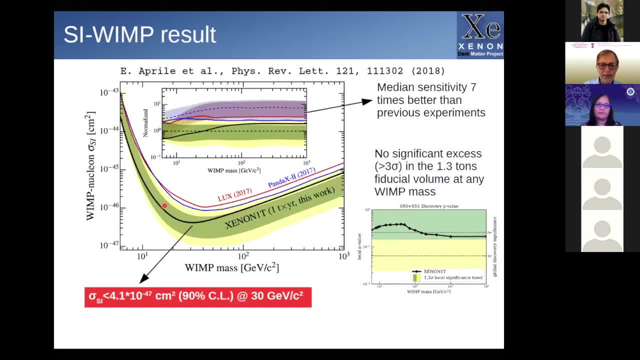 And this gives you then this plot here. So this is the line of confidence where one can say, okay, a WIMP cannot scatter up here, Of course. so in this sense, if your question was: how confident can we be that the WIMP is excluded in this region? 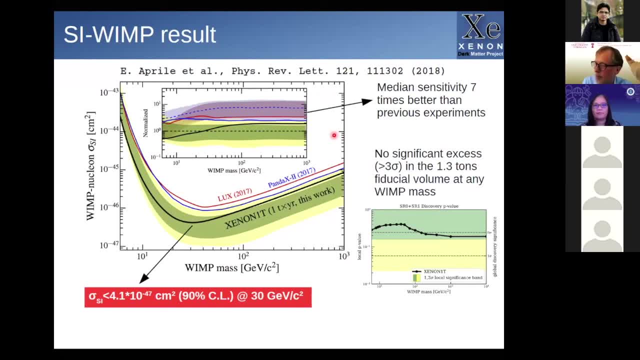 I think we can be very, very confident. I believe that experiment that's carefully done and they can experimentally prove that if a WIMP would scatter more than this, we would see it. The question is, however, restricted to a WIMP with a certain with certain properties. 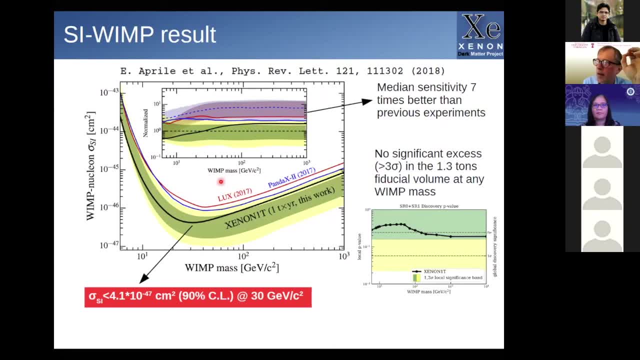 So this is a WIMP which interacts via weak interaction coherently on nuclei. Now, if you now invent another WIMP and you say, okay, my WIMP, my or my dark matter particle does not interact coherently with the nucleus. 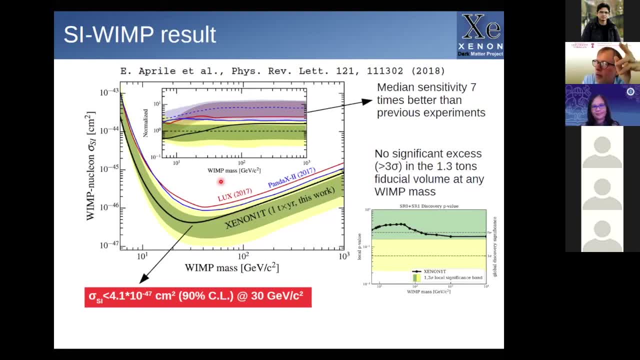 but it only interacts with the electrons in the atomic shell, then this doesn't hold. So all these experiments explore a specific way to do this particle explanation of dark matter and exclude that at present. if they would find something, they could prove it, but since they haven't found anything, they they check this. rip your hypothesis. 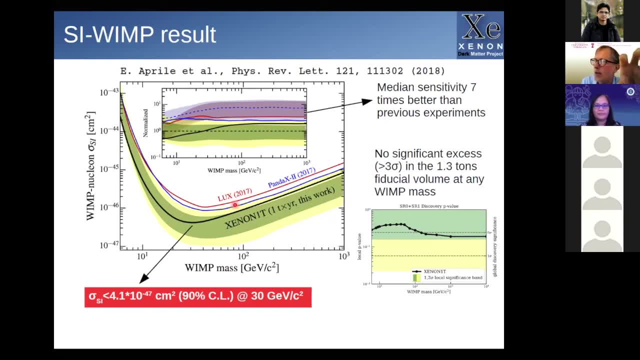 and that's that's. we can be very, very confident and it's actually it's not a disadvantage that they only have this few counts. i think that's a huge, huge challenge that you make a detector such clean that in a ton detector which you run for two years, you would see 10 nuclear recoils. 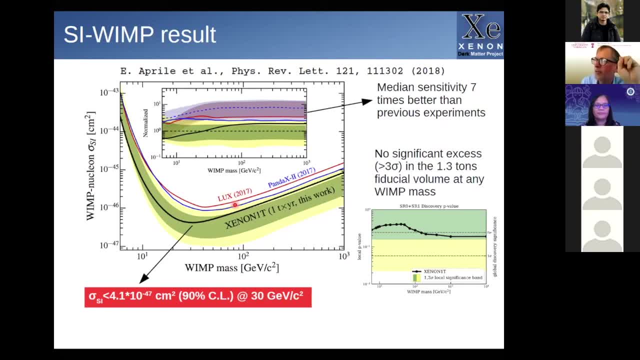 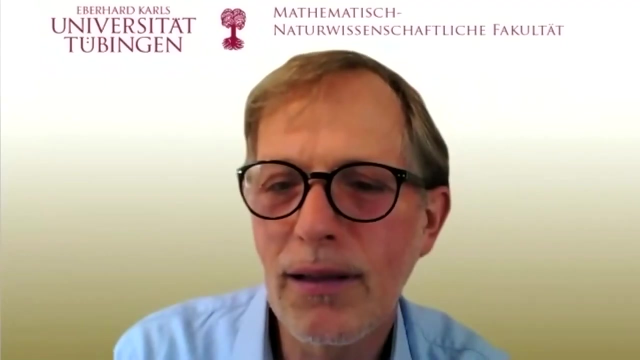 that's an incredible achievement. so, okay, does this answer your question, michelle? that was very good. thank you very much. okay, okay, okay, okay. so uh next is from tanwei shen. so uh next is from tanwei shen. so uh next is from tanwei shen, please. 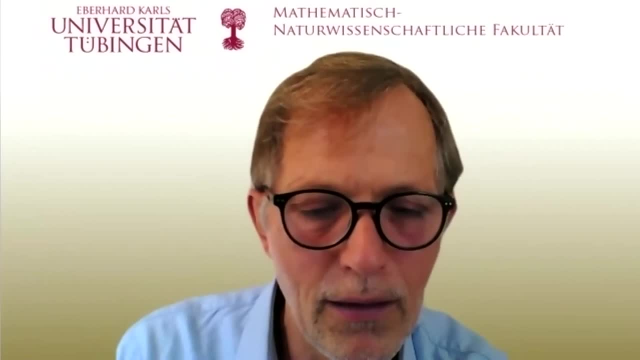 please, please, um okay um. can you explain how is the um um okay um. can you explain how is the um um okay um? can you explain how is the um experiment process inside the detector experiment process inside the detector experiment process inside the detector, for example? for example: 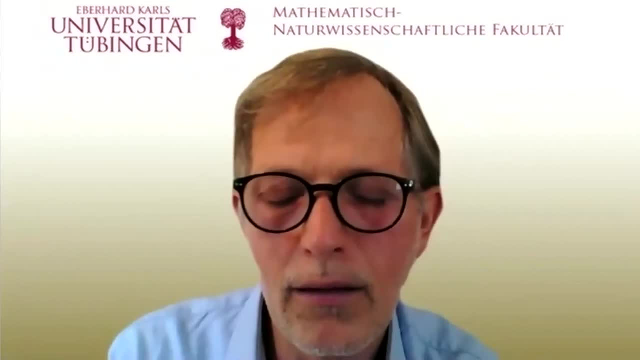 for example, signal or any detector signal or any detector signal or any detector. so i did not fully understand what you. so i did not fully understand what you. so i did not fully understand what you asked. so you asked for the physics. asked, so you asked for the physics. 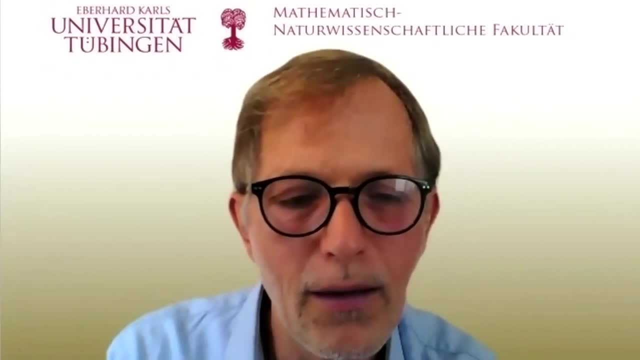 asked. so you asked for the physics process in the detector process in the detector process, in the detector. yeah, how is the experiment process? yeah, how is the experiment process? yeah, how is the experiment process for the in the, for the in the detector, for the in the detector? 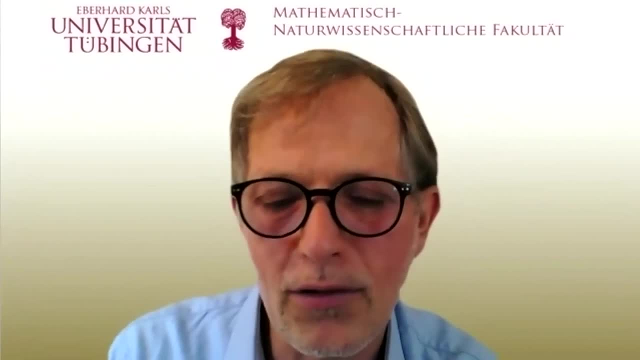 uh, the experiment. so do you mean the? uh, the experiment? so do you mean the? uh, the experiment. so do you mean the physics process? so i, i could understand physics process. so i, i could understand physics process, so i, i could understand your question two ways. so your question two ways. so 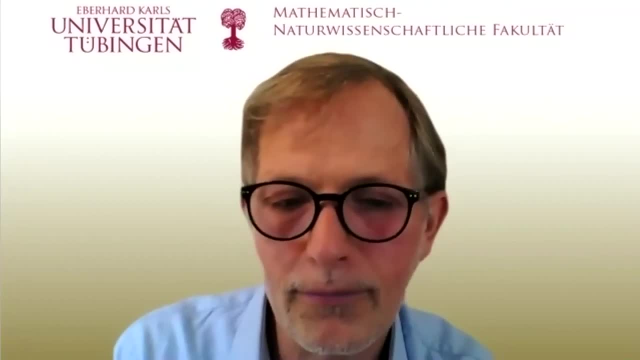 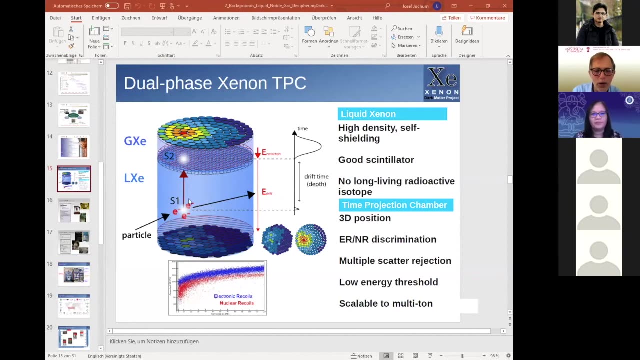 your question two ways. so one is: let me see, so, so, so, whoops, whoops, whoops. you see, this is the detector again you. you see, this is the detector again you. you see, this is the detector again. you ask me what, ask me what, ask me what. okay, do you see my mouse? so you ask me. 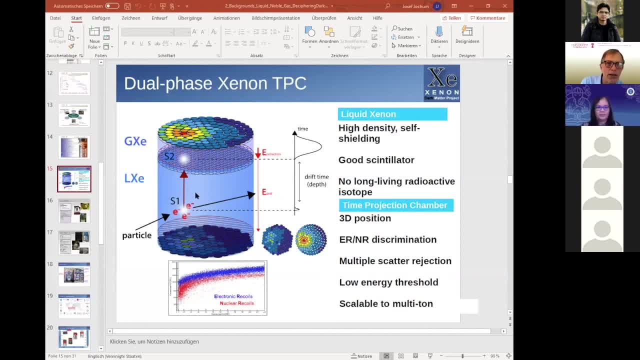 okay, do you see my mouse? so you ask me: okay, do you see my mouse? so you ask me: what happens here? what happens here? what happens here in physics or physics wise in physics or physics wise in physics or physics wise? or you ask me what the physicists do. 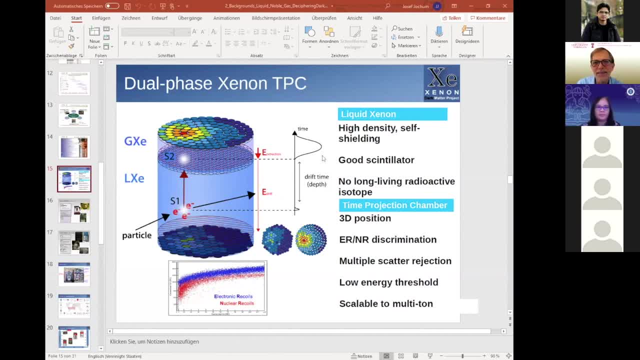 or you ask me what the physicists do, or you ask me what the physicists do with the signals. the first one, the first one. okay, the first one, the first one, okay, the first one, the first one, okay, okay. the first one is okay, basically what. okay, the first one is okay, basically what. 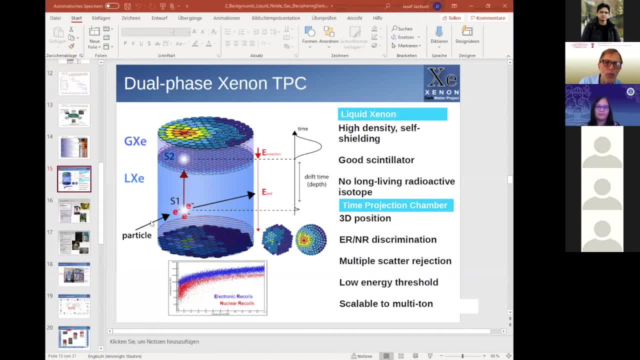 okay, the first one is okay. basically, what happens? you have a particle coming happens. you have a particle coming happens. you have a particle coming in, in, in assume, make it simple. assume it's a assume, make it simple, assume it's a assume, make it simple, assume it's a photon. 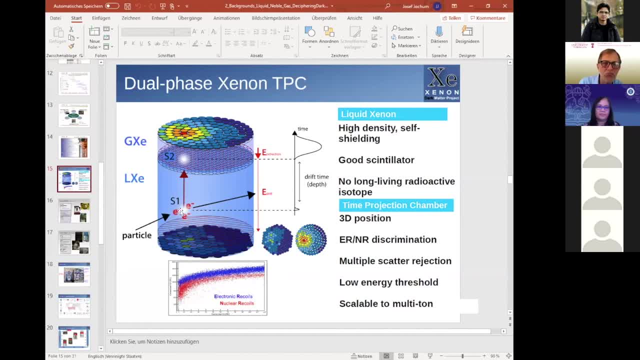 photon, photon. yes, this photon does. yes, this photon does. yes, this photon does photo effect, or most likely a photo effect, or most likely a photo effect, or most likely a compound scatter in the liquid xenon. compound scatter in the liquid xenon. compound scatter in the liquid xenon. so you have a high energy electron. 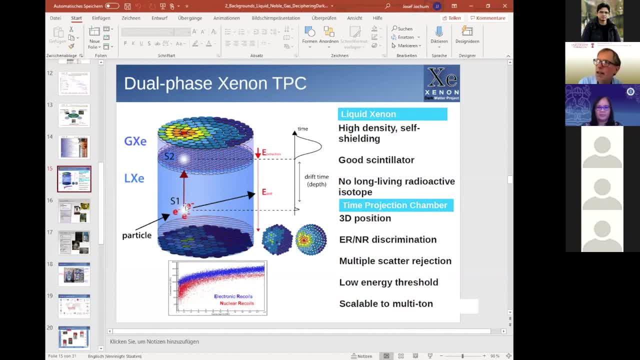 so you have a high energy electron. so you have a high energy electron, suddenly, suddenly, suddenly so you have an electron, which then so you have an electron, which then so you have an electron which then ionizes the liquid xenon, ionizes the liquid xenon, ionizes the liquid xenon. right, you have a track of the electron a. 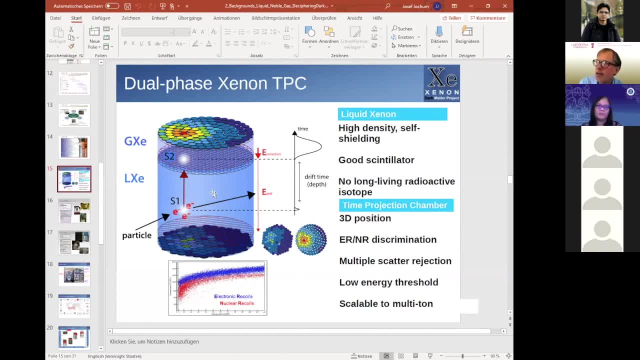 right, you have a track of the electron. a right, you have a track of the electron, a short track, a few micrometers. short track, a few micrometers, short track, a few micrometers. and along this track you ionize the. and along this track you ionize the. 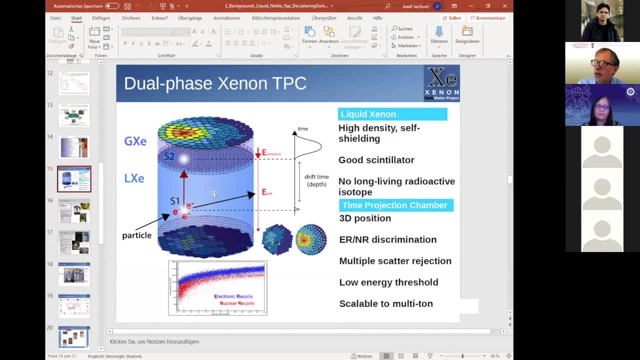 and along this track you ionize the liquid, so you have positive liquid, so you have positive liquid, so you have positive ions and negative electrons, then ions and negative electrons, then ions and negative electrons, then separated, separated, separated, and now a part of these electrons, and now a part of these electrons. 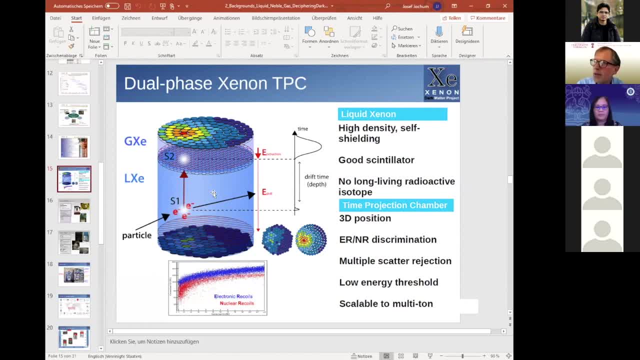 and now a part of these electrons relaxes back, relaxes back, relaxes back. so recombines with the. so recombines with the, so recombines with the. with the xenon under the emission of. with the xenon under the emission of. with the xenon under the emission of light. 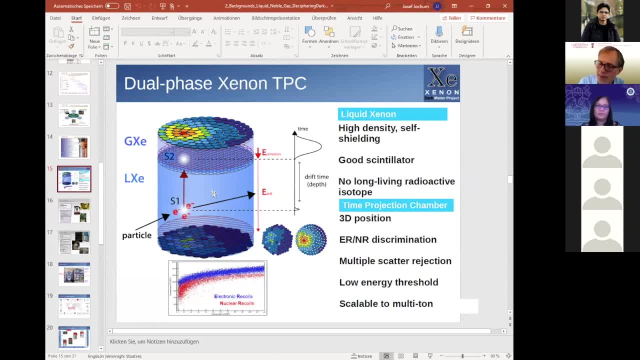 light, light, so, uh, so, uh, so, uh, it and it, but it takes a while. so this, it and it, but it takes a while. so this, it and it, but it takes a while. so this, this energy is the electrons. this, this energy is the electrons. this, this energy is the electrons, this, this ionization electrons which are created. 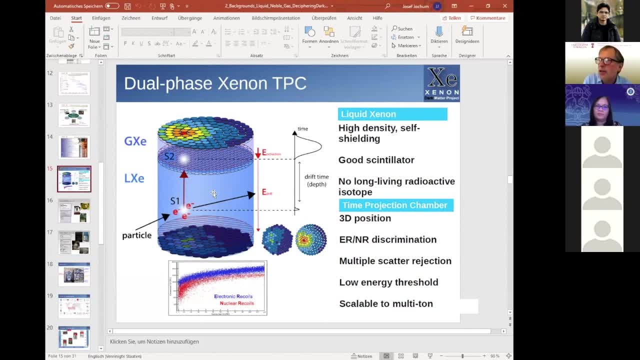 this ionization electrons which are created, this ionization electrons which are created have quite a high energy. they have a have quite a high energy. they have a have quite a high energy. they have a hundred ev or so hundred ev or so hundred ev or so, far away from atomic binding energies. 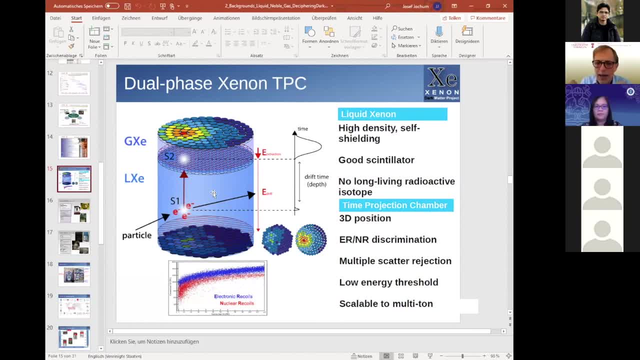 far away from atomic binding energies, far away from atomic binding energies. so they need to relax down in energy. so they need to relax down in energy. so they need to relax down in energy producing another electrons. so there's a producing another electrons, so there's a producing another electrons. so there's a whole cloud of electrons being produced. 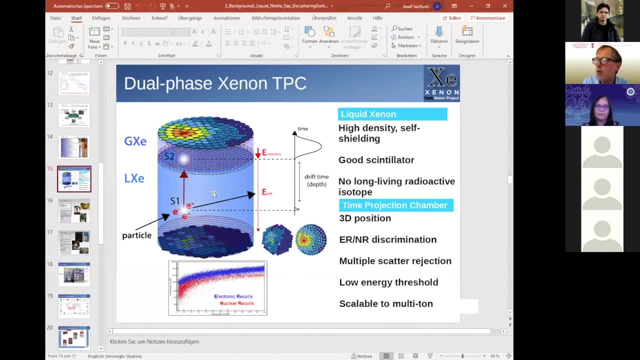 whole cloud of electrons being produced, whole cloud of electrons being produced and part of these electrons recombine and part of these electrons recombine and part of these electrons recombine again with the positive ions producing again with the positive ions producing again with the positive ions producing light. 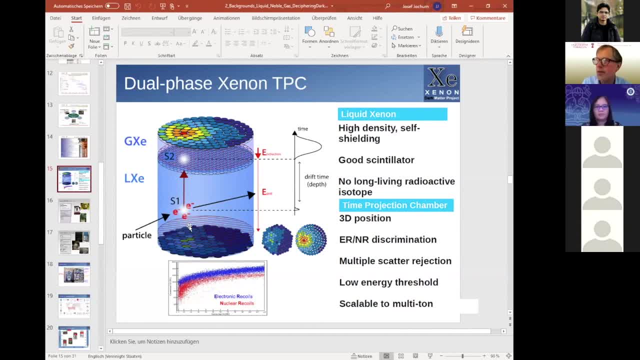 light, light so, and this light is emitted and this so, and this light is emitted and this so, and this light is emitted and this actually has a certain frequency. this is actually has a certain frequency. this is actually has a certain frequency. this is characteristic light of xenon, which you 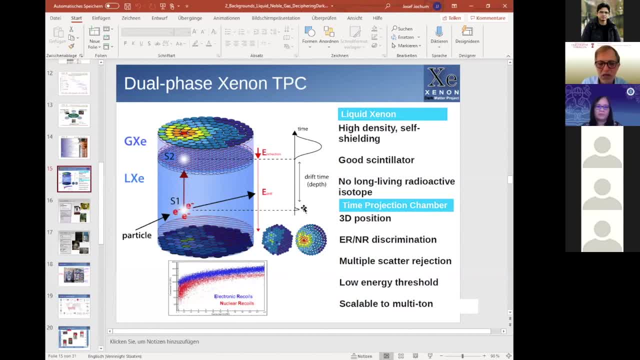 characteristic light of xenon, which you characteristic light of xenon which you then see in the phototubes, then see in the phototubes, then see in the phototubes. so you could even say this light needs. so you could even say this light needs. 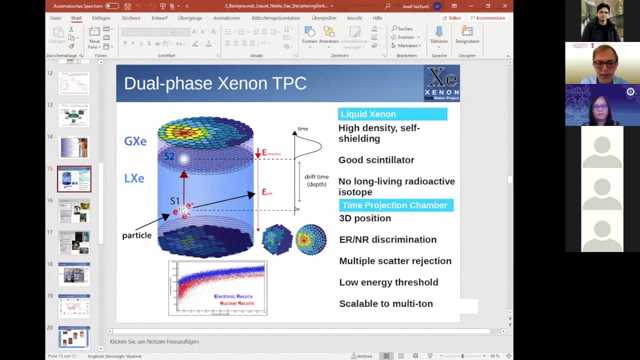 so you could even say this light needs to have a certain wavelength, to have a certain wavelength, to have a certain wavelength, otherwise it's not from the signal, so otherwise it's not from the signal, so otherwise it's not from the signal. so this is one thing. what happens. 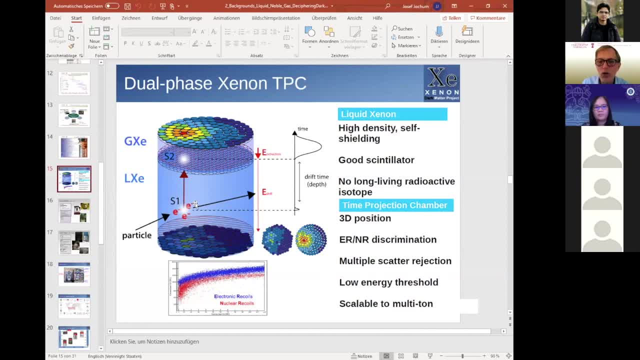 this is one thing, what happens. this is one thing, what happens. but there is a part of the charges, but there is a part of the charges, but there is a part of the charges which do not recombine, which do not recombine, which do not recombine and they or which take longer to. 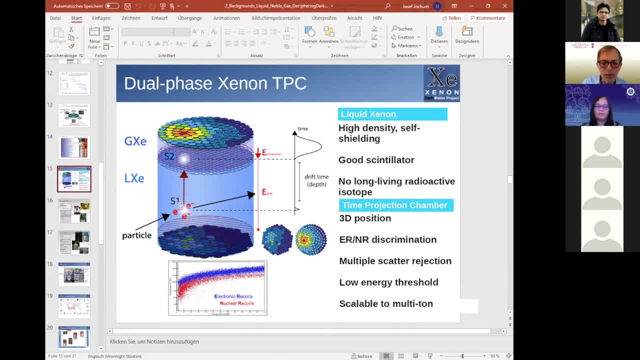 and they or which take longer to, and they or which take longer to recombine and this, this recombine, and this, this recombine, and this, this, this discharges. you have a charge chance- this discharges. you have a charge chance- this discharges. you have a charge chance to drift them away. 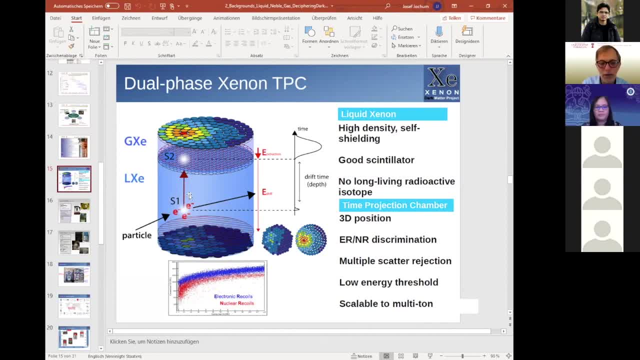 to drift them away, to drift them away from the position, and you drift them then from the position, and you drift them then from the position, and you drift them then through the liquid xenon, through the liquid xenon, through the liquid xenon, and then this, experimentally, is it's: 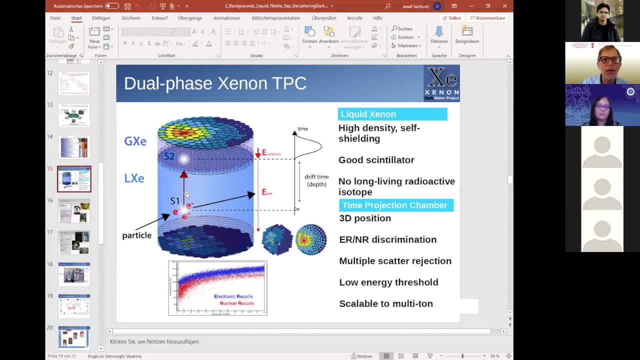 and then this, experimentally, is it's? and then this, experimentally, is it's? it's that the point is along this pass. it's that the point is along this pass. it's that the point is along this pass. when the charge drifts through the liquid. 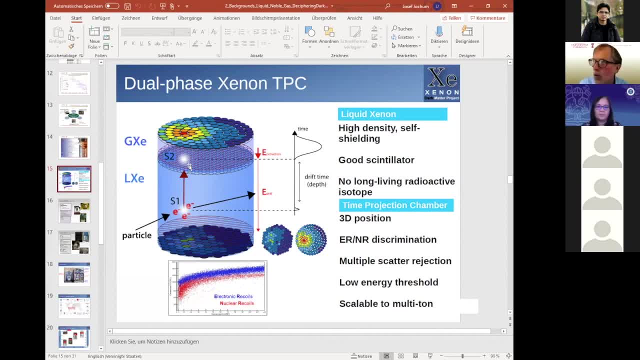 when the charge drifts through the liquid. when the charge drifts through the liquid, xenon these electrons also could xenon. these electrons also could xenon. these electrons also could be bound by molecules or by be bound by molecules, or by be bound by molecules or by impurities in the detector. so the 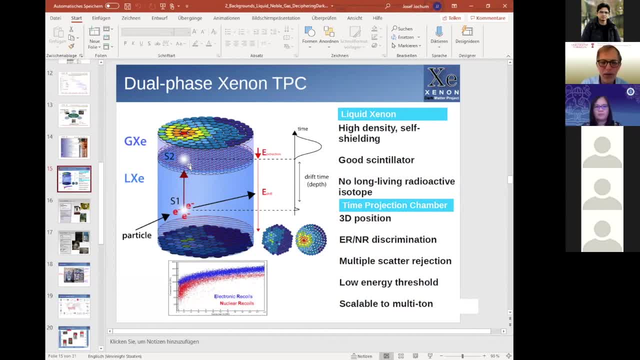 impurities in the detector, so the impurities in the detector. so the detector never is completely pure. detector never is completely pure. detector never is completely pure, but the electrons could be catched for. but the electrons could be catched for. but the electrons could be catched, for example, by remnants of oxygen in the. 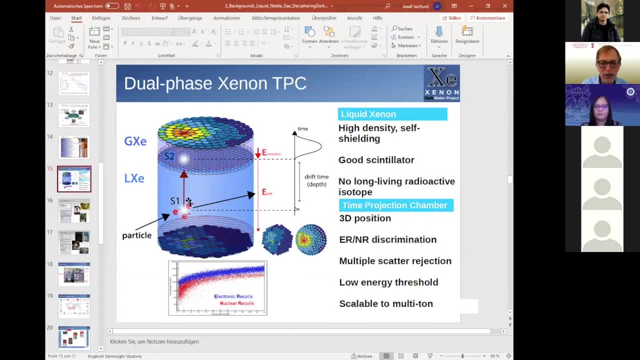 example, by remnants of oxygen in the example, by remnants of oxygen in the liquid xenon: liquid xenon, liquid xenon. so if your xenon is not so, if your xenon is not so, if your xenon is not pure enough, you might lose your charges. 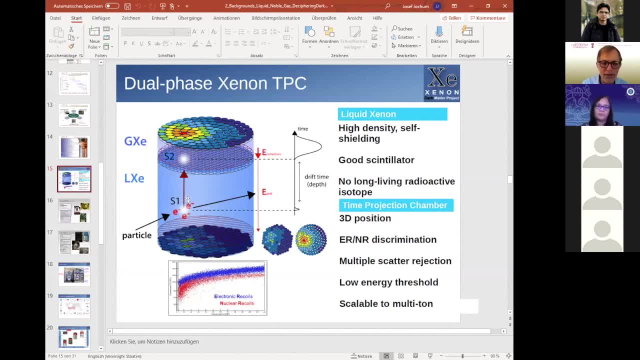 pure enough, you might lose your charges. pure enough, you might lose your charges along the way, along the way, along the way your xenon is pure enough and your field, your xenon is pure enough and your field, your xenon is pure enough and your field is high enough, then you can drift the. 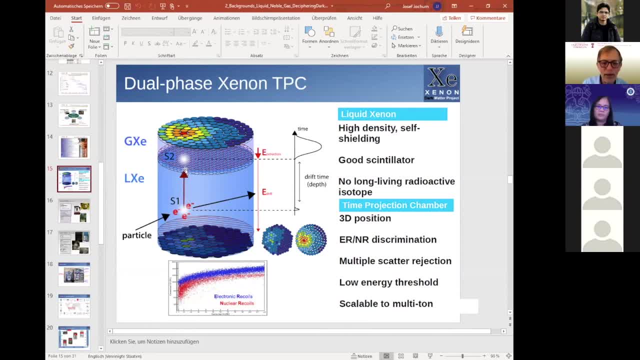 is high enough, then you can drift the is high enough, then you can drift the charges up to the surface, charges up to the surface, charges up to the surface. and of course you could measure the and of course you could measure the and of course you could measure the electrons with electrodes. 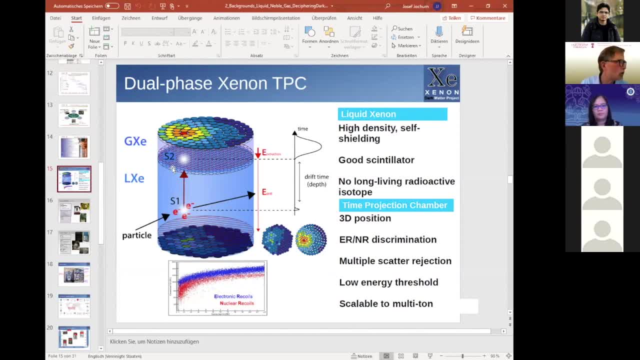 electrons with electrodes, electrons with electrodes. so for the large, so for the large, so for the large. cern experiments, cern experiments, cern experiments. there are also such liquid xenon. there are also such liquid xenon. there are also such liquid xenon. detectors, detectors, detectors, but they measure the charges. 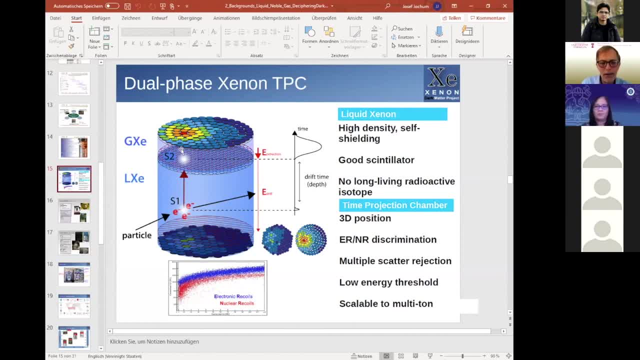 but they measure the charges, but they measure the charges. they measure the charges by electrodes. they measure the charges by electrodes, they measure the charges by electrodes. but but, then, but, but, then, but, but then, these electrodes in this detectors, would these electrodes in this detectors, would these electrodes in this detectors would introduce 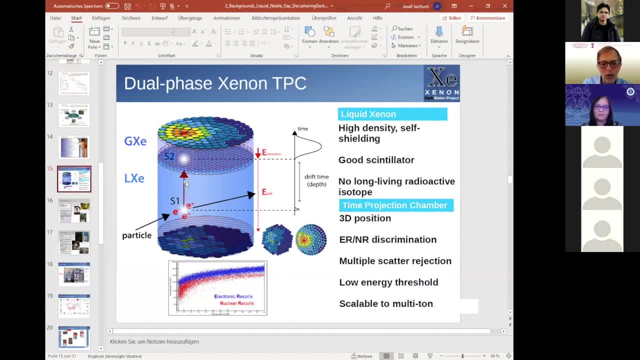 introduce, introduce contaminations. so that's why in xenon contaminations. so that's why in xenon contaminations. so that's why in xenon, one decides to measure without electrodes. one decides to measure without electrodes, one decides to measure without electrodes, and the trick is, you extract the 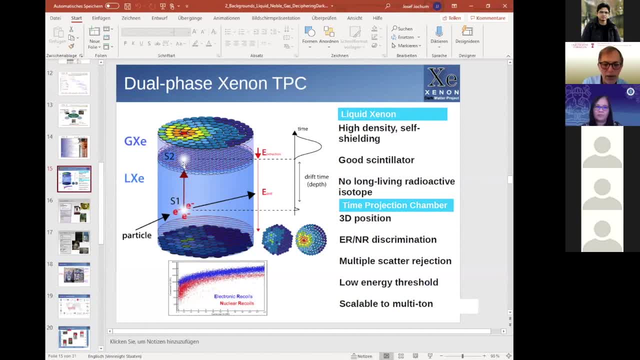 and the trick is you extract the. and the trick is you extract the electrons into the gaseous phase. so up electrons into the gaseous phase. so up electrons into the gaseous phase. so up here is gas, xenon gas, down here is the. 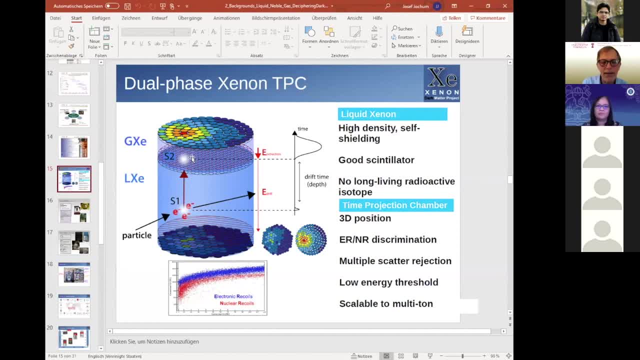 here is gas, xenon gas. down here is the. here is gas- xenon gas. down here is the liquid. you extract them in the gaseous liquid. you extract them in the gaseous liquid. you extract them in the gaseous phase, in the gaseous phase. 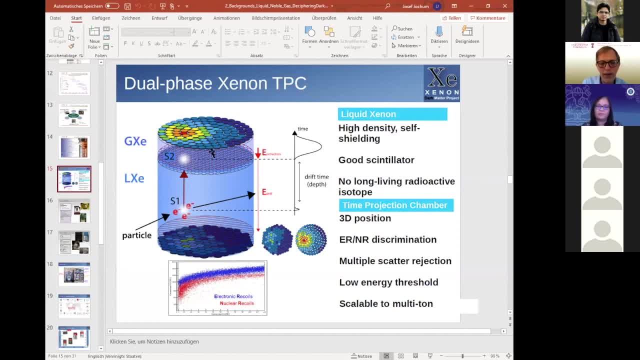 phase, in the gaseous phase, in the gaseous phase, in the gaseous phase, they produce again light. similar like they produce again light. similar like they produce again light. similar like before they ionize the gas: the gas is. before they ionize the gas, the gas is. 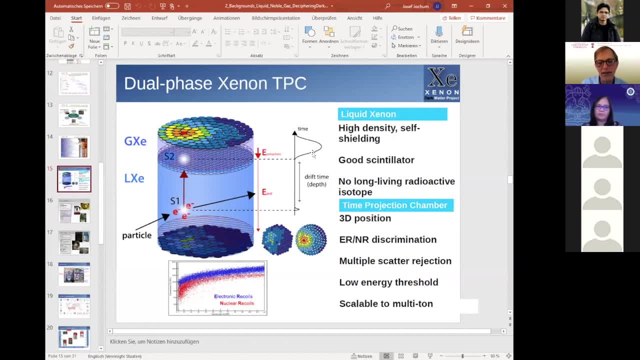 before they ionize the gas. the gas is again, again, again emitting light, and this you see as the emitting light, and this you see as the emitting light, and this you see as the secondary signal, secondary signal, secondary signal. so these are the physics processes. so these are the physics processes. 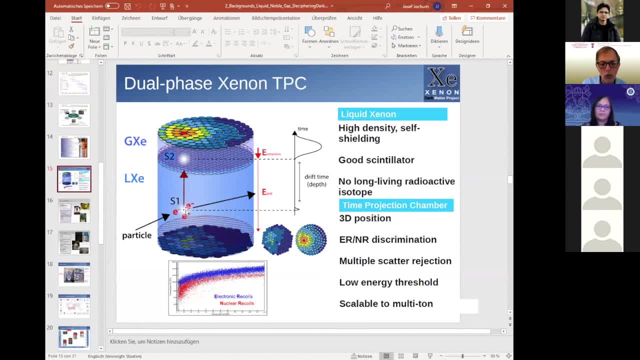 so these are the physics processes happening here and then happening here, and then happening here, and then i i said this was a photon starting i. i said this was a photon starting i. i said this was a photon starting here, here, here, if a vimp comes in, a vimp only gives a. 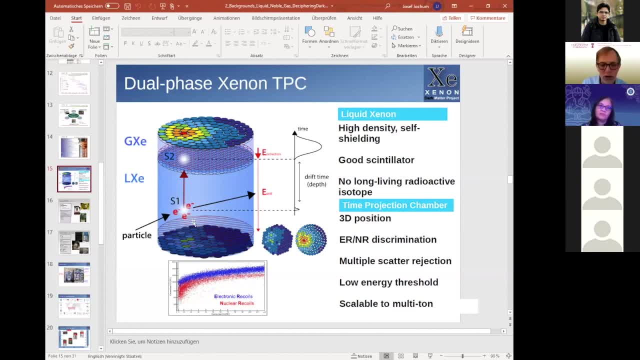 if a vimp comes in a vimp only gives a. if a vimp comes in a vimp only gives a. nuclear recoil to a xenon nucleus, nuclear recoil to a xenon nucleus, nuclear recoil to a xenon nucleus. and this xenon nucleus if it's 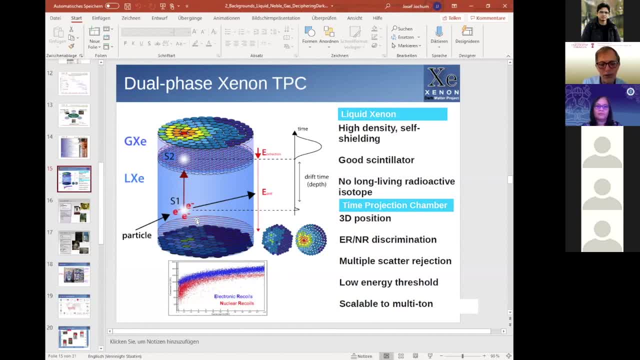 and this xenon nucleus, if it's, and this xenon nucleus, if it's. if it gets, let's say one kev of energy. if it gets, let's say one kev of energy. if it gets, let's say one kev of energy. this kev of energy is enough. 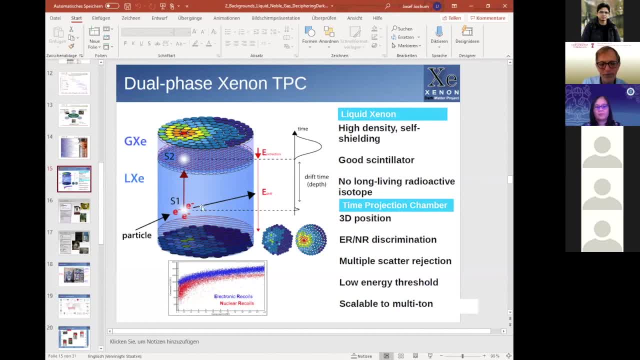 this kev of energy is enough. this kev of energy is enough, so it loses some of its electrons. so it loses some of its electrons, so it loses some of its electrons. and then you have again a positively, and then you have again a positively, and then you have again a positively charged. 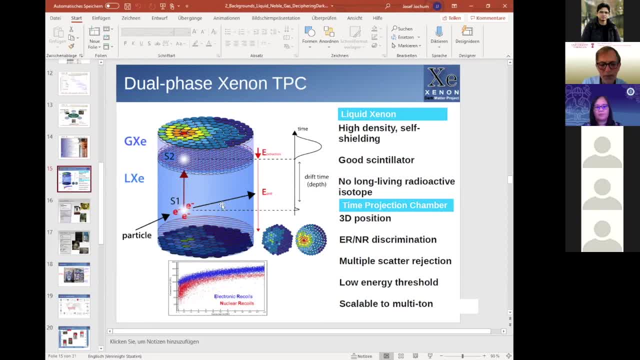 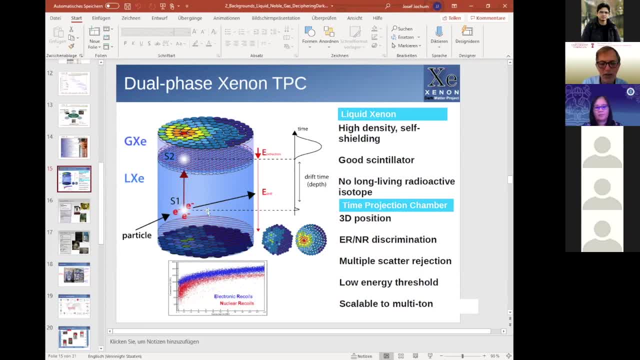 much slower. so because it's a heavy, much slower. so because it's a heavy nucleus with one kv, nucleus with one kv. nucleus with one kv, it's. it's much, much slower than an it's. it's much, much slower than an it's. it's much, much slower than an electron with one kv. 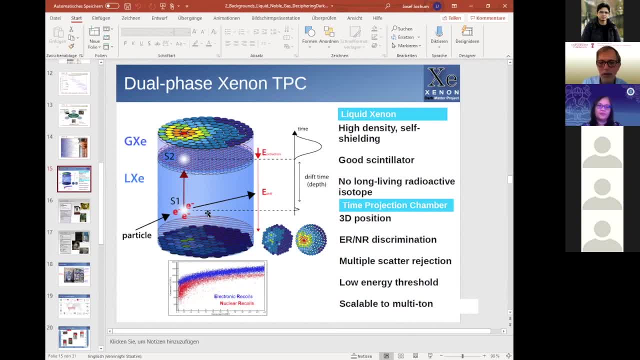 electron with one kv. electron with one kv. that's why this nucleus with one kv, if that's why this nucleus with one kv, if that's why this nucleus with one kv, if you know the beta block formula, for you know the beta block formula, for you know the beta block formula for ionization. 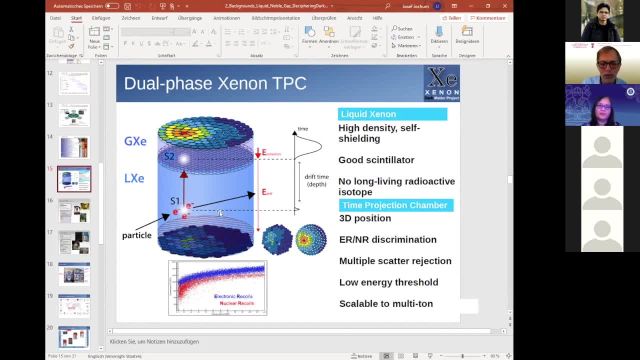 ionization. ionization depends on the speed of the charge, depends on the speed of the charge, depends on the speed of the charge going through your detector. so the speed going through your detector, so the speed going through your detector, so the speed of this liquid, of this liquid. 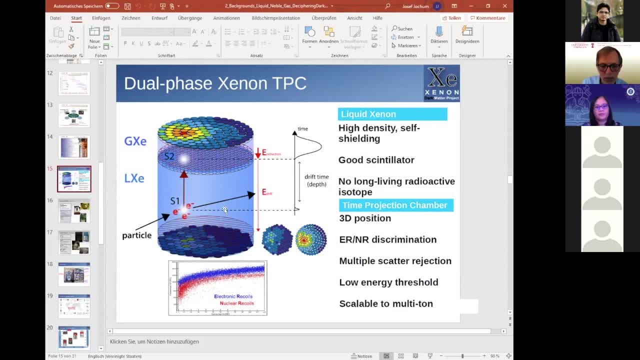 of this liquid. the speed of this nuclear recoil is much, the speed of this nuclear recoil is much. the speed of this nuclear recoil is much, much lower, much lower, much lower than the speed of an electron at the, than the speed of an electron at the, than the speed of an electron at the same energy. 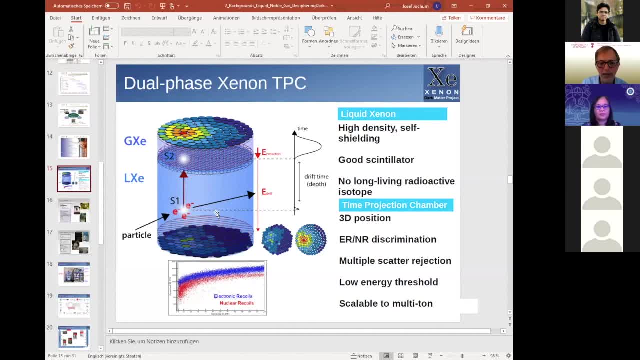 same energy. same energy. that's why this nucleus produces much. that's why this nucleus produces much. that's why this nucleus produces much, much less, much less, much less light than the electron. and that's the light than the electron. and that's the light than the electron. and that's the trick. how you distinguish the two. 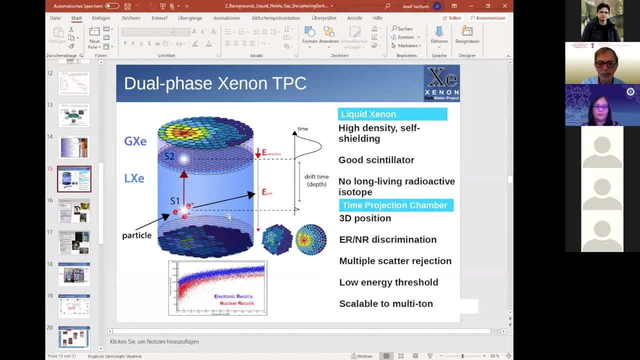 trick, how you distinguish the two trick, how you distinguish the two, so from the light signal versus the, so from the light signal versus the, so from the light signal versus the charge signal, charge signal, charge signal. so this gives you this difference here. so this gives you this difference here. 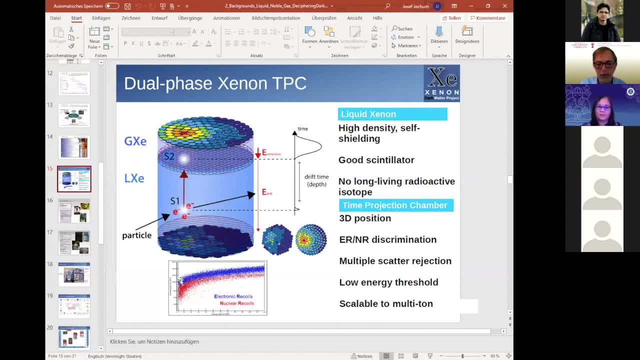 so this gives you this difference here in this plot, where you can distinguish, in this plot, where you can distinguish in this plot, where you can distinguish nuclear records from electronic records, nuclear records from electronic records, nuclear records from electronic records. okay, does this answer your question? okay, does this answer your question. 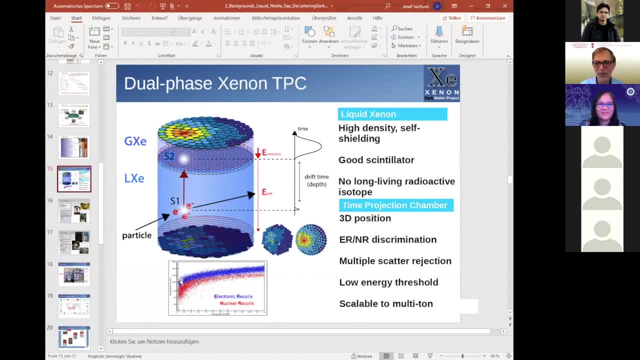 okay, does this answer your question? yes, it's a very good detailed. yes, it's a very good detailed. yes, it's a very good detailed explanation. thank you explanation. thank you explanation. thank you, thank you, okay, you're welcome. thank you, okay, you're welcome. thank you, okay, you're welcome. so you, you still have seven minutes do. 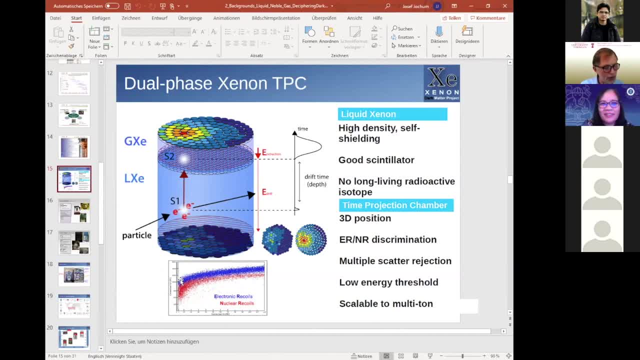 so you, you still have seven minutes. do so you, you still have seven minutes. do you want to continue? uh, you want to continue. uh, you want to continue? uh, i could continue a little bit. maybe i could continue a little bit. maybe i could continue a little bit. maybe that's i could. i could add to the. 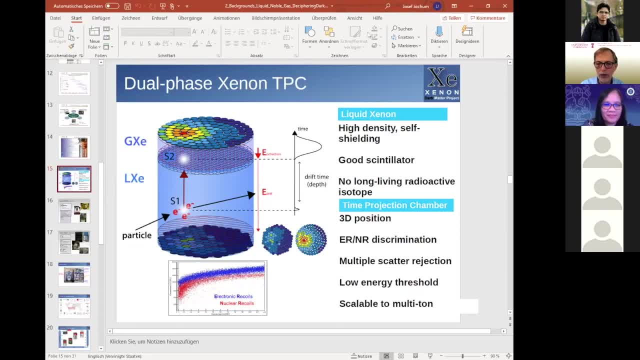 that's i could i could add to the that's i could i could add to the slides. let's see slides. let's see slides. let's see um on on the lomas swims. why lomas um on on the lomas swims, why lomas um on on the lomas swims, why lomas swims are. 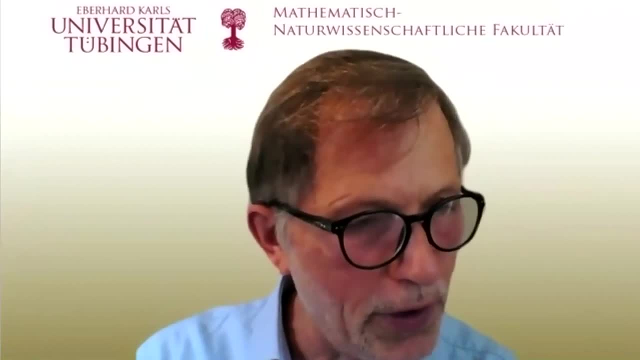 swims are, swims are. so these are basically three slides. and so these are basically three slides. and so these are basically three slides. and then we stop and do a break for half an, then we stop and do a break for half an, then we stop and do a break for half an hour. is that correct? 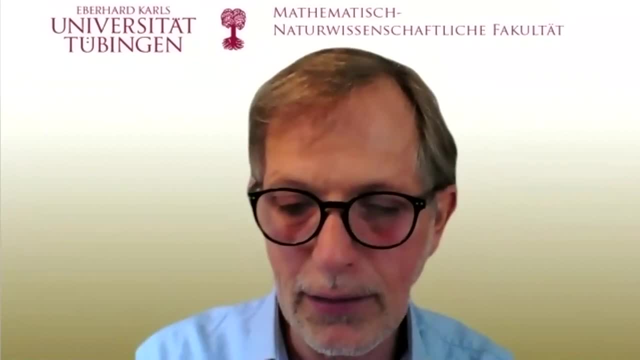 hour. is that correct hour? is that correct? yes, okay, good, so let's see um. yes, okay, good, so let's see um. yes, okay, good, so let's see um. where do i have that file? where do i have that file? where do i have that file? let's see i. 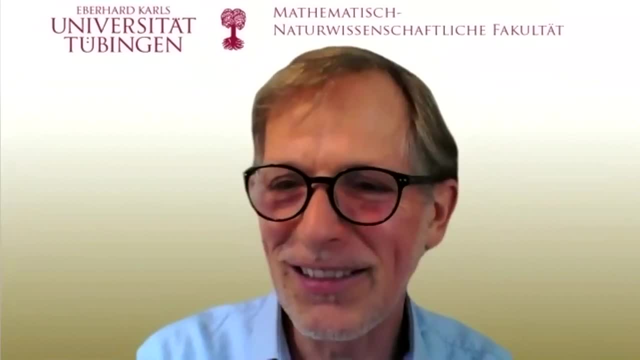 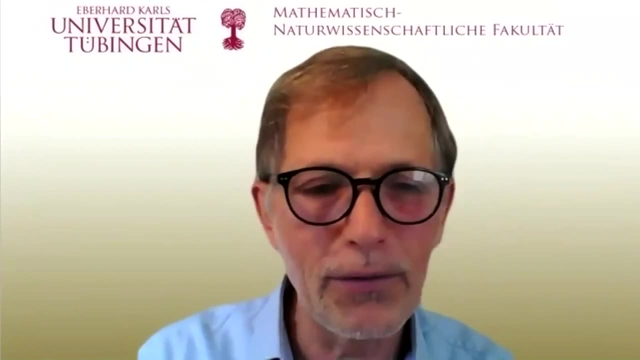 let's see, i let's see, i have to clean up a little bit my desk, have to clean up a little bit my desk, have to clean up a little bit my desk here, here, here. so this is this one okay. so this is this one okay. so this is this one okay. okay, here we are. 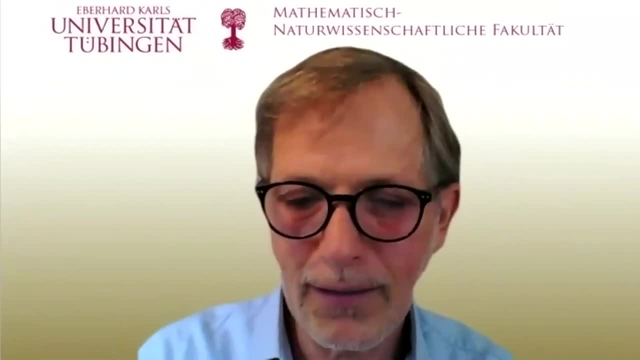 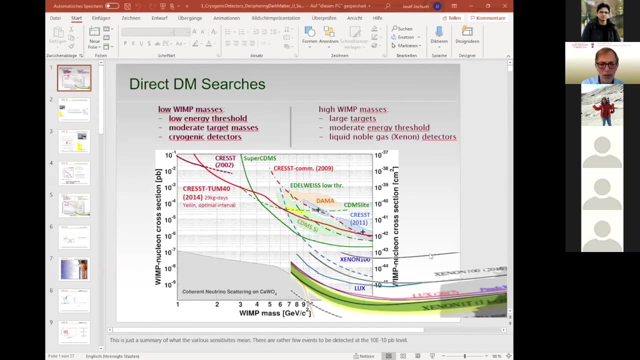 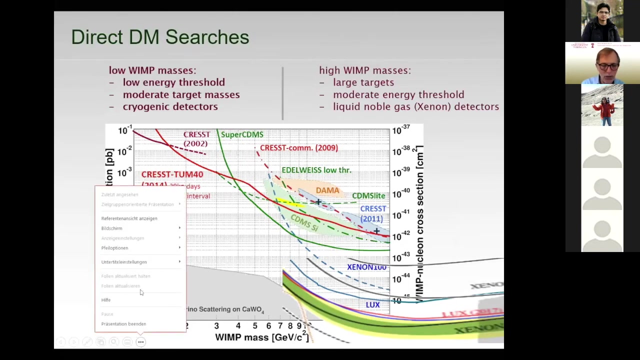 okay, here we are okay. here we are uh, uh, uh, or maybe okay, or maybe okay, or maybe okay, okay, now i go with that. yes, okay, okay, now i go with that. yes, okay, okay, now i go with that, yes, okay. so so here again is this blood which i 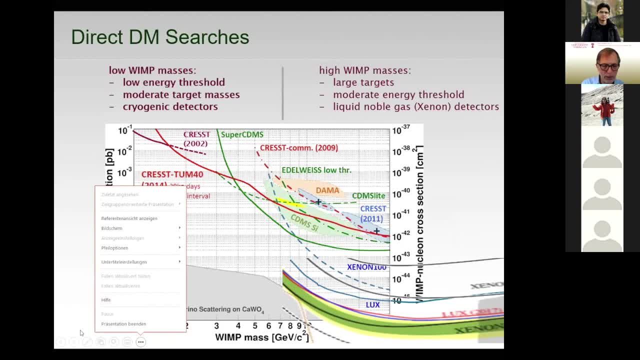 so here again is this blood which i, so, here again is this blood which i showed before. so get the pointer and okay, so this is again okay, so this is again okay. so this is again the plot: uh, vimp mass versus cross. the plot: uh, vimp mass versus cross. 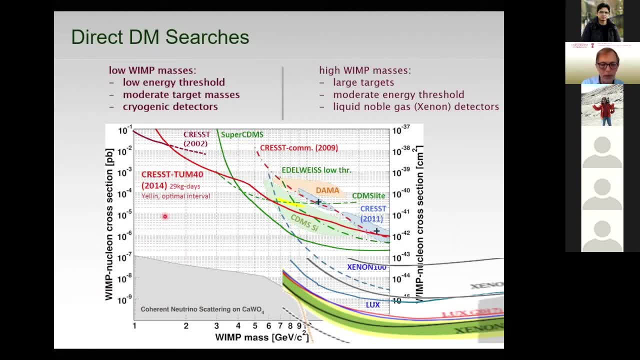 the plot: uh, vimp mass versus cross section on nuclei, section on nuclei, section on nuclei. um in a double logarithmic scale, um in a double logarithmic scale, um in a double logarithmic scale. so here is above a few. gev is the. so here is above a few gev is the. 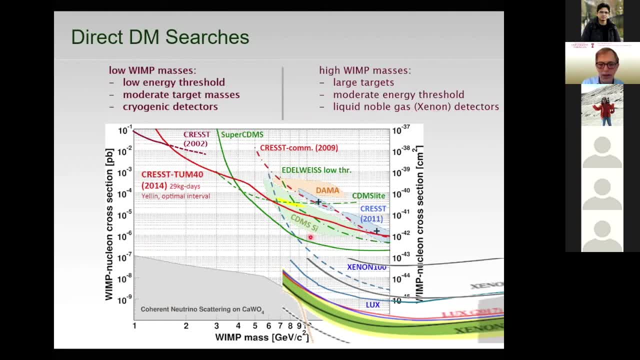 so here is above a few. gev is the region, region, region where the liquid noble gas detectors are, where the liquid noble gas detectors are, where the liquid noble gas detectors are the best ones, the best ones, the best ones, and they are unchallenged there at the 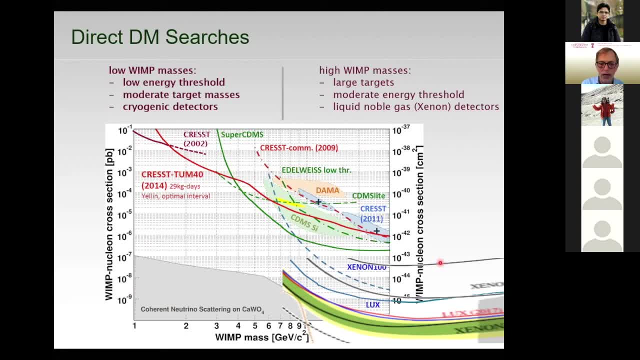 and they are unchallenged there at the and they are unchallenged there at the moment, and i told you about xenon lz moment and i told you about xenon lz moment and i told you about xenon lz and in future, darwin, they will go all. 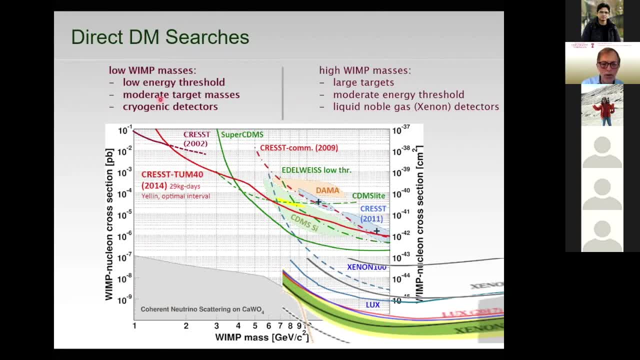 and in future darwin, they will go all, and in future darwin, they will go all. the way down here, the way down here, the way down here, then at the low wind masses. there are then at the low wind masses, there are then at the low wind masses, there are the cryogenic detectors. 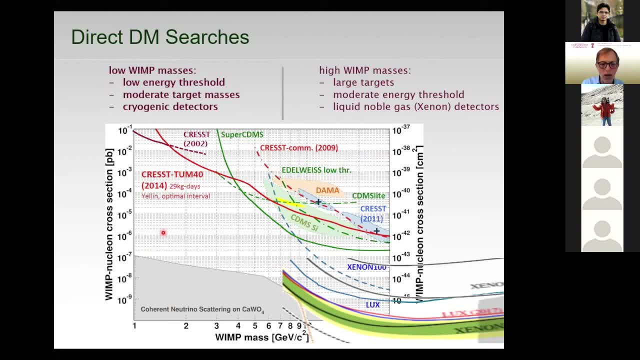 the cryogenic detectors, the cryogenic detectors, and i will just motivate now, in a few, and i will just motivate now in a few, and i will just motivate now in a few minutes, minutes, minutes, why the low wind masses are fashionable, why the low wind masses are fashionable. 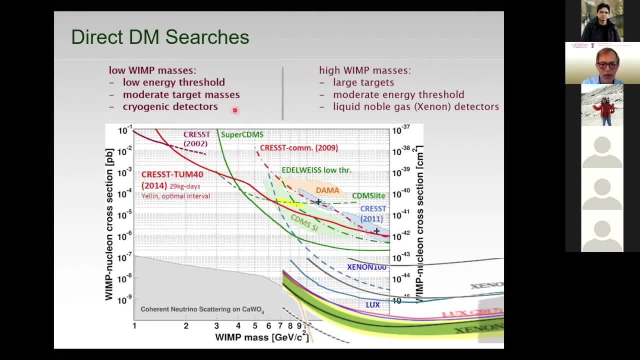 why the low wind masses are fashionable again, again, again. they haven't been 20 years ago, but now. they haven't been 20 years ago, but now they haven't been 20 years ago, but now they are fashionable again. they are fashionable again. they are fashionable again because there are several model. 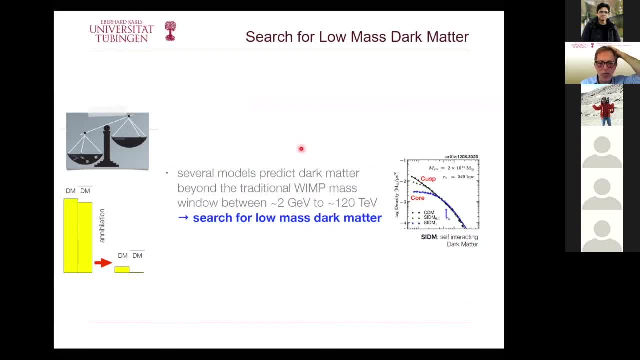 because there are several model, because there are several model models which predict dark matter beyond models which predict dark matter beyond models which predict dark matter beyond the traditional wind mass window, so the the traditional wind mass window, so the the traditional wind mass window, so the traditional, traditional. 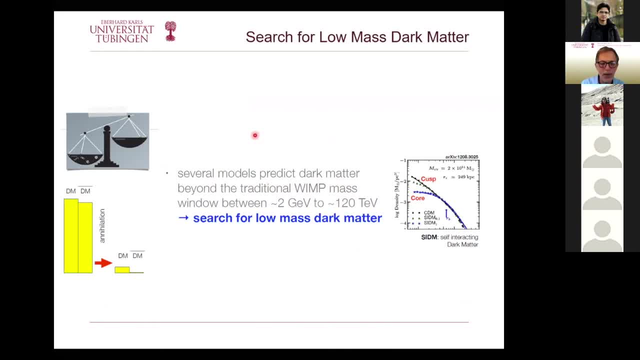 traditional window is gev to 120 tev. window is gev to 120 tev. window is gev to 120 tev. but there are a few ideas and a few. but there are a few ideas and a few, but there are a few ideas and a few. actually also very well motivated. 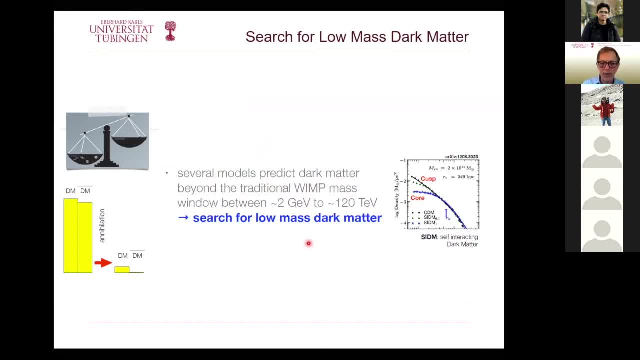 actually also very well motivated, actually also very well motivated uh ideas why dark matter could be very uh ideas why dark matter could be very uh ideas why dark matter could be very light, light, light. and i will just mention two, and i will just mention two, and i will just mention two. one has is the name called asymmetric. 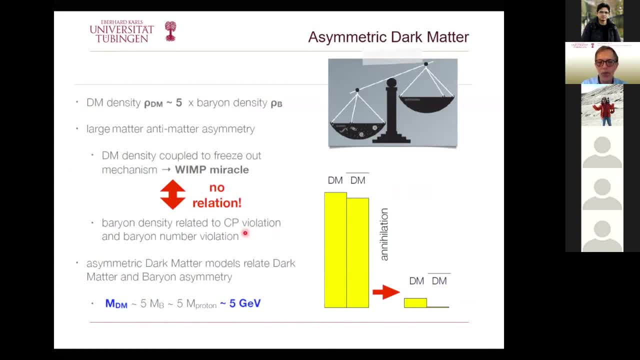 one has, is the name called asymmetric. one has, is the name called asymmetric. dark matter, dark matter, dark matter. so, from the numbers we get from so, from the numbers we get from so, from the numbers we get from cosmology, we know that the dark matter, cosmology, we know that the dark matter 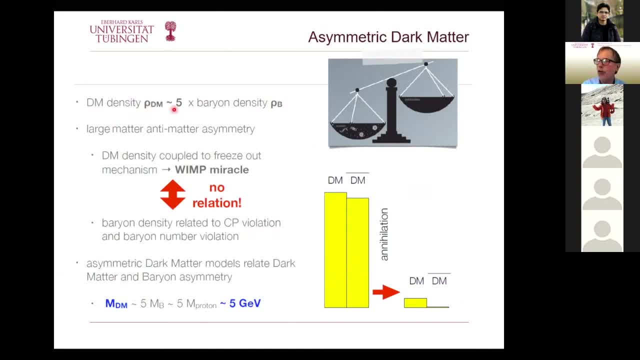 cosmology, we know that the dark matter density, density, density, it's around an omega of 23 or so. it's around an omega of 23 or so it's around an omega of 23 or so, while the baryonic density, so the. while the baryonic density, so the. 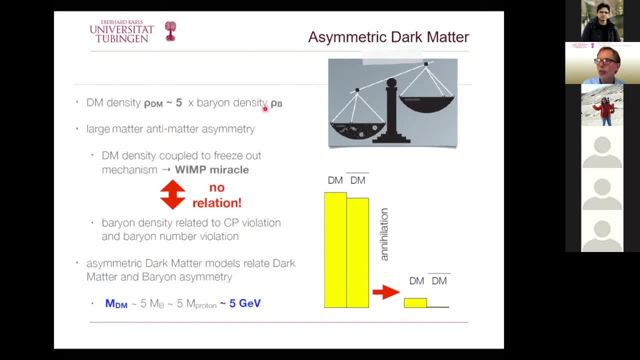 while the baryonic density, so the standard model particle, let's say standard model particle, let's say standard model particle, let's say, is on an omega of 0.04, is on an omega of 0.04, is on an omega of 0.04. so the dark menda density is five times. 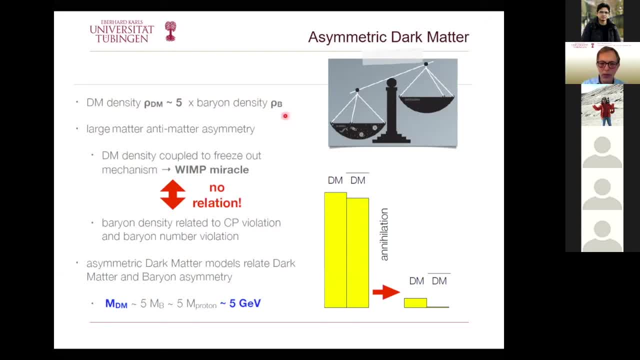 so the dark menda density is five times. so the dark menda density is five times the baryon density, the baryon density, the baryon density. so that's the observation from cosmology. so, so so, and the standard picture for dark matter. 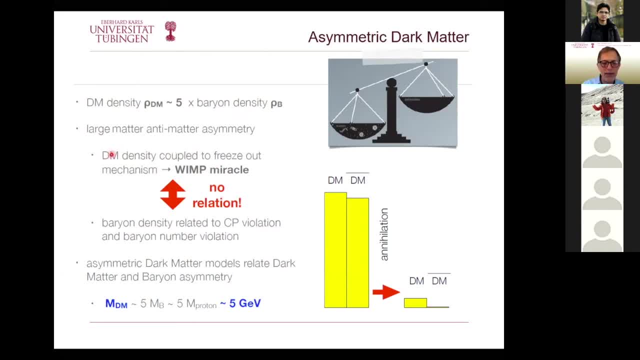 and the standard picture for dark matter. and the standard picture for dark matter is: is is. so which gives us the heavy dark matter, so which gives us the heavy dark matter, so which gives us the heavy dark matter is is, is that the dark matter was an equilibrium. 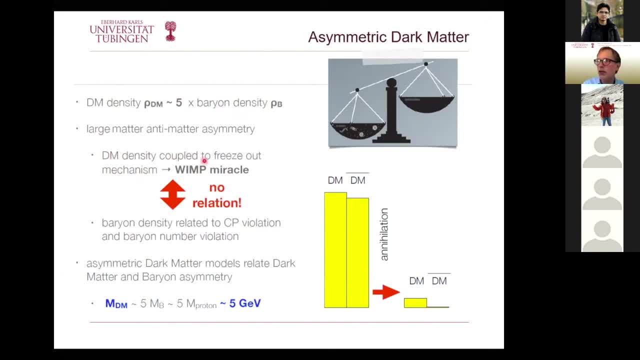 that the dark matter was an equilibrium, that the dark matter was an equilibrium in the early universe, in the early universe, in the early universe. but due to the weak interaction, it froze. but due to the weak interaction, it froze. but due to the weak interaction, it froze out. 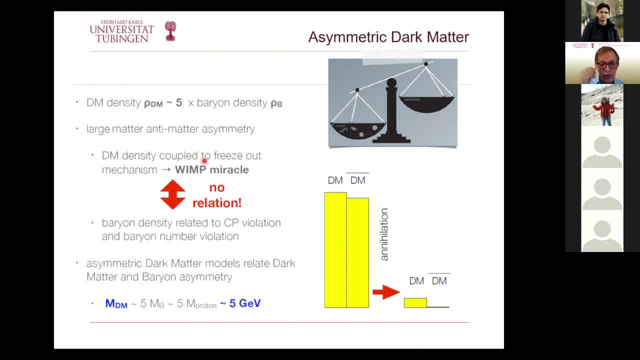 out, and this: this was left over. this was the. and this, this was left over. this was the. and this, this was left over. this was the left over, which produced us the. the dark left over, which produced us the the dark left over which produced us the the dark matter. 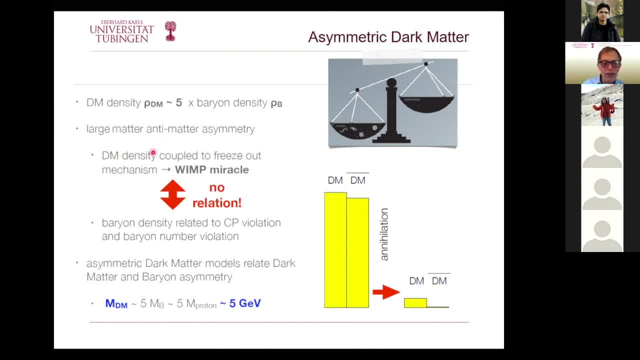 matter matter. and the funny thing is this freeze out. and the funny thing is this freeze out. and the funny thing is this freeze out mechanism needs the weak interaction mechanism, needs the weak interaction mechanism, needs the weak interaction scale, and that's what's called the vimp. 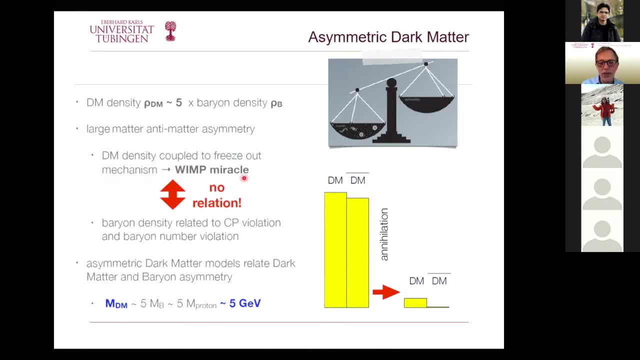 scale, and that's what's called the vimp scale, and that's what's called the vimp miracle. why weak interaction is seen as miracle. why weak interaction is seen as miracle. why weak interaction is seen as being a connection to dark matter, being a connection to dark matter. 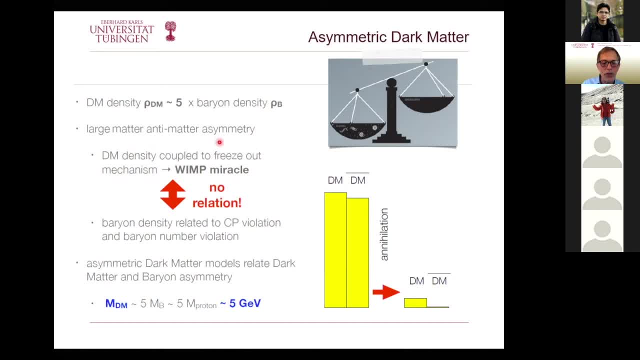 being a connection to dark matter. okay, this is how dark matter is in the. okay, this is how dark matter is in the. okay, this is how dark matter is in the standard picture being produced into the standard picture being produced into the standard picture being produced into the universe. 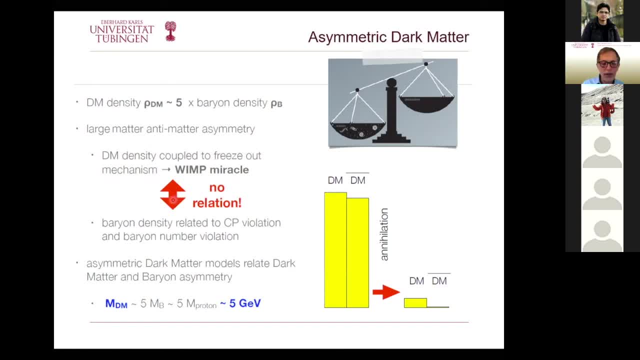 universe, universe. uh the baryons, uh the baryons, uh the baryons, the baryon density, the baryon density, the baryon density is considered as being a left over, is considered as being a left over, is considered as being a left over from an asymmetry between meta and 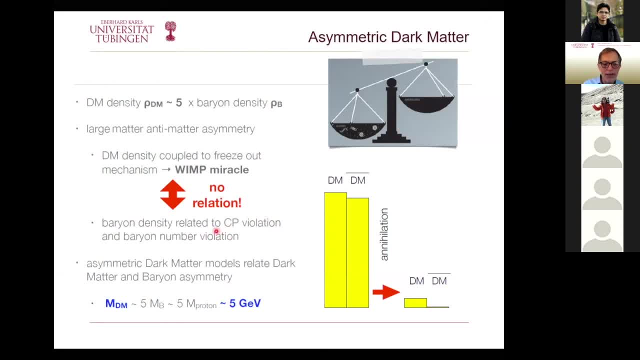 from an asymmetry between meta and from an asymmetry between meta and antimatter: antimatter, antimatter. so the baryon density is is related to cp. so the baryon density is is related to cp. so the baryon density is is related to cp violation. so the idea is in the early. 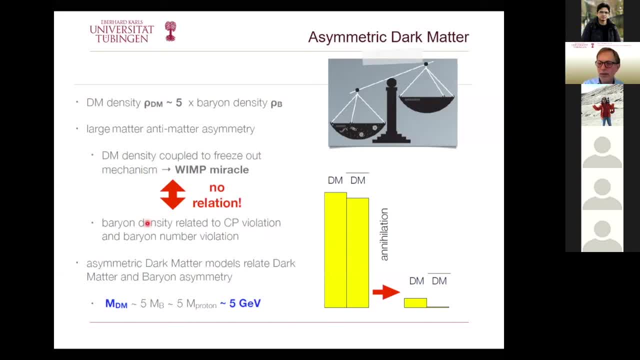 violation. so the idea is in the early violation, so the idea is in the early universe. universe universe we have meta and antimatter symmetric. we have meta and antimatter symmetric. we have meta and antimatter symmetric. actually the standard model, actually the standard model, actually the standard model, the standard model of particle physics. 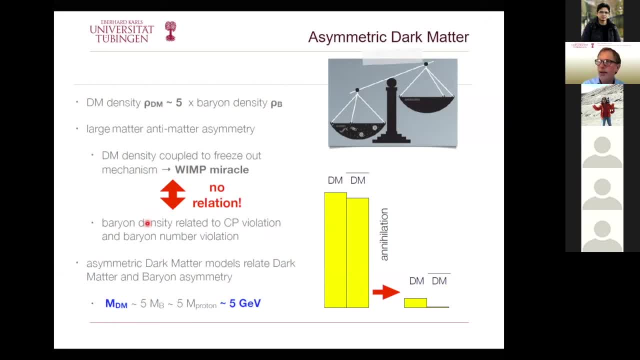 the standard model of particle physics, the standard model of particle physics, expect the two be symmetric, expect the two be symmetric, expect the two be symmetric. and then and then, and then, when the universe cools down this meta, when the universe cools down this meta, when the universe cools down this meta and antimatter would completely 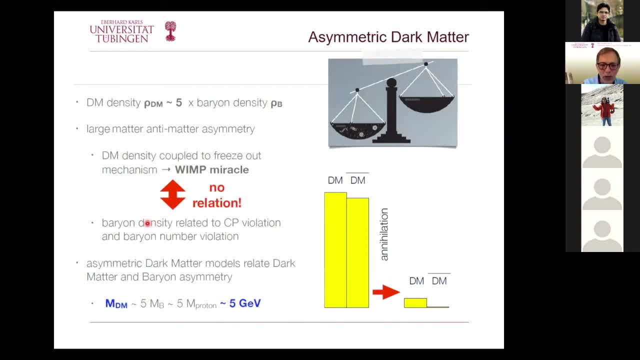 and antimatter would completely, and antimatter would completely annihilate and we would not be left with annihilate and we would not be left with annihilate and we would not be left with any matter at all, any matter at all, any matter at all. but there must have been a tiny asymmetry. 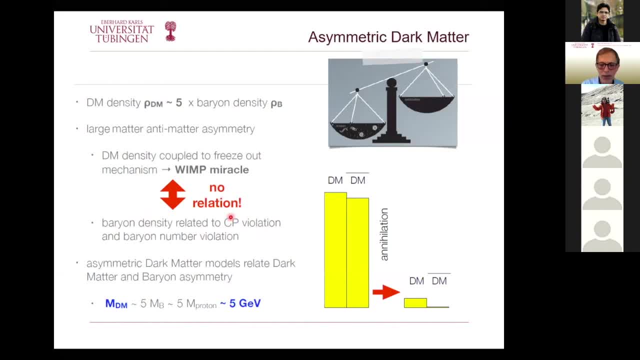 but there must have been a tiny asymmetry, but there must have been a tiny asymmetry between meta and antimatter, so between meta and antimatter. so all the met, most of the matter and antimatter annihilated, but a little bit of matter, didn't find antimatter to annihilate, had no partners, and this asymmetry is on a level of 10 to the minus 9. 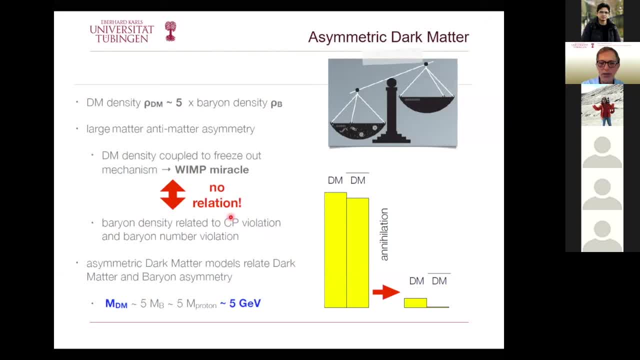 and this is also being measured in cosmology, because the ratio between the number of baryons we have and the number of photons we have is 10 to the 9.. so we see there was a huge annihilation at the beginning in the universe. all the matter and antimatter annihilated. 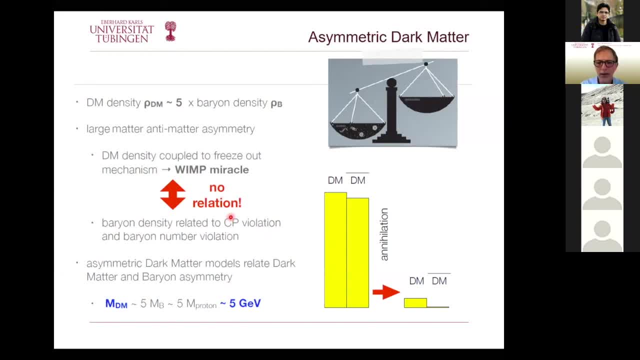 one billion protons annihilated with anti-protons, but one out of one billion was left without partner. so this is a measurement. we see that, and the funny thing is that, between the production of matter in the universe and the production of dark matter in the universe. 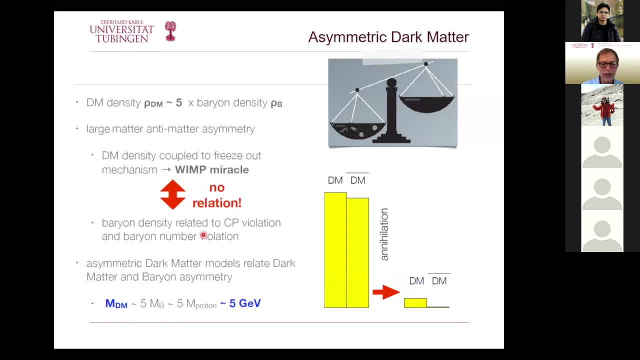 in this picture there is no relation and that's strange. so that's the weakness of the standard limp dark matter paradigm. so here in asymmetric dark matter, one says you, one started completely differently. one says, okay, there must be a cp violation to produce this asymmetry between matter and antimatter. 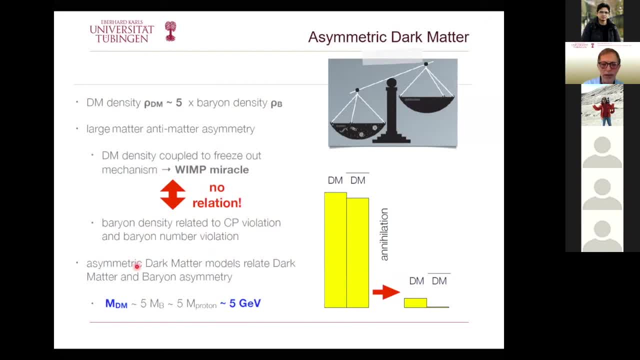 and the assumption now is that dark matter and normal dark matter share the same asymmetry. so there was an early pro pro process producing asymmetry between meta and antimatter and it produced the same in the dark matter as in the normal meta sector. so that's also a very natural. 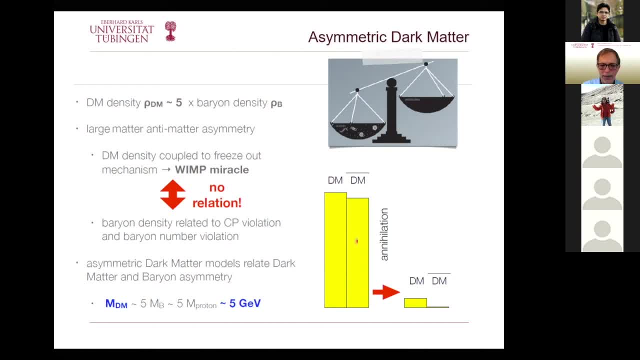 assumption, and then all the dark matter and the antidark Score-based analysis matter are annihilated and only this asymmetry, dark matter, was left over. the same process, like in the matter production, and this tells you immediately that the mass of the dark matter, so this tells you that the number of dark meta particles is the same, like the. 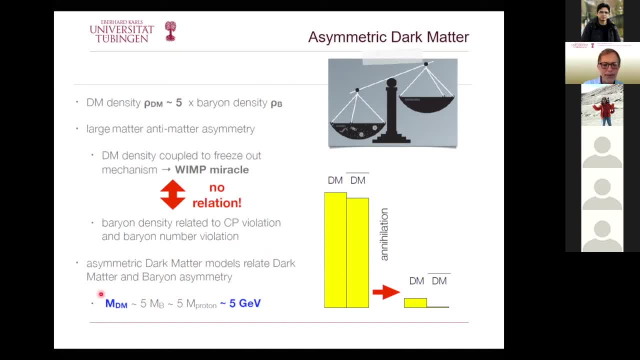 number of normal meta particles. and this tells you that the dark matter particle must have 5 times the mass of the proton, because the dark matter density is 5 times the density of the dark matter retailers density of protons. So this gives you immediately a dark metamath of 5 GeV. So this is weak. 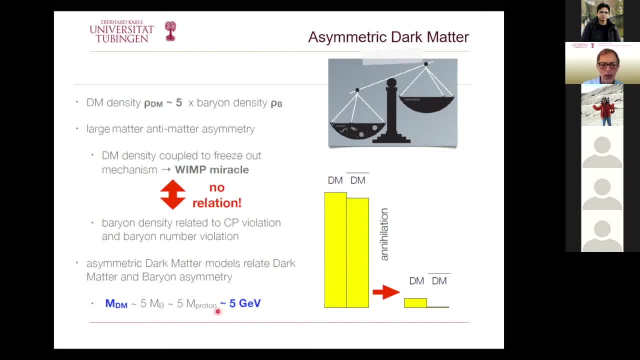 This is a small mass, So this is a low mass, And you can tweak this 5 GeV down to below 1 GeV, of course, if you play a little bit around with the CP valuation. Another thing has to do with the problem of n-body simulations of the profile of galaxies. 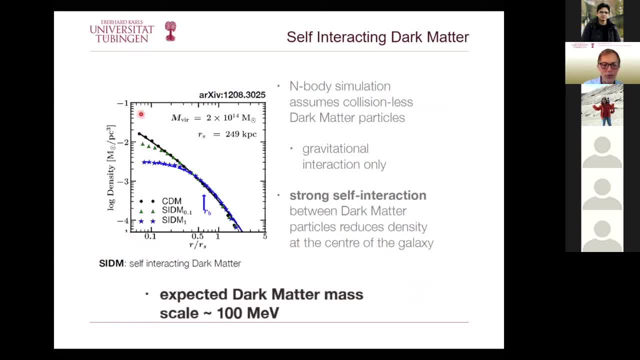 So this is the radius of a galaxy and this is the density profile, And n-body simulations of structure formations tell you something like this: a very high mass density in the center. The measurements show you flatter curves in the center, So we have flatter. 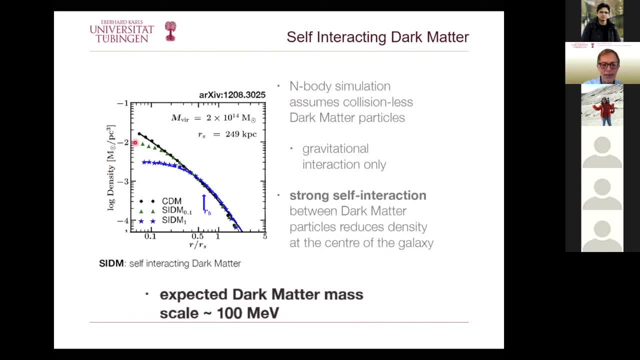 dark matter profiles in the center of galaxies And this is an open issue in astrophysics. It could be a property of the dark matter. if you give dark matter some self-interaction, that dark matter can interact with itself. So the dark matter particles have some interactions. 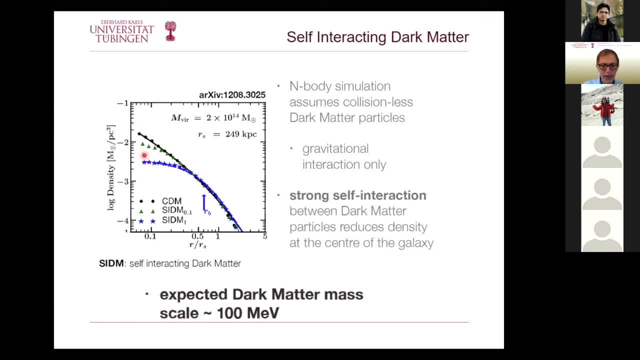 among them. Then you can flatten this slope here. And from the calculations, then from the particle models, which I cannot go into detail here, this self-interacting dark matter also brings you in the dark matter mass range of only 100 MeV. So this is a tenth of GeV. 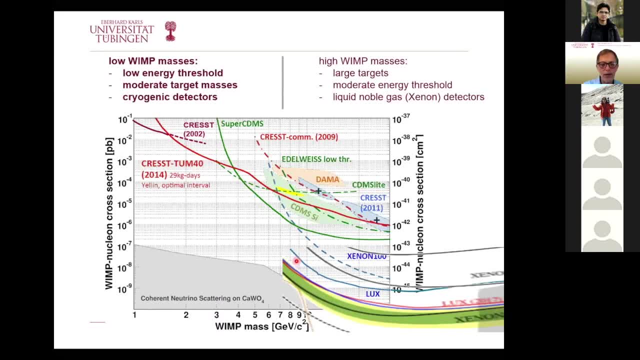 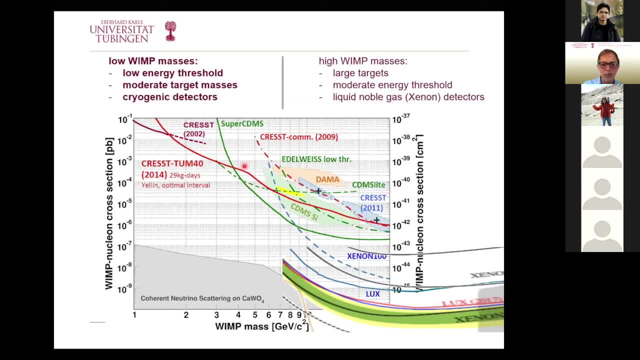 motivated, as, for example, by this asymmetric dark matter things And the liquid xenon detectors have a hard time to get there because the energy threshold is not low enough. As I told you at the beginning, as lower the the mass, the lower are the energies of the recoil. So in this exclusion plots if this 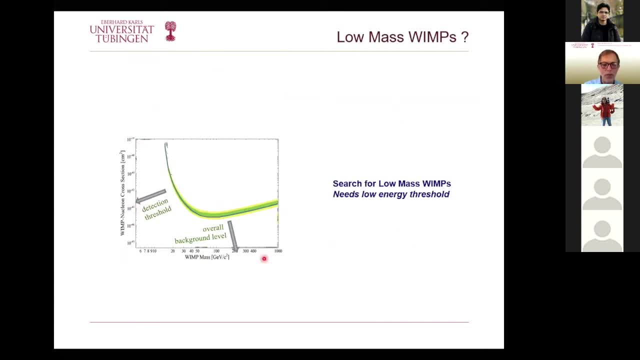 is your exclusion plot. this is cross-section against WIMP mass. going this direction with your exclusion plot means you need a lower detection threshold. While going this direction needs you need to reduce the overall background level. So of course you need both. You need. 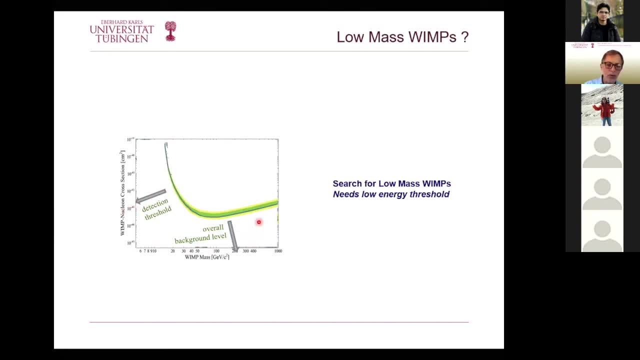 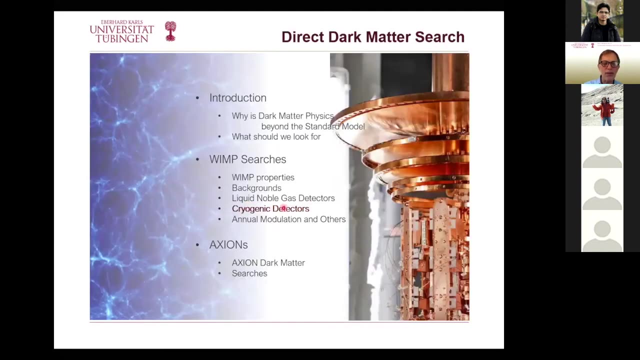 also low background here. but the limit while these curves bend up here is due to the tech nical issue that all the detectors have energy threshold And only if you lower this threshold you can go to the low WIMP masses And this will bring me to cryogenic detectors after. 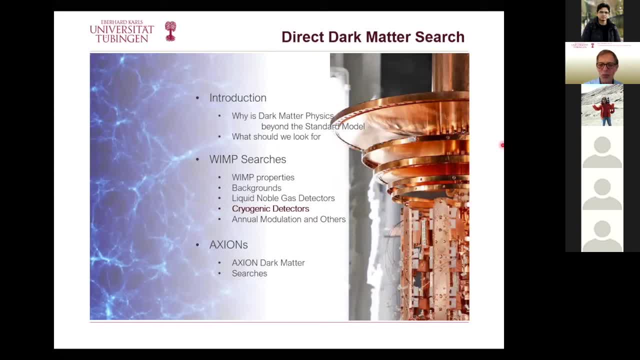 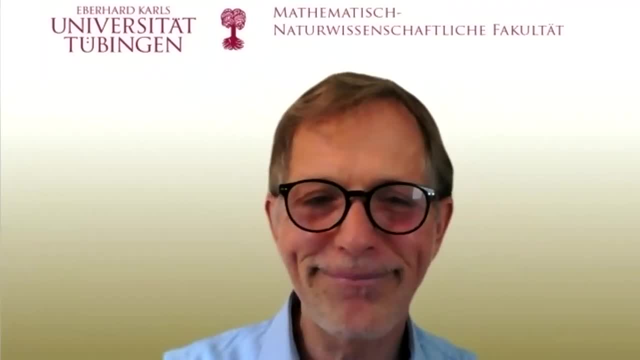 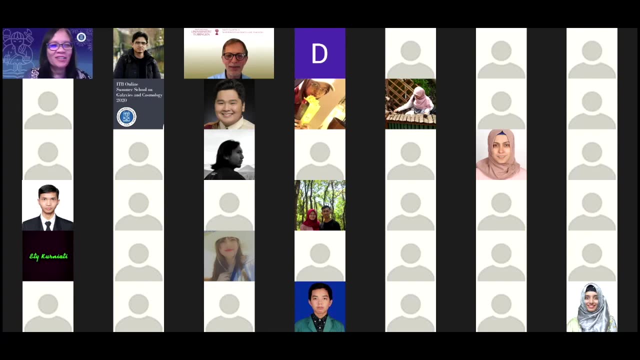 the break. Okay, And I would stop here, Hestie now. Okay, Thank you very much, Youssef. We will have a break now, but before that it's traditional to have group picture, So Smile. 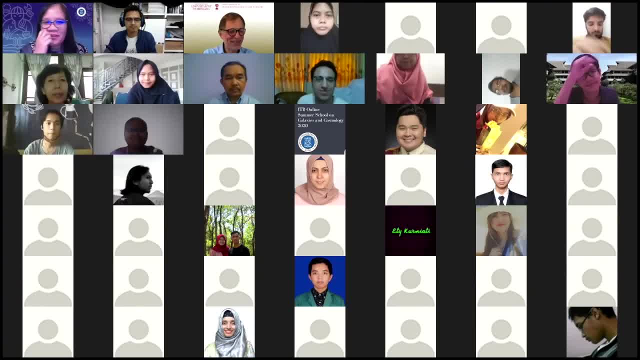 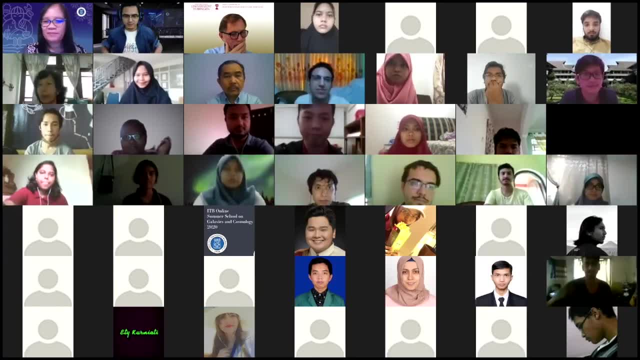 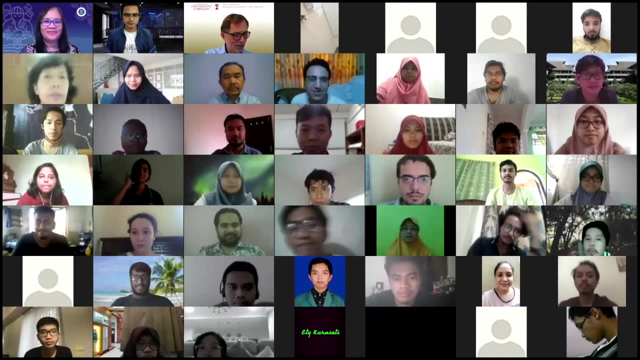 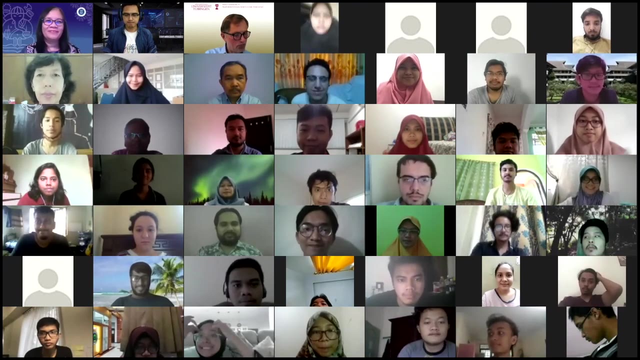 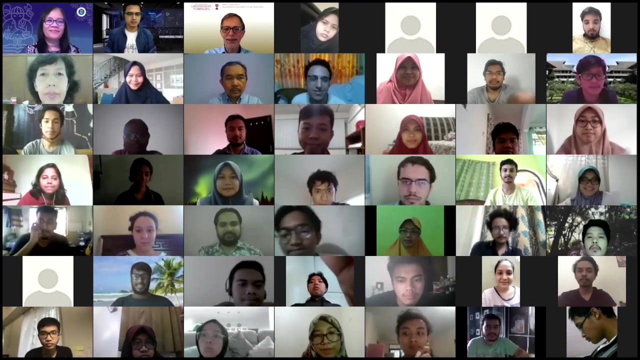 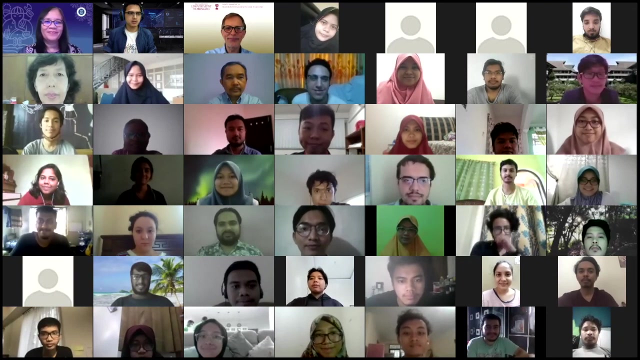 Anton, can you help help us to take? Yeah, Okay, I will take picture. So please open your videos on: Okay Okay, Okay, Okay, I will start to take a picture for slide one: Okay, 1,, 2, 3.. Second slide: Okay, Wait a minute.